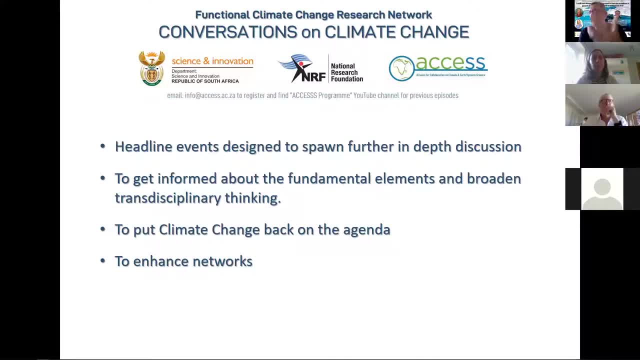 we've covered a fair range and we'll be getting into further depth in some of these topics a bit later in the year. The goal is really to get informed about the fundamental elements and broaden transdisciplinary thinking. A lot of big events happening. We read them in the news often at the moment. 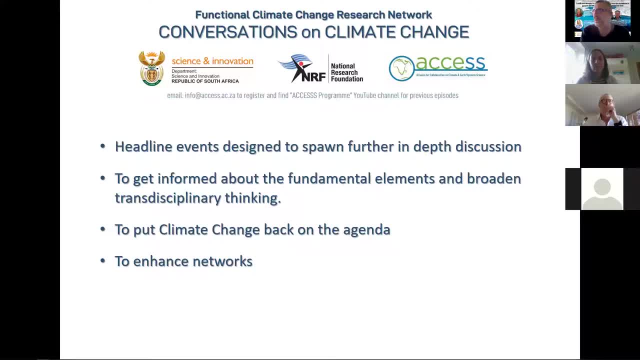 overwhelmed by COVID, And so we really wanted to put climate change back on the agenda and to consider various elements and aspects of climate change, And so that's really what we're doing here, And then also so we can cross disciplines and really enhance the networks. 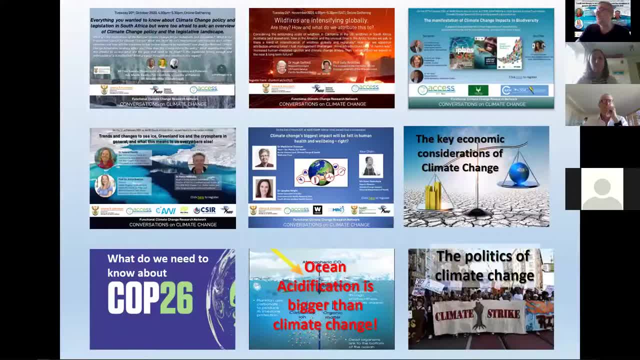 that we have. So, today, these are the topics that we're going to be talking about. We're going to be talking about a number of topics, So we've done one on climate law, one on wildfire, We did one on the biodiversity reports of last year. This week we are dealing with a cryosphere, And I 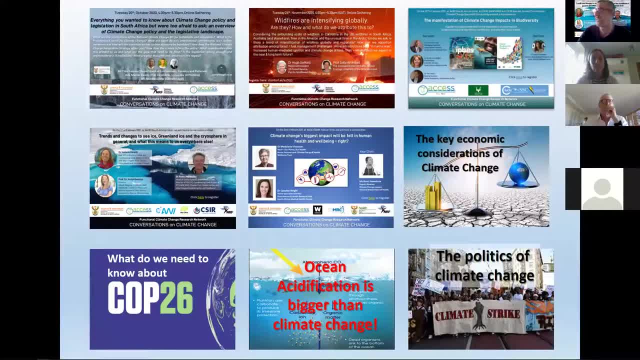 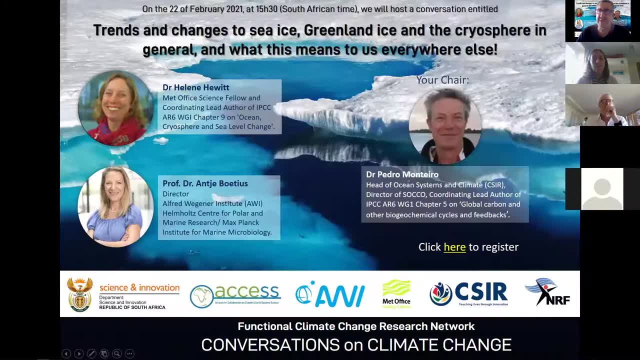 think it's next week, we have an event on climate and health, And then we have a couple of other topics we're going to consider. So this week it's really a great pleasure for me to welcome our very prestigious group of contributors. Pedro is a. 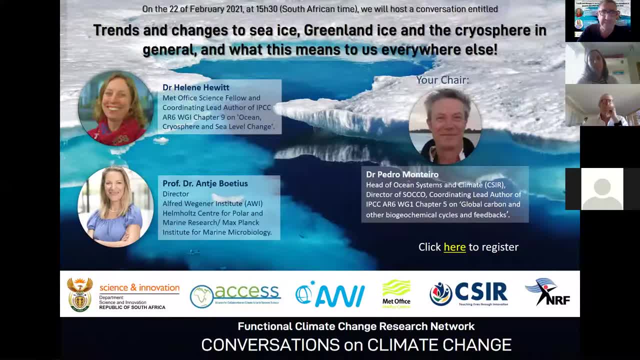 colleague of mine. He works at the CSR. He is an oceanographer at the CSR, holds the position of chief oceanographer at the CSR and runs a research program there, as well as a network called SOCO, which is the Southern Oceans Carbon and Climate Observatory and also is the coordinating lead. 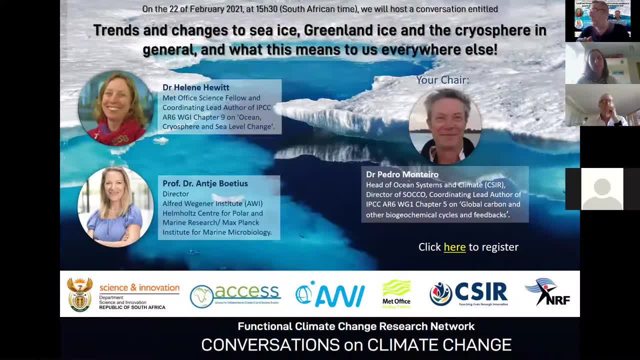 author of IPCC, AR6, Working Group 1, Chapter 5 on global climate change, And he's also a and other biogeochemical cycles and feedbacks, And Helene- who, by the way, is not Helen Chapman, to which I apologize profusely again. I got confused between people I'm dealing with. 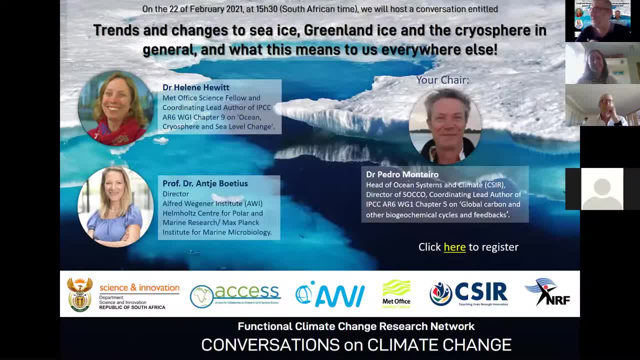 Helene is Helene Hewitt, And Pedro will introduce her, And then we have Dr Ancha Boetius, who will join us a bit later. So that's really all I'm going to say, And now I'm going to hand. 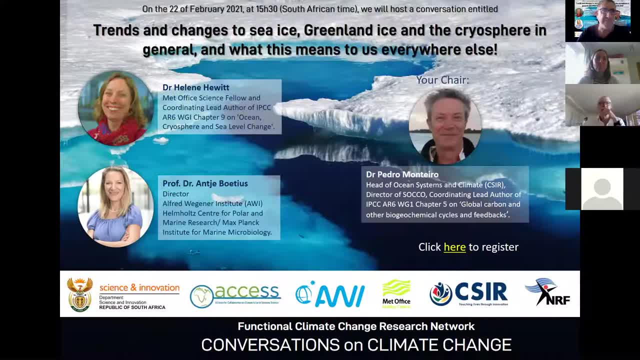 the floor to Pedro, who will take us through this event. So if you have any comments or chats that you want to make, please use the chat box for that purpose. Please keep yourself on mute all the time And we can have some time for discussion. 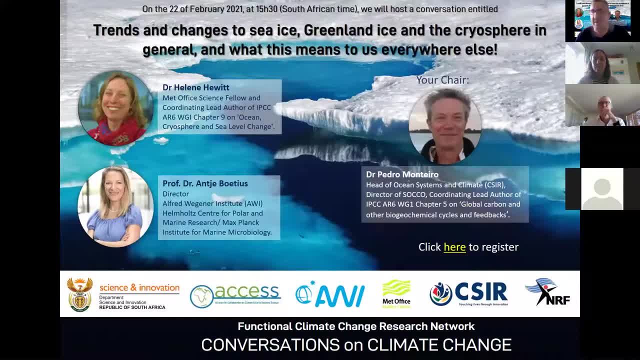 after Helene has given us her input. So, Pedro, over to you, Thanks. Thanks very much, Neville, And thanks very much for inviting me. So first of all, let me do a quick sound check. Can you hear me? Okay, Excellent, Welcome everyone to this really important discussion dialogue around the 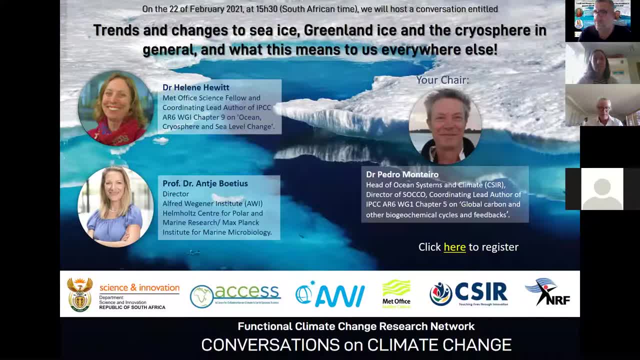 topic which is a really important topic in a global sense, but it actually has quite a low profile in the South African and I say perhaps beyond that landscape of climate discussion topics. So the cryosphere, just briefly. so what is it? 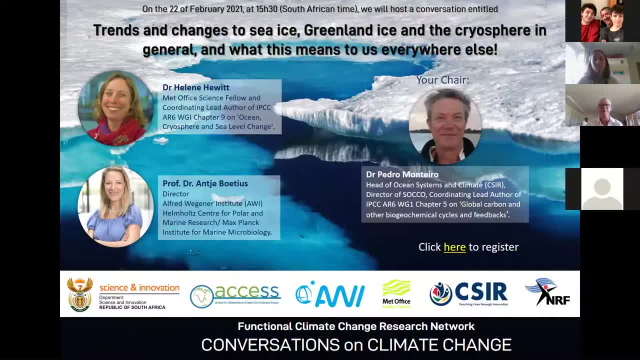 So, essentially, at its simplest, it's the frozen part of the hydrosphere or the water part of the planet, And it includes the sort of ice sheets, glaciers, ice shelves, sea ice In the southern hemisphere. interestingly, even though it holds from a water volume perspective, 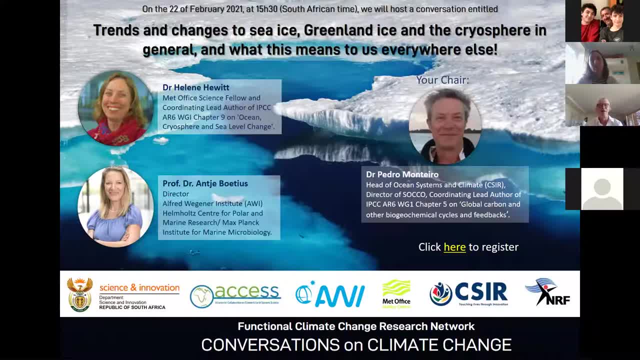 the largest part of the cryosphere in Antarctica it actually has. it's not a very well, sufficiently well- explored topic as much as it is in the northern hemisphere, And at one level it's an easy concept to and it's relatively easy to understand that. It's just that we lack. 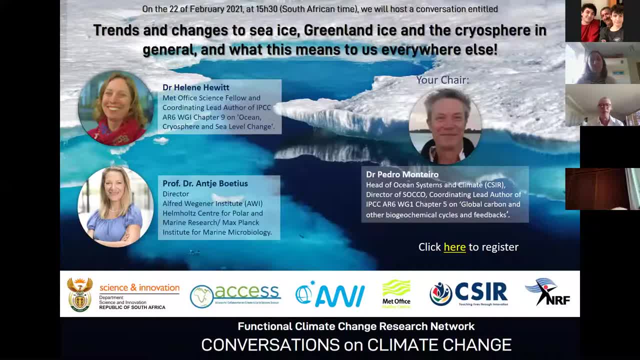 the land mass in the mid to high latitudes. So, for example, Antarctica is separated from Cape Town by 4,000 kilometers of ocean And, to give you another perspective on that, Cape Town and Sydney are at about the latitude of Morocco in the northern hemisphere. 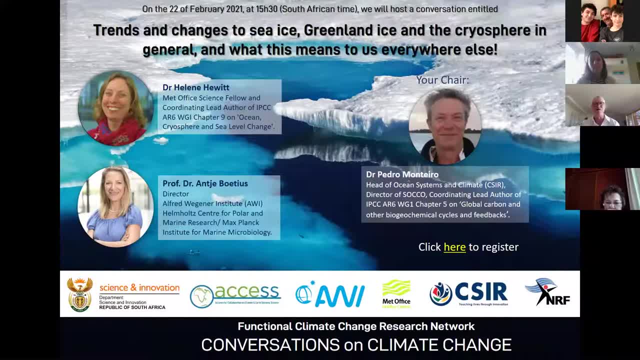 So that kind of gives you the sense of the asymmetry of the relative and experience of the cryosphere, which is a much stronger idea in the northern hemisphere than it is in the southern hemisphere. So the cryosphere is, I mean, one of the reasons why. 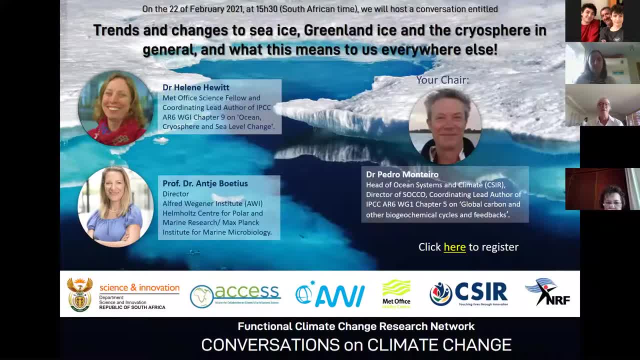 it's really very wide. it's a major topic of discussion And our two guests today- I'll introduce them in a minute- are really evidence of how much effort is going into understanding the cryosphere. The cryosphere has many dimensions And it plays. it has an impact on the atmosphere. 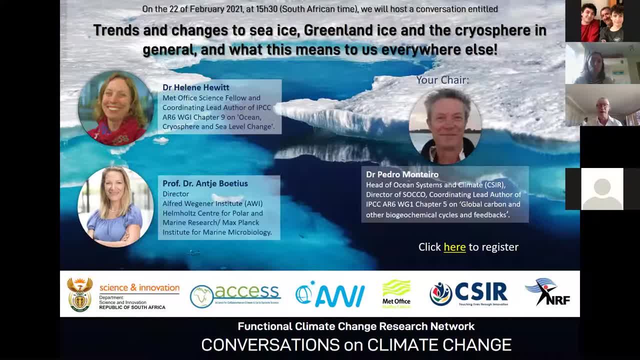 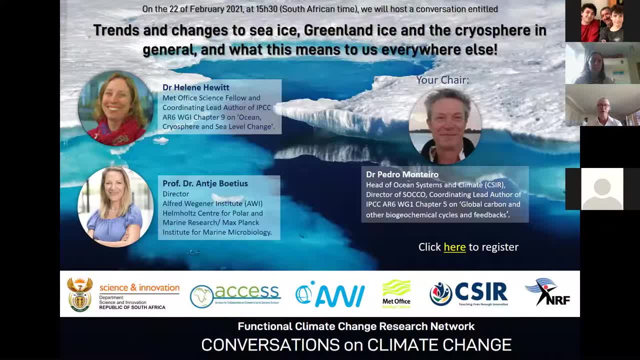 level, we don't really understand all the connections that would allow us to predict how it will evolve under global warming, And so that's kind of really the major effort is kind of understanding cryosphere in the context of the planet and its ecosystems. 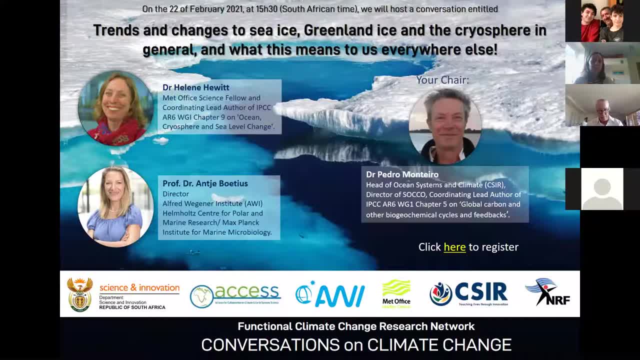 So the kind of questions that one might sort of be thinking about are sort of about hemispheric contrasts, which I've already referred to. How quickly are they changing as a result of global warming, And what are the long-term- in the sort of decades to centuries- implications? 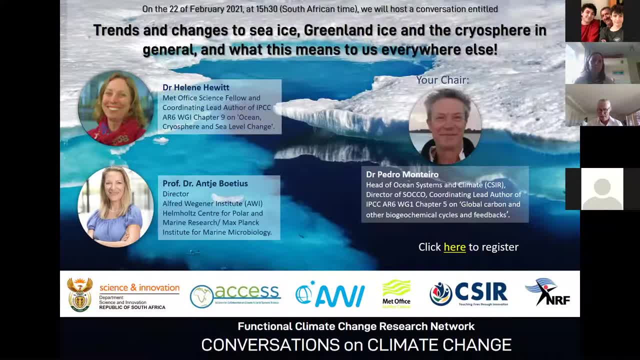 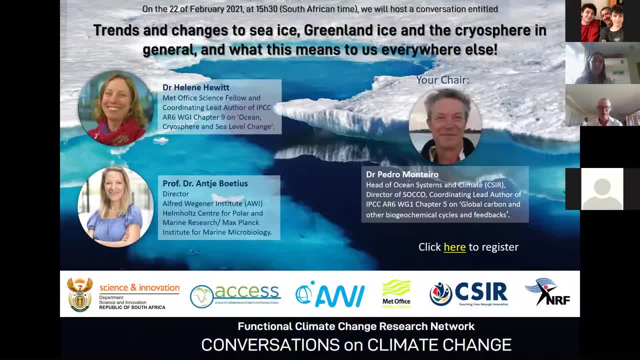 guests who spend a significant part of their research time and space thinking about problems to do with the cryosphere from very different perspectives. So Dr Helene Hewitt from the United Kingdom really comes at it from a sort of physics, physical, climate and physical. 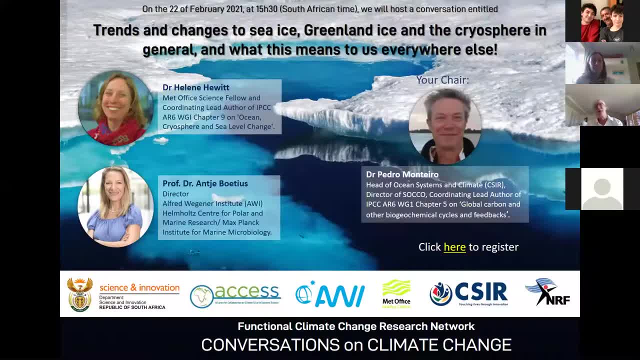 ocean. So the ocean, cryosphere and climate nexus, let's call it that. And Professor Antje Boisius really comes at it from a perspective of the biological implications and in very specific, especially microbiology perspective. So we'll get to that a little bit later when she joins us. So without further ado, I'd like 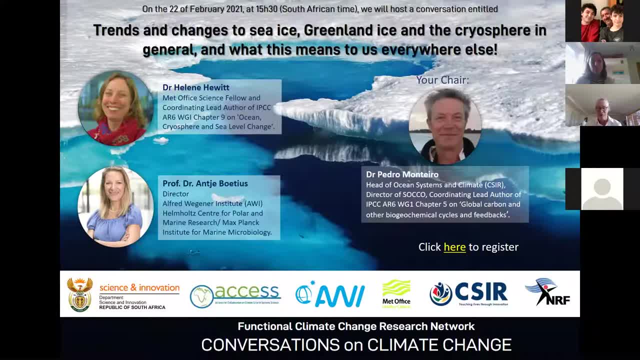 to introduce Dr Helene Hewitt, who's an oceanographer, a modeler in the ocean, climate, space and actually also a colleague in the IPCC, a sixth assessor. She's a science fellow at the UK Met Office and she leads what in the UK is a joint UK. 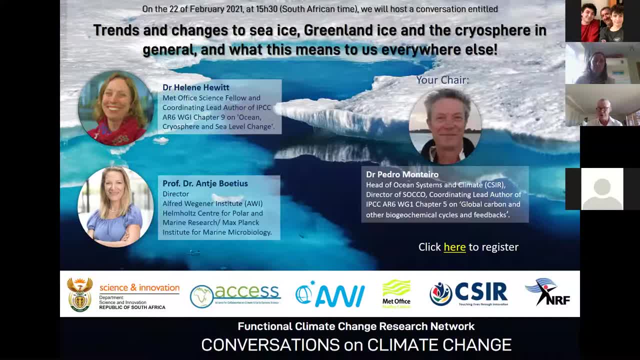 marine modeling program, which is a sort of joint initiative between the Met Office, NERC, which is the Environment Research Council, the NOC, which is an oceanographic center in Southampton, and the British Antarctic Survey, Dr Helene Hewitt. 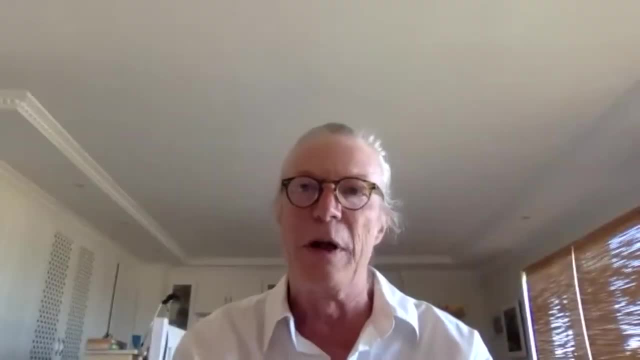 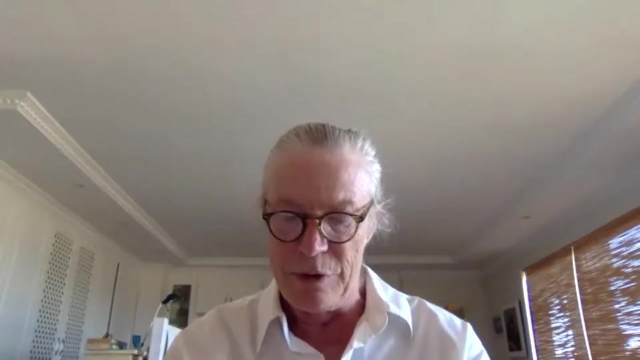 And so these institutions collectively have created a series of models, developed and set up a series of models and modeling platforms that are available to the community, And it's a kind of an indication of the amount of effort it takes to put this together that it's a multi-institutional effort. 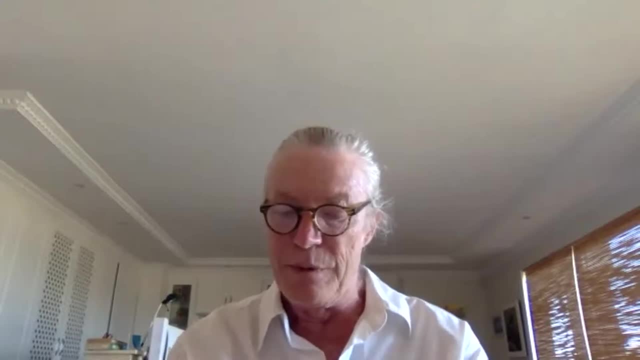 So she's going to be talking a little bit more about this. She's going to be talking to us about the Greenland ice sheets specifically, and its changes and its potential implications for South Africa. So, Helene, I pass it over to you now. Thanks very much. 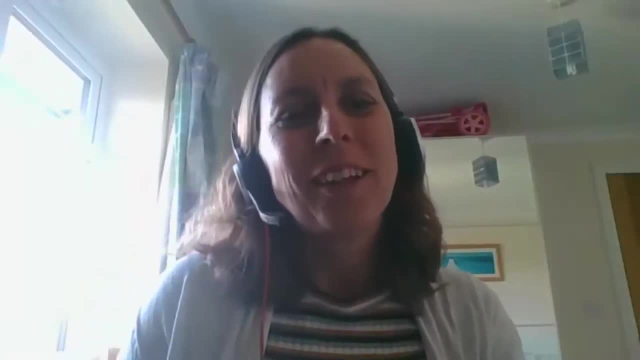 Thank you, Pedro, for a kind introduction. What I'll do is I'll just share my screen first, and then I can talk rather than talk. Thank you, Pedro, for a kind introduction. What I'll do is I'll just share my screen first, and then I can talk rather than talk. 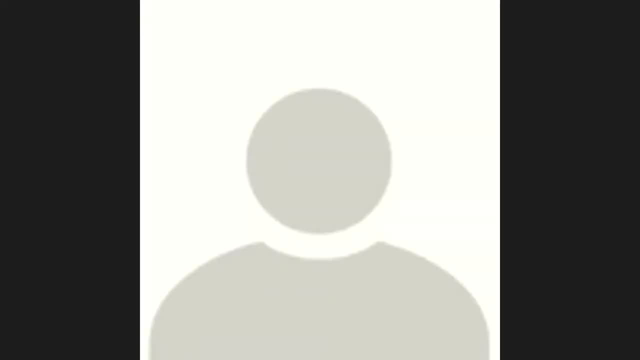 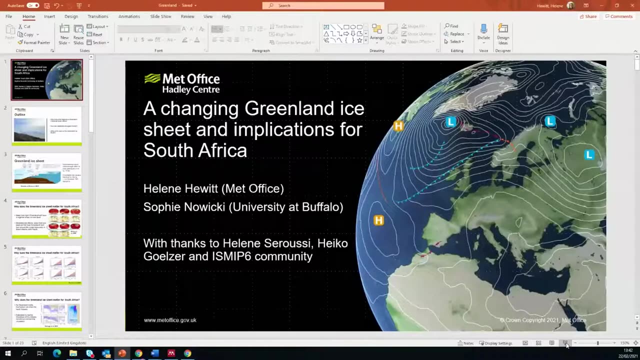 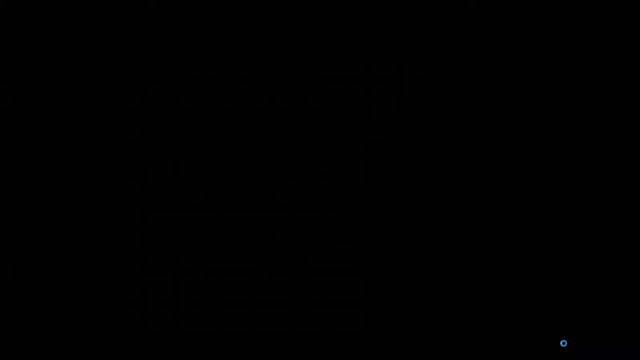 Okay, so I will just try and multitask on this. I'll try and multitask on this. Okay, perhaps Neville can tell me if that looks okay. Okay, perhaps Neville can tell me if that looks okay. Yep, it's on its way over. 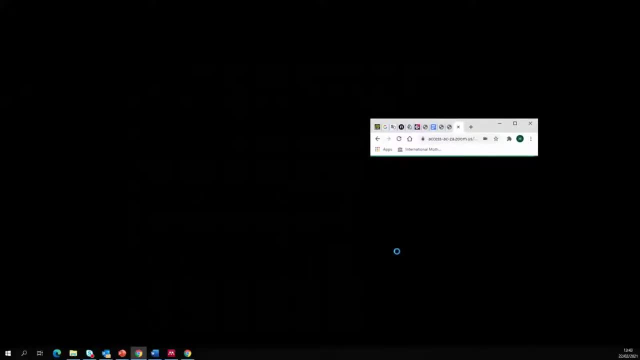 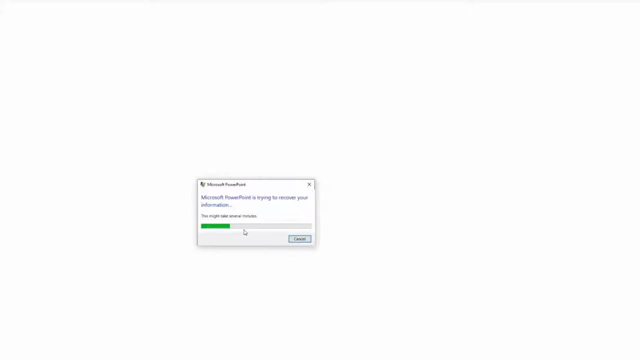 Yep, it's on its way over. I at the moment have a black screen, but I think something's coming. I at the moment have a black screen, but I think something's coming. okay, powerpoint's not happy. it was all fine when we tested it, okay, well, um, while i'm just um waiting for that to uh restart. 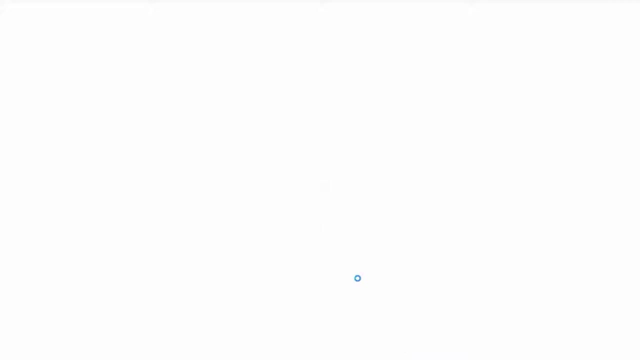 um, okay, so, um, i'll just i'll just talk while that's restarting. so, um, thank you for inviting me. so, as pedro said, uh, i work at the met office hadley center. i work a lot with um colleagues, um in the uk on modeling. my background is um, originally in oceanography. i i did my phd actually. 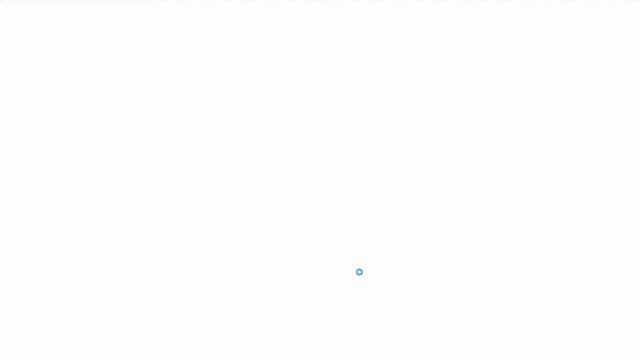 on the equatorial pacific, uh, but increasingly i've moved out to the polar latitudes, uh. so i've worked on sea ice and now also on ice sheets. i'm the one of the coordinating lead authors of the um chapter nine of the uh sixth assessment report, and that covers 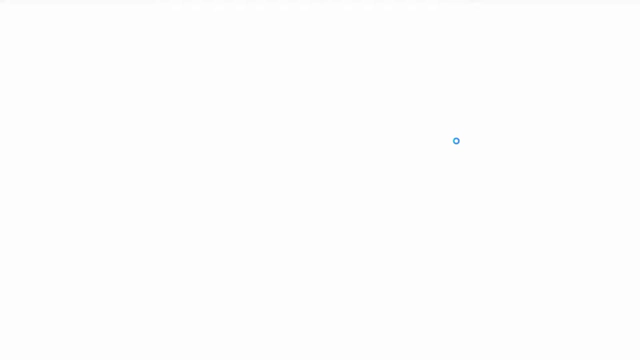 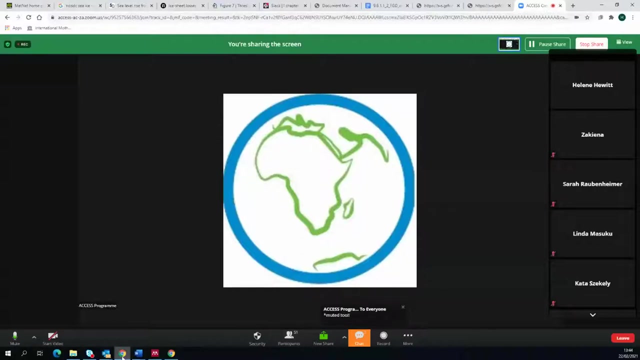 uh, so we're assessing their oceans, the cryosphere, so sea, ice, ice sheets, permafrost, um and also um, uh, yeah, and and uh, also sea level as well. sorry, i'm slightly distracted by trying to set up my computer as well. you try and get it going. 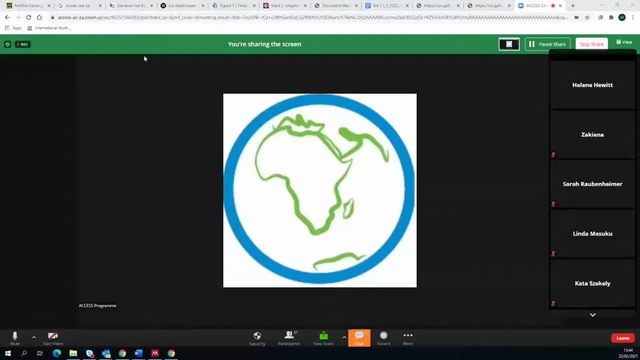 try and get the the powerpoint going and we'll take it from there. so take your time. yeah, um, and so, um, neville asked me to to give this talk and, uh, we agreed that i would. i, i agreed that i would focus on the greenland ice sheet, so what i'm going to do is very much a. 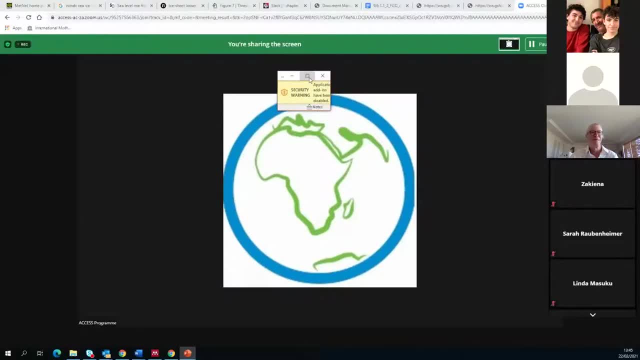 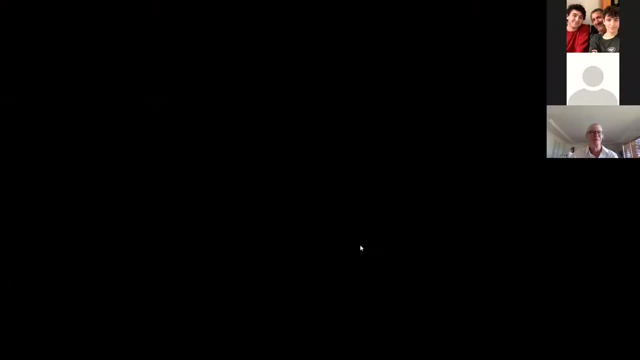 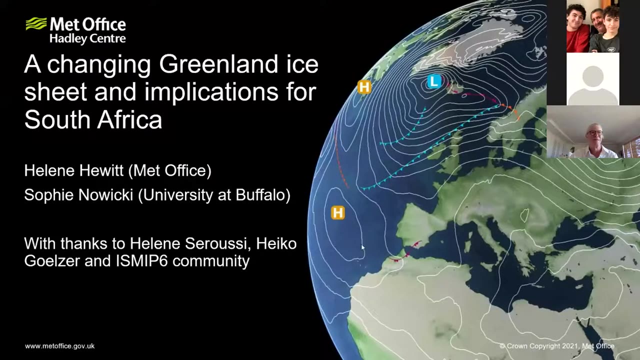 an overview talk here of the some of the latest um research on the greenland ice sheet, um and trying to put it into context: uh for you, okay, can you see that? now you've got that, thanks, okay, so great, okay, now i can start for a proper uh, so, uh, so hopefully. 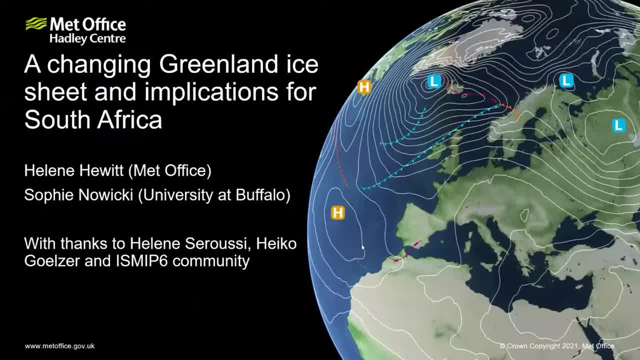 i'll cover some of the implications for south africa. i just wanted to uh acknowledge sophie novicki, who's uh one of my uh co-authors on ipcc and the leader of the ismip six project, which i'll talk about, and uh other people in ismip 6, particularly helene cerisi and uh. 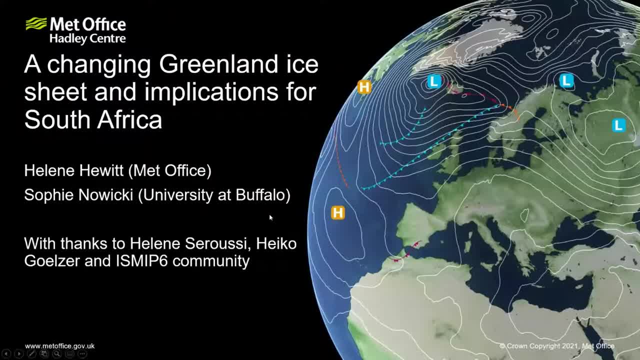 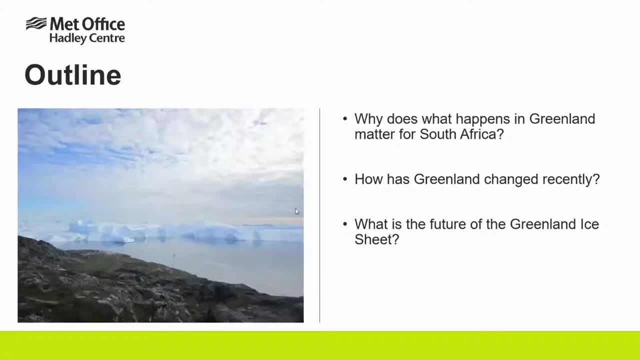 haiko golza. who've uh who? whose slides uh sophie has shared with me, so here's a picture of the greenland ice sheet and uh. so three things that i hope you can take away from from this. uh, short talk is uh. why does what happened in greenland matter? for 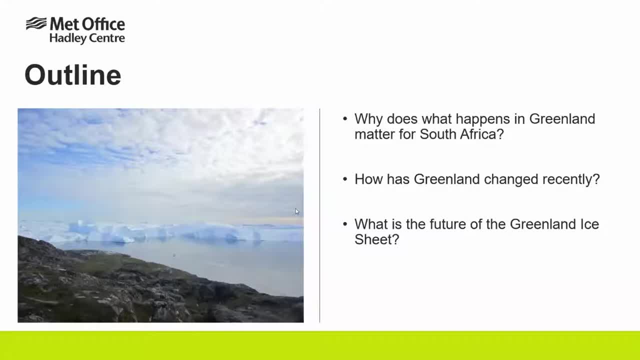 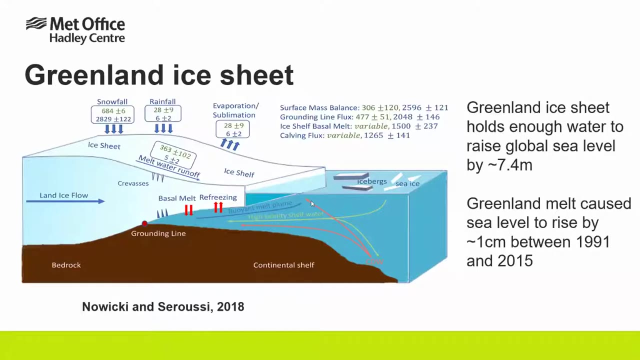 south africa, ismip six, and how can it help to improve climate change for the, for the, for the south africans, Africa? How has the Greenland Ice Sheet changed recently And what is the future of the Greenland Ice Sheet? So this is a schematic. well, it's a schematic that applies not just to the Greenland. 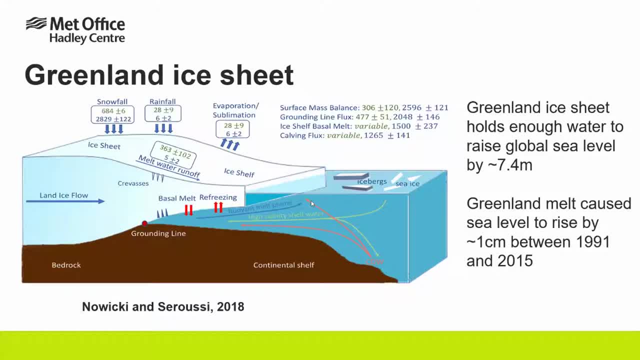 Ice Sheet, but also the Antarctic Ice Sheet. But for now, if you concentrate on the green numbers, those are the ones that really apply to the Greenland Ice Sheet and the others are for Antarctica. So the Greenland Ice Sheet is a huge mass of frozen water. If it melted instantaneously. 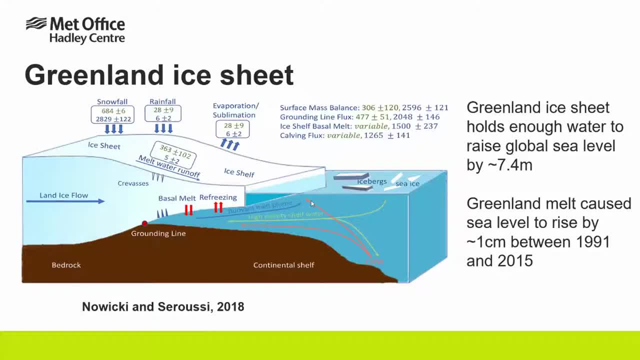 it would raise global sea level by about seven- almost seven and a half meters Between 1991 and 2015,. it raised sea level by about one centimeter on its own And the main balance in the Greenland Ice Sheet is really by between the surface mass balance and 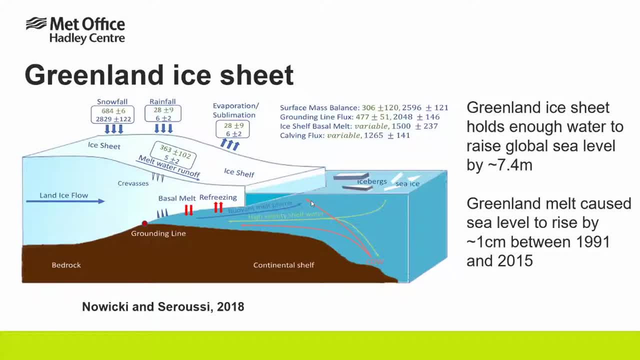 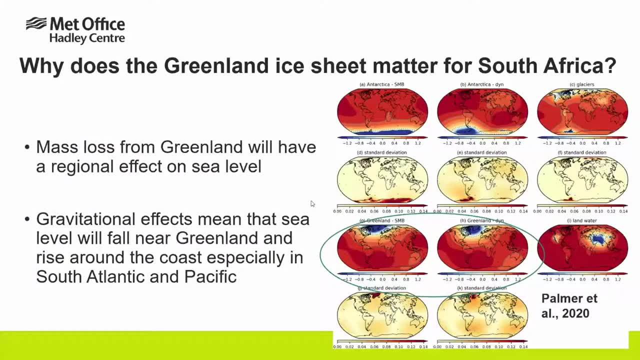 the flux past the grounding lines. And so I thought I'd ask- I just kind of turn it around first and talk first about why the Greenland Ice Sheet might matter for South Africa And the reason for the reason why it matters. I mean I could have written on here that actually will. 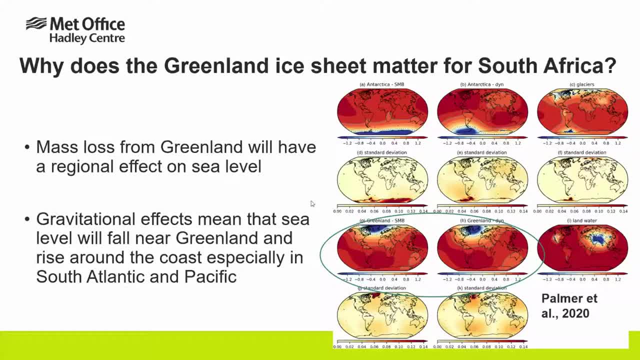 affect global sea level. So that will affect, affect everybody, But in particular for South Africa. what happens when, when you lose mass from from the ice sheets and the glaciers, is they have a regional effect on sea level And the gravitational effects actually mean that closest to the source. 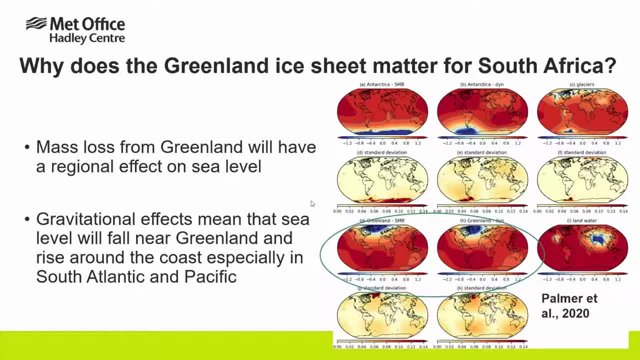 sea level will go down, whereas away from the source sea will sea level will will rise more. So if you look in this figure here, I don't know that you can see. Can you see my mouse? Hopefully you can see. you can see where I've circled these plots from a sea level projections. 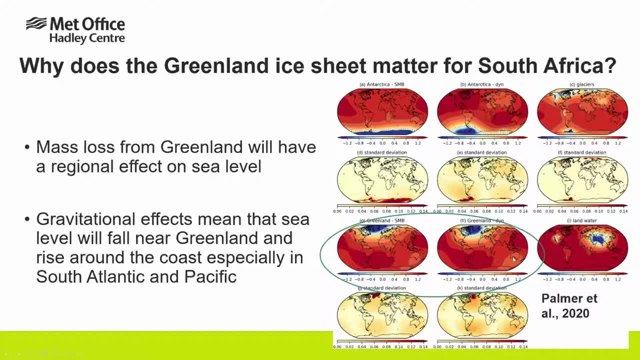 paper by Matt Palmer and co-authors And they show the the ratio of the local contribution to the far field contribution. And they show the the ratio of the local contribution to the far field contribution. And so you can see that that for the Greenland Ice Sheets, when, when ice is is lost to the to the ocean. 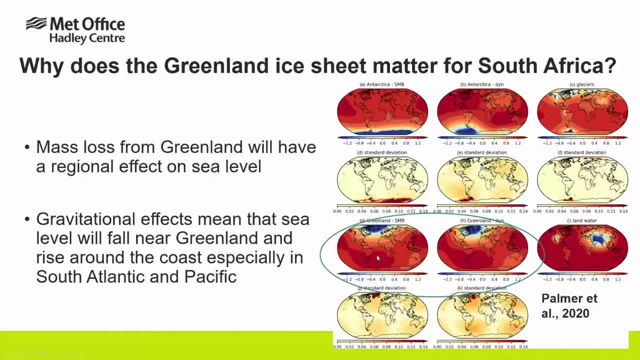 sea level actually dip down slightly close to Greenland, but in you know, around South Africa and the Southern Ocean going up into the Pacific, it will actually have quite a strong far field effects And you know, you can see that if you compare this with Antarctica, for example, this is: 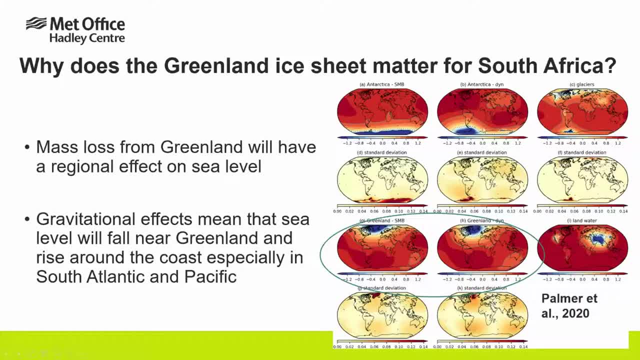 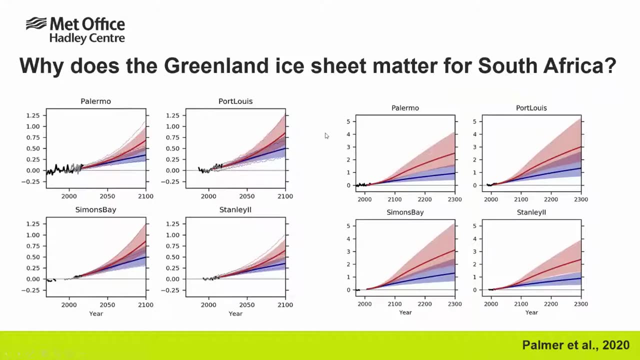 very different. So for us in the UK, for example, Antarctica might have a smaller effect near Antarctica itself and a much larger effect up to the north. And so if you then look at sea level projections- and in this case I'm showing them for 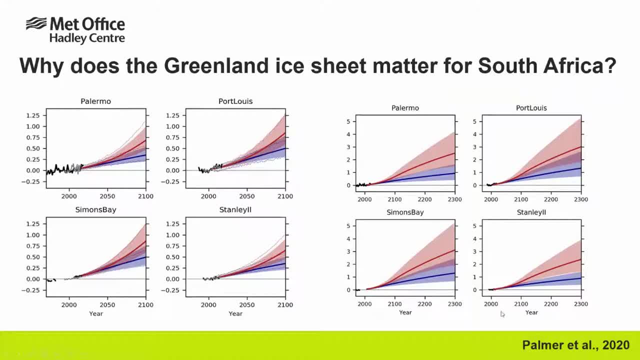 four locations from the paper by Matt Palmer. So in this, so Port Louis and Mauritius, Simons Bay, which is near Cape Town, I believe, and Palermo and Stanley, which are over the other side of the Atlantic. then you know, you can see that out to 2100, we're looking at. 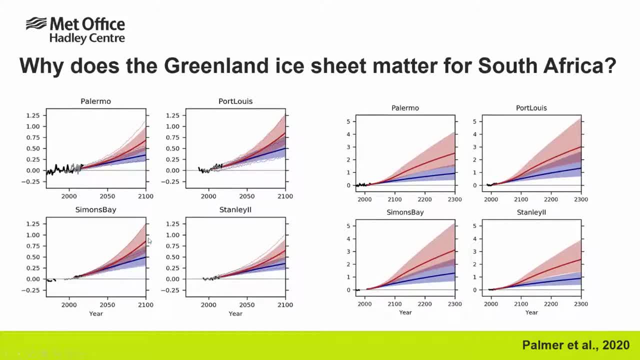 getting to 2100.. So we're looking up between 0.75 and a metre in the highest projections. So the red line is the RCP 8.5, which is one of the highest projections, And the blue line is RCP 2.6.. 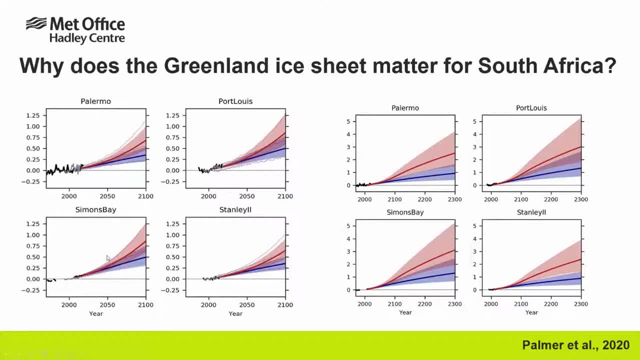 And you can see that you know for Port Louis and Simons Bay they're quite similar, Perhaps a little lower in these other two examples. So you can see the regional effect there And more pronounced even when you look out to projections to 2100. 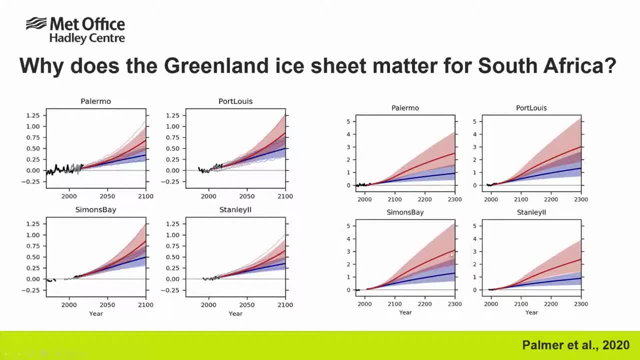 When we're looking, when it's projecting up to a median of three metres in Cape Town, going up possibly to five metres. even So, there's quite strong effects And you can see this is. you know, Port Louis and Simons Bay are much higher than the other two out. 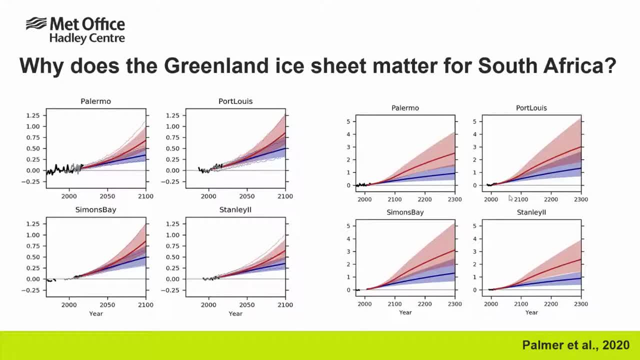 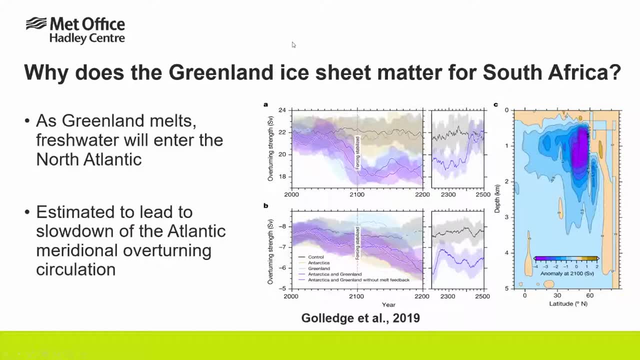 to 2300.. So it is important from a sea level point of view, both globally and regionally. Another reason that you might be concerned about is in the Atlantic. obviously, the ocean circulation- for people who aren't oceanographers- is driven by what we call the Atlantic meridional. 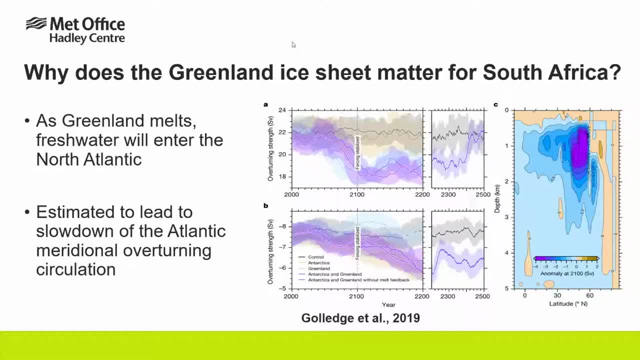 overturning circulation So that has strong warm water northwards, it sinks in the northern hemisphere and travels back southwards And that transports heat northwards throughout the Atlantic. And so, as the green line goes up, it's going to be a lot of heat, And so it's going to be a lot of. 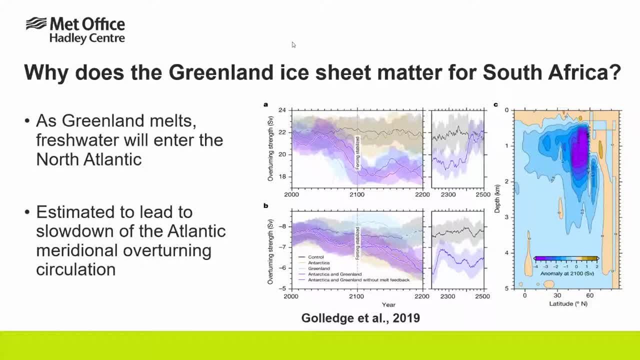 ice sheet melts, that will put a large amount of fresh water into the North Atlantic, And additional fresh water in the North Atlantic can have the impact of shutting off convection in the North Atlantic region and then slowing down the meridional, overturning circulation. 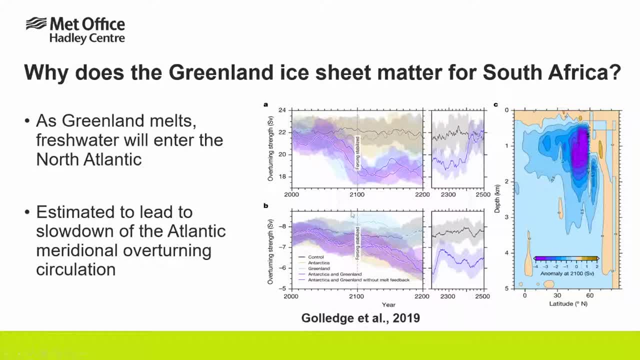 So, if you look in, here's an example of this from a paper by Nick Gulledge and others. And so what they do is they take the ice sheet and melt it And they put a large amount of on dried snow on the ice sheet and they allow the atmosphere for getting much better. So what? 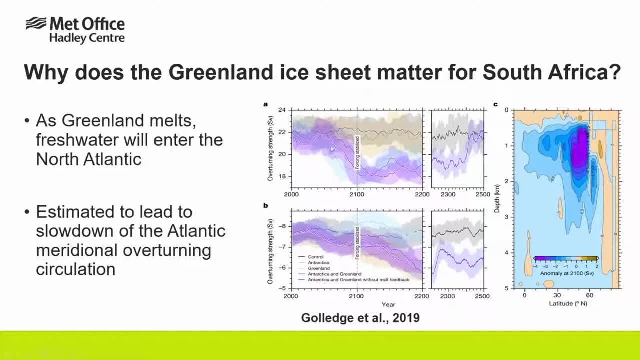 they did? there was the. they allowed the Greenland and Antarctica to melt in different experiments. But if we focus on the Greenland experiment, for example, and you look in the top panel, which is the upper part of the overturning in the top few thousand meters of the ocean and which does 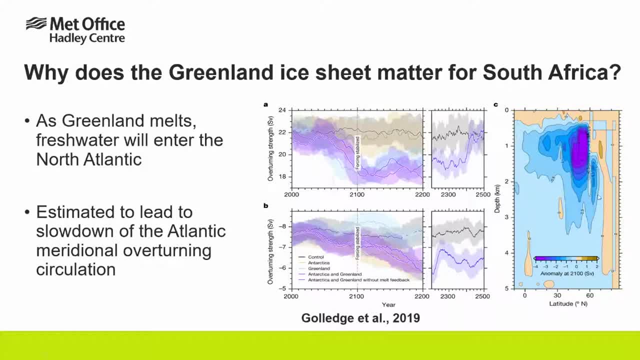 most of the heat transport northwards in the Atlantic. you can see, if you look at this, the light blue line which I'm pointing to here, You can see that when Greenland melts it has an impact on the overturning circulation. 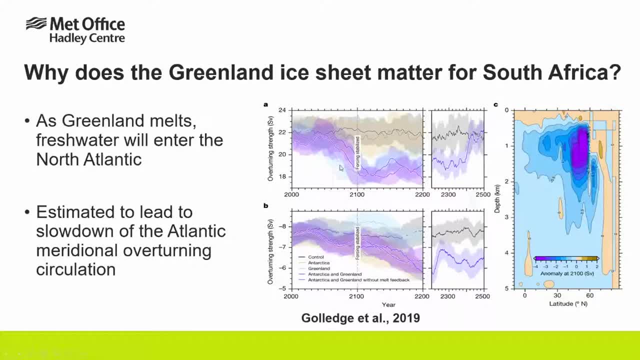 So you can see here, as Greenland melts it's shutting down the circulation from 22 sverdrops down to 18 and below And then later on it's able to recover as it stabilises. And you can see this impact. I mean it's very strong in the North Atlantic, shutting down the circulation. 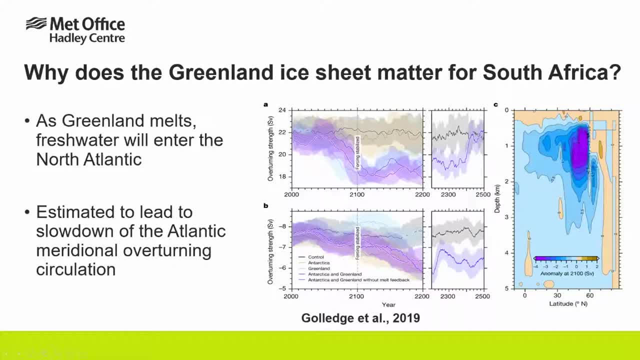 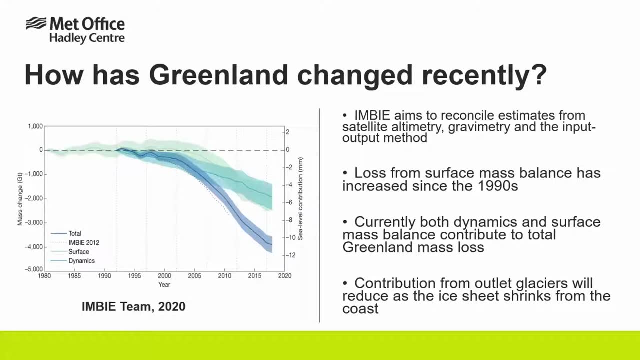 But that's also extending into the Southern Hemisphere as well, So that would have impacts in the South and the North Atlantic. but also the AMOC has an effect globally on climate. So how do we think? how have we seen the Greenland ice sheet change recently? 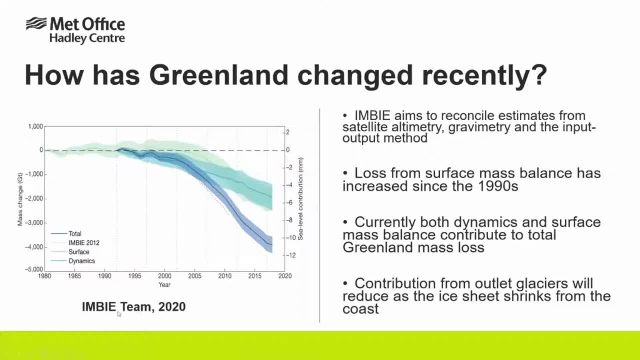 So these are results from a paper by the IMBI team which was published last year. So IMBI is a project which aims to reconcile estimates from a number of different sources measuring the ice sheet, So from satellite, altimetry, the gravimetry and the input output method. 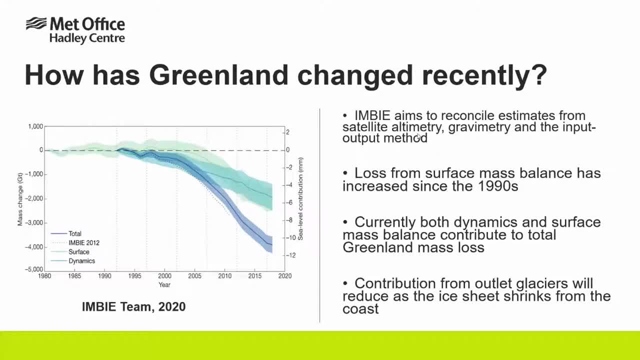 And these are put together for a consolidated estimate. And so what you can see is You can. you can see in the dark blue the total loss of mass from the ice sheet from the 1990s to the present day. You can. if you look at the green line, you can see that in the 1990s the surface mass balance was was approximately close to zero. 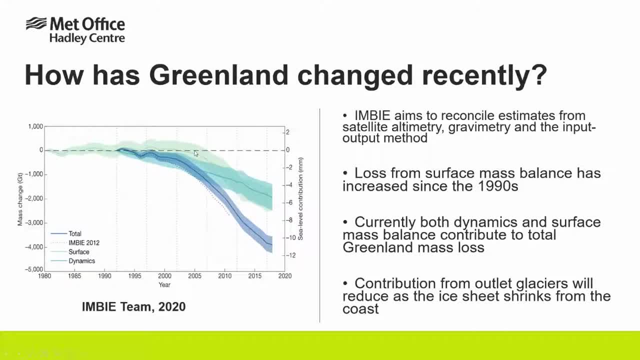 And that's since about 2005 onwards. That's that has declined And prior to that there's been decline of the ice. So the ice sheet from the, from the dynamics, So at the moment it appears there's a contribution from both effects. 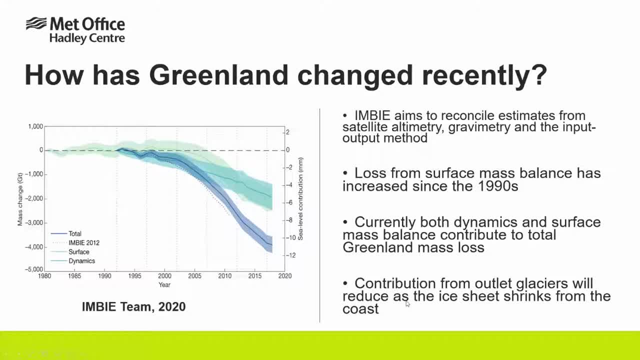 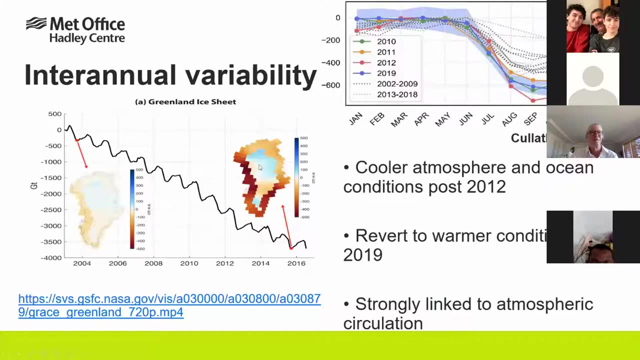 But as the ice sheet shrinks away from the outlet, away from the coast, the contribution from the outlet glaciers will reduce much more and there'll be- there'll be, more melting and runoff there. So here's a. what I want to show you here is a. this is a figure. 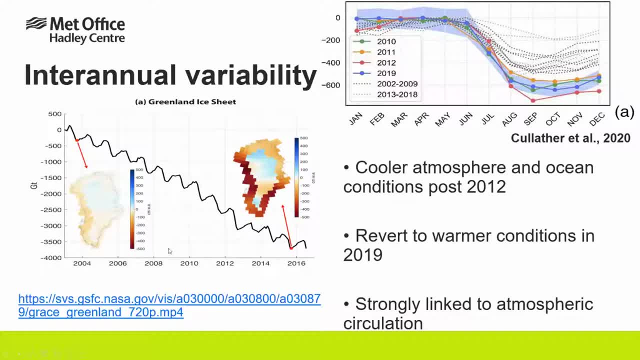 And I'm going to show you a picture of the ice sheet. And I'm going to show you a picture of the ice sheet. I'm going to just quickly show you the video, if it works, which was produced from NASA, And you can see the evolution of the the ice sheet from 2003 onwards. 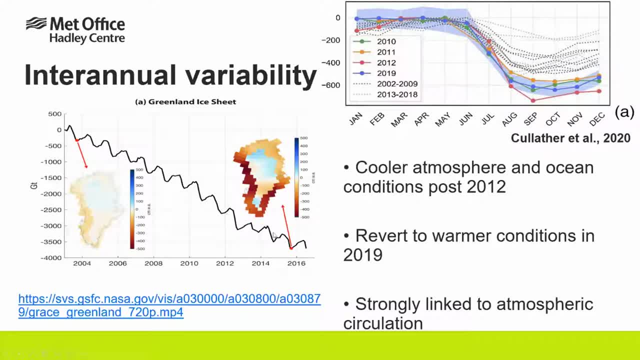 You can see there's a seasonal cycle, but you can see this large decline And what you see is that around 2012, it moves to cooler conditions, So there's less ice loss And this doesn't quite continue to 2012.. 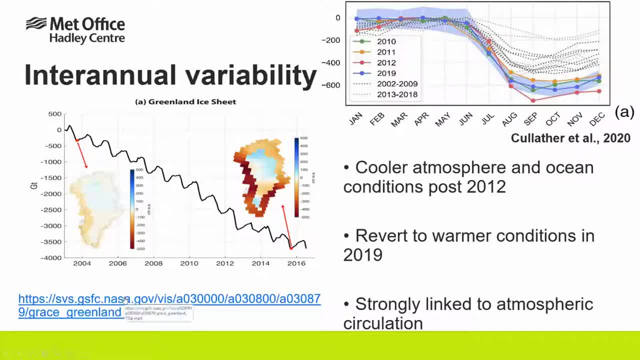 And this doesn't quite continue to 2012.. And this doesn't quite continue to 2012.. But although you'll see in a minute from the other picture that it picks up again then, So hopefully this is going to work now. 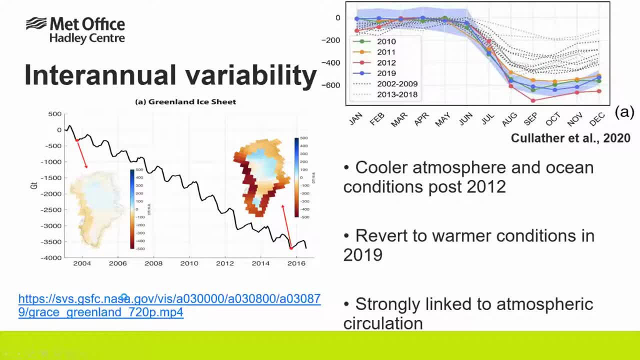 It did work for me And we both. it did work in our trial. OK, well, well, that's so I'll just say So. here's a plot which is showing. this is to show the the interannual variation You can see. 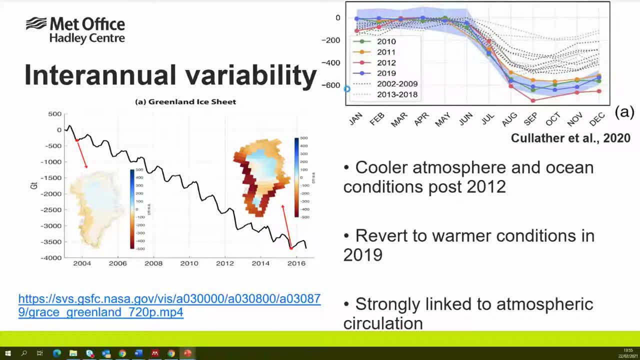 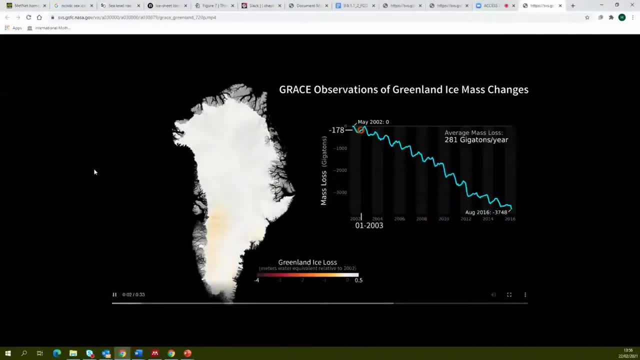 This is the, the mass loss on the axis here, And, OK, it's going to work, Great, OK. so here this is a video and you can see in the circle here it's showing you. we're tracking the, the total loss. 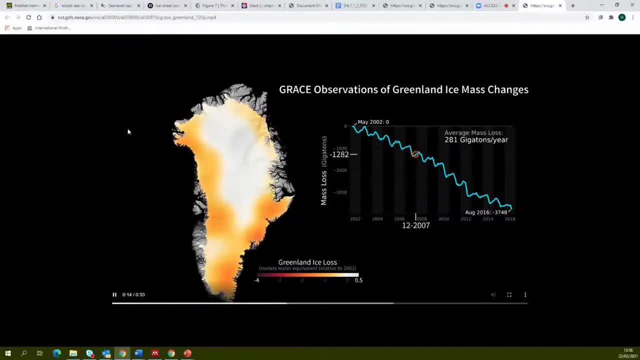 And the map is showing you where that loss has occurred. So you can see now, as we're moving into the the late 2000s, large loss at the Around the coast, particularly in the southern and western regions, And that's really intensifying as you get down to 2016.. 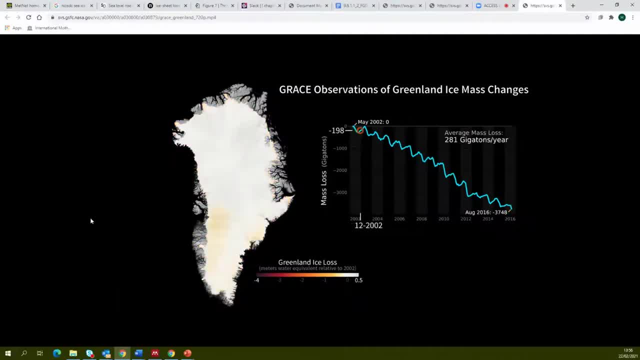 I'll just show you that once more. So here you can see it gradually building up in that south southwestern area, near where there's glacier outflows, And it's intensifying as it goes through. And it's intensifying as it goes through. 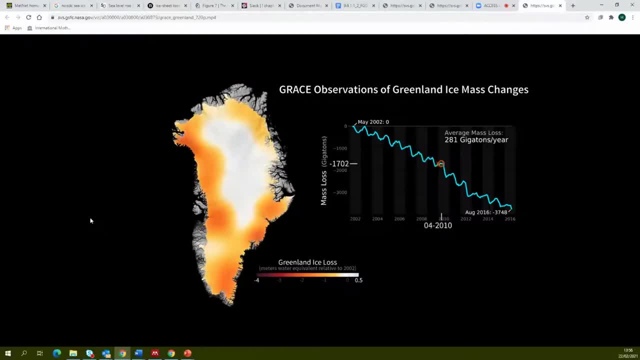 And it's intensifying as it goes through, So that you can see that strong seasonal cycle. You can see as we come up to a large loss around 2012.. And then you can see it slow down a little as we move to warmer atmospheric conditions. 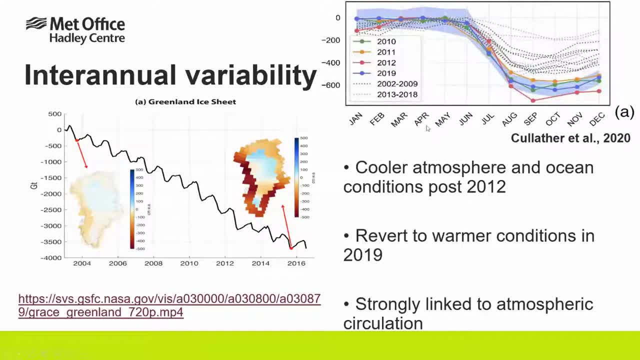 That was on the side. I wanted OK, and, and. so if you look in the top panel You can see how this varies from from year to year. You can see the loss in 2012 was very large, much, you know, intermediate in 2010 and 2011.. 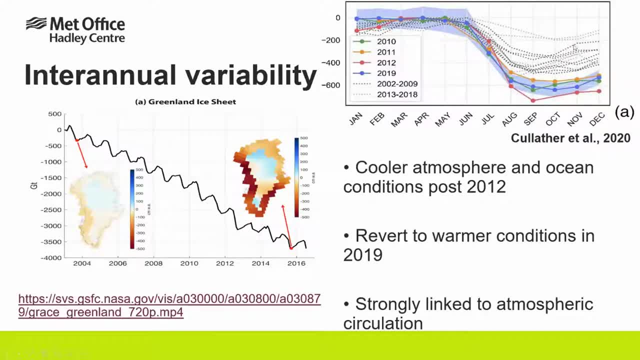 Then after 2012,. much less loss generally until 2019 when it reached the 2000.. And almost a year Than when it's almost half way through 2010, 20 and 10 levels. So you can see that into. 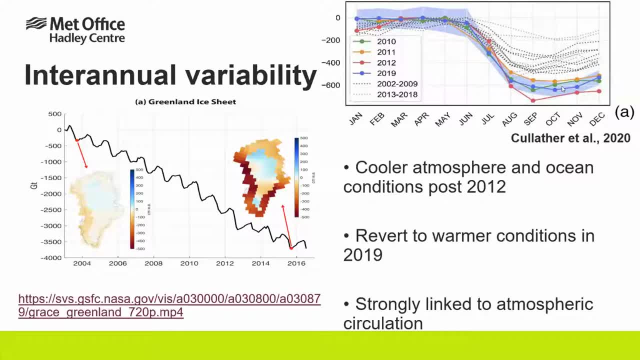 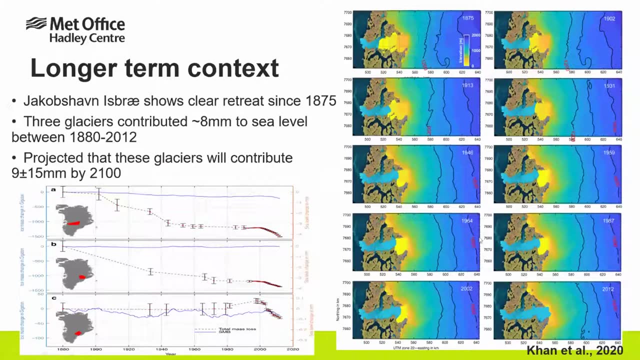 Annual variability there and this is strongly linked to to atmospheric circulation. It is a clouds in particular as well, so The Annual variability there. This is another recent paper which was produced in nature by Kahn and co-authors, and in this they look, they really focused on three of the glaciers. 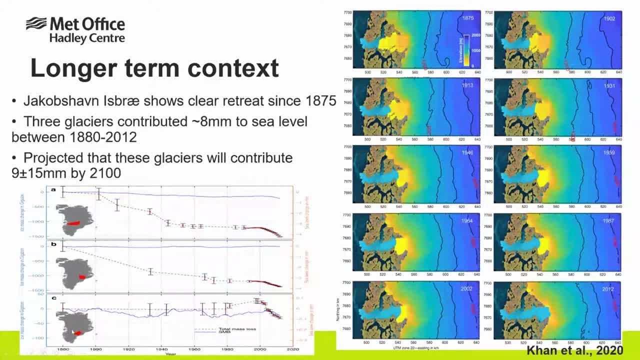 which they were able to look at right back to the 1880s, looking at various sources, including photographic images of it, and so you can see as you look through. so it goes in this direction, across and then down and across, you can see that there was retreat in the early periods. 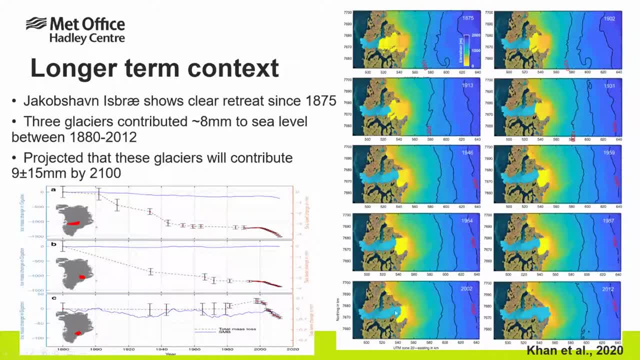 that retreat of, you know, has particularly sped up recently and you can see that here if you look. this is the same glacier here. you know well there was some loss through the the century. there's been a lot of loss in the very recent periods, you know, looking like. 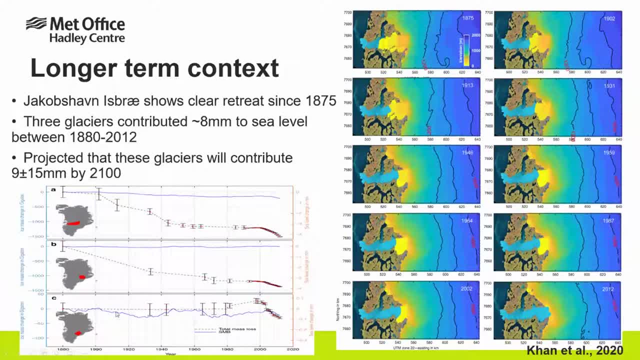 it's some sense perhaps of accelerating, and true also here. so these three glaciers alone contributed about eight millimetres to sea level rise between 1880 and 2012, and it's projected that they could contribute- maybe even- you know- 9 to 26 millimetres by 2100. 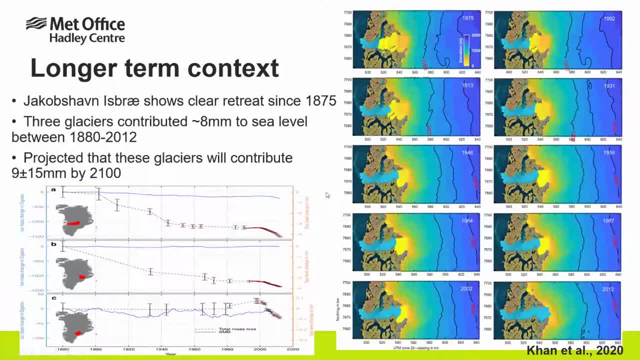 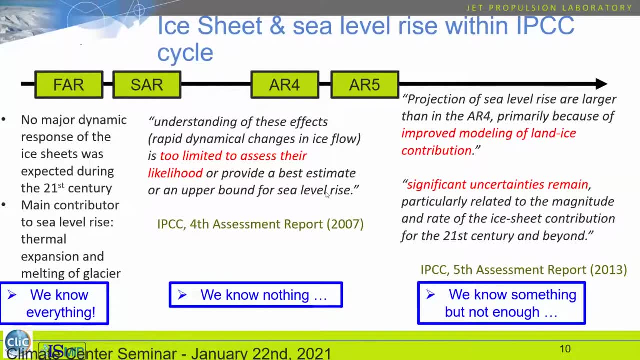 so if you sum that up over large areas that will add up to a lot. so that moves me on nicely to projections. so this is a nice summary that Sophie put together of how we thought, how IPCC thought, about ice sheets and sea level rise. so in the first assessment, 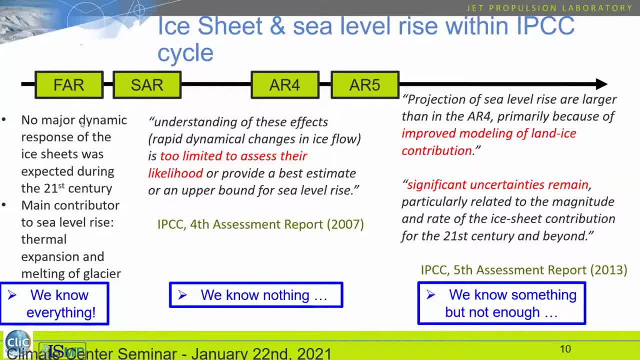 report, the view was that there was no major dynamic response of the ice sheets expected during the 21st century and that thermal expansion and the melting of the glaciers would be the main contributor to the sea level rise. or we know everything about ice sheets and then in by the time we got to the fourth assessment report. 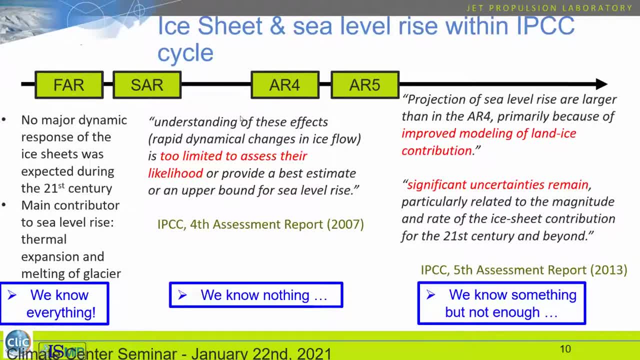 they were saying that understanding of these effects is too limited to assess their likelihood and they couldn't provide a best estimate or even an upper bound for the sea level rise. so, basically, we know nothing. and then, by the time we got to the fifth assessment report in 2013, 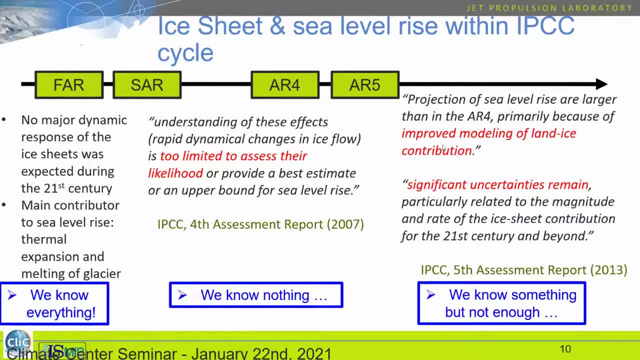 they noted there that there was improved modeling of the land ice contribution, but that significant uncertainties remain, particularly related to the magnitude and rate of the ice sheet contribution for the 21st century and beyond. so basically, you know we know something about the future of ice sheets, but really not enough. 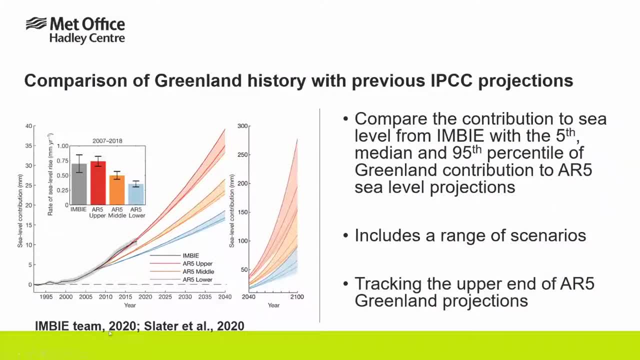 so other work that people have done. recently, the InB team and a follow-up paper by Slater and co-authors looked at how the Тыne and sell green salt-based ice sheets would help with the impact of ice sheet climate change on the environment. 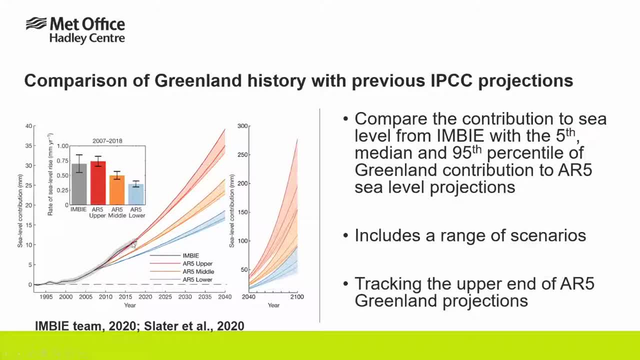 at how the iSheet contributions from INBI compared to those projected from the AR5. So what you're seeing here is the blue line shows the fifth percentile of the iSheet projections from the AR5.. The orange is the median and the red is the upper part. 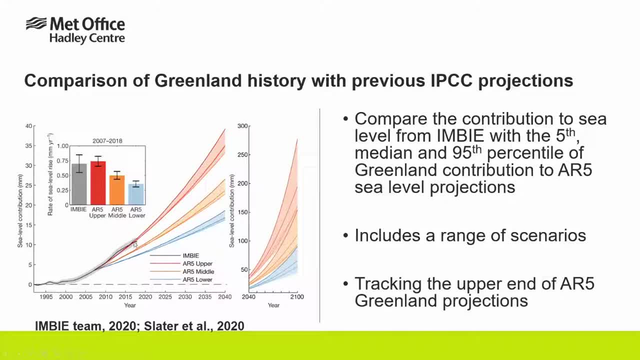 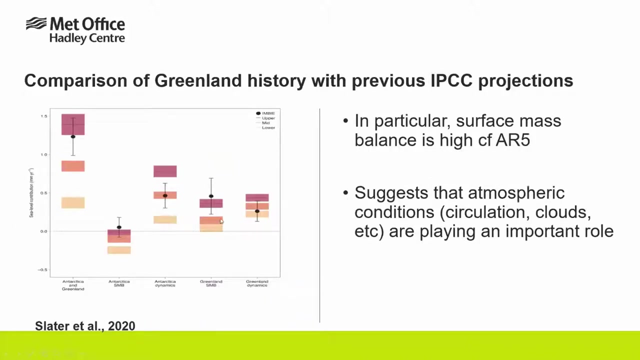 And so you can see that the INBI data appears to have been tracking the the upper edge of the projections in the fifth assessment report, You know, whereas you probably would have expected it to track much more closely to the median. And if you look then at the contributions, you can then see that the surface mass balance here 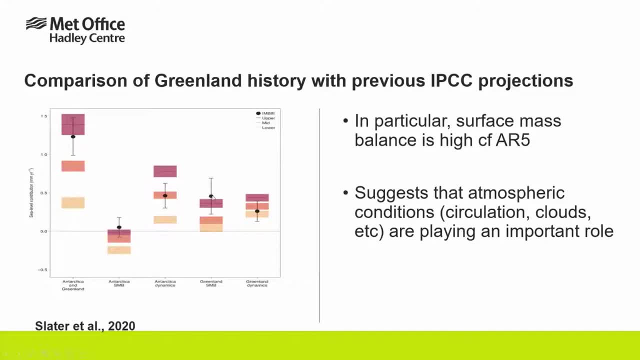 you can see the Greenland surface mass balance. the median of that, or the central estimate from INBI, is outside the upper range there of the AR5 projections, whereas the dynamics is much more, is much closer to the median. So this perhaps fits with the picture that we've seen earlier. 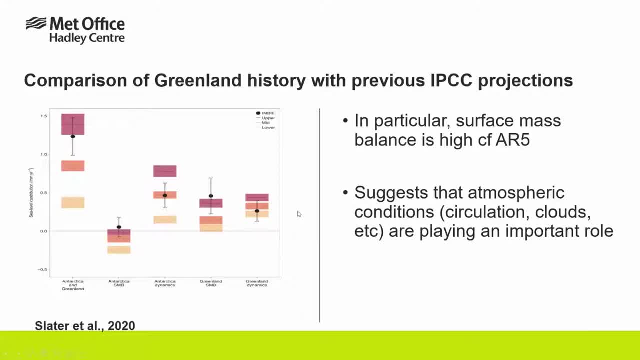 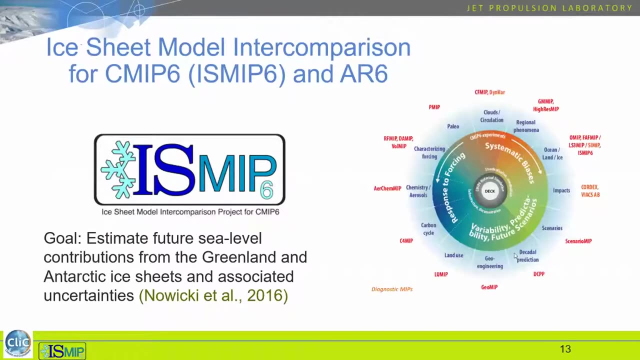 the fact that atmospheric conditions could be playing an important role with the circulation and the clouds, And so that brings us to how we move on from the AR5 perspective, And so In the sixth assessment report there has been a big push on the CMIP6,. 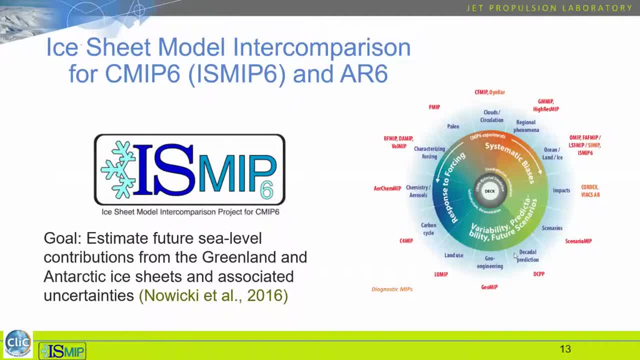 or the Climate Model Inter-Comparison Project, And ISMIP6 is one of those. So that stands for the iSheet Model Inter-Comparison Project, and its goal is to estimate the future sea level contributions from both the Greenland and the Antarctic. iSheets and 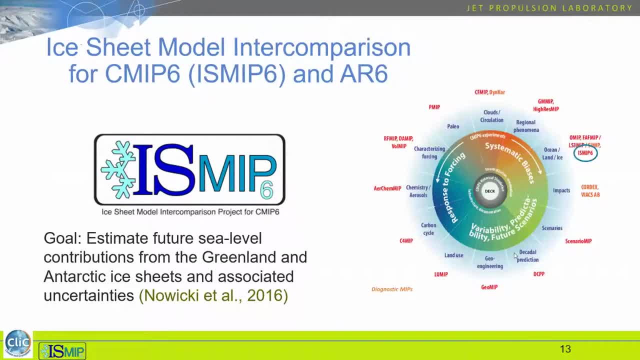 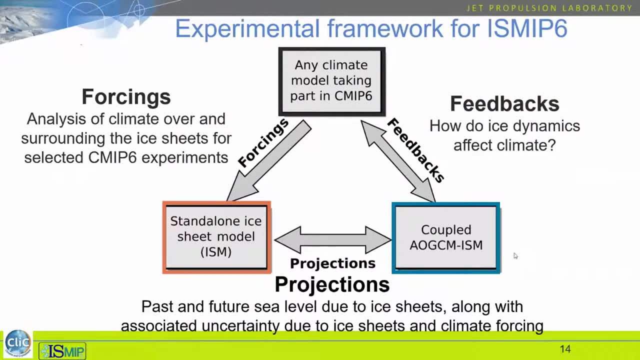 the associated uncertainties, and they have a framework where the forcings are taken from climate models taking part in CMIP6 and then these are used to force standalone ice sheet models, but there are also some coupled models that interactively include ice sheets, and so then you can explore the impact of forcings, the impact of feedbacks and the impact of the 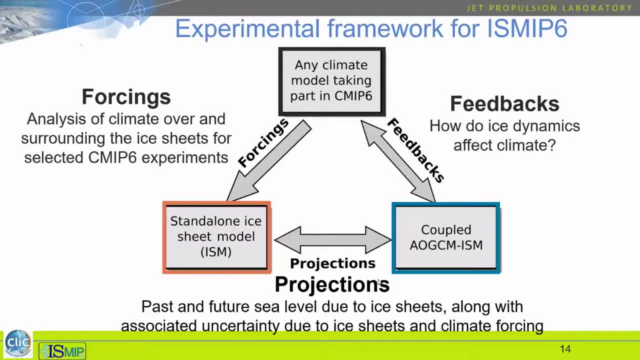 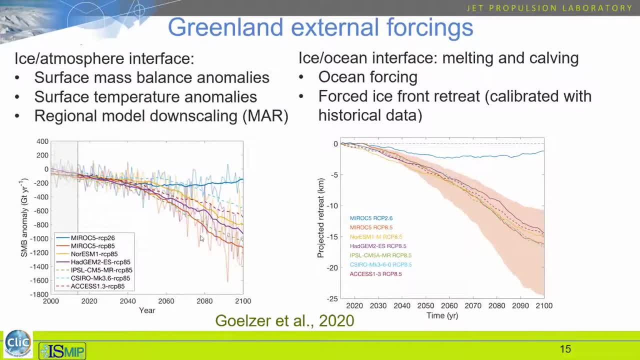 projections. so which scenario, for example? and so what was done in CMIP6 for Greenland was that a selection of the CMIP6 models were chosen to try and encompass a whole range of models and and futures. so this shows you mostly us. well, these are the bottom. 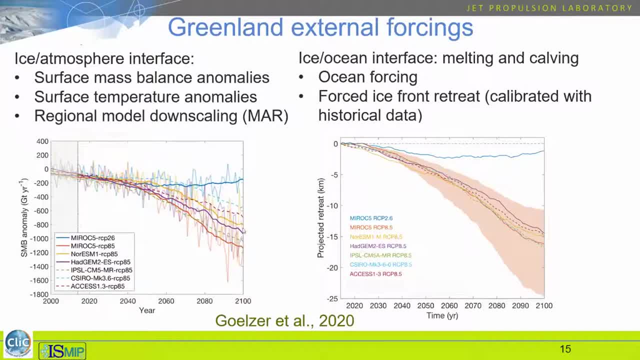 lines are all RCP 8.5, so a high emission scenario and they chose one low emission scenario for comparison. and and these were also used for the ocean forcing and it gives projected retreat of of the ice sheets and you can see obviously it's much higher with. 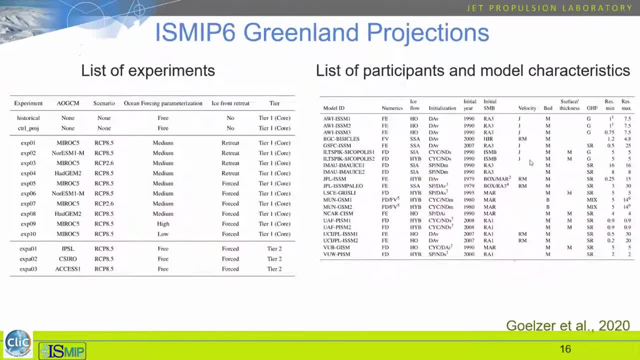 8.5 than 2.6. this is- this slide is really to ship, to kind of emphasize the huge amount of effort which goes into these, these models. so there was a series of experiments, so so 10 experiments and and three extra experiments which were run with a range of different forcings. 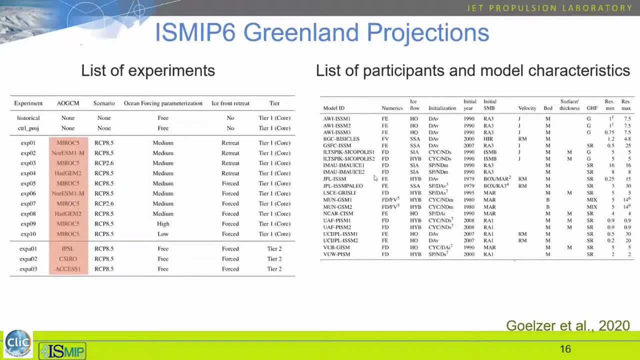 and each of these were applied to the different ice sheet models. so you can see the there's a whole range of ice sheet models. they have different types of dynamics included, different types of initialization. there is a range in the initial years that were chosen and a range also of resolution. so some very high resolution ice sheet models, some much. 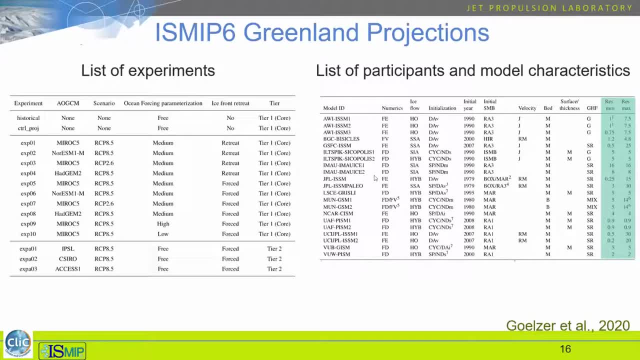 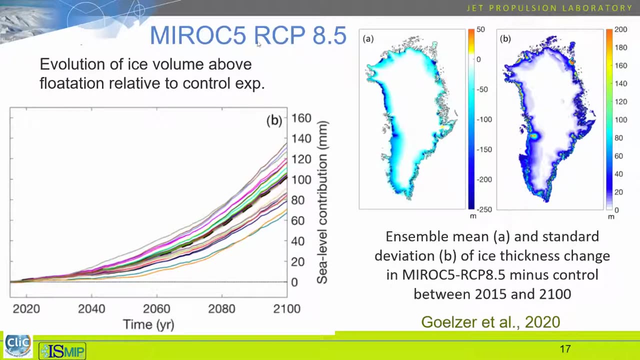 lower ones. so the lowest is 16 kilometers and high, the highest can be, you know, really sub kilometer in places. So this is a slide showing the comparison from from one model at 8.5, and you can see that all the ice sheet models- this is the different ice sheet standalone models- simulating. 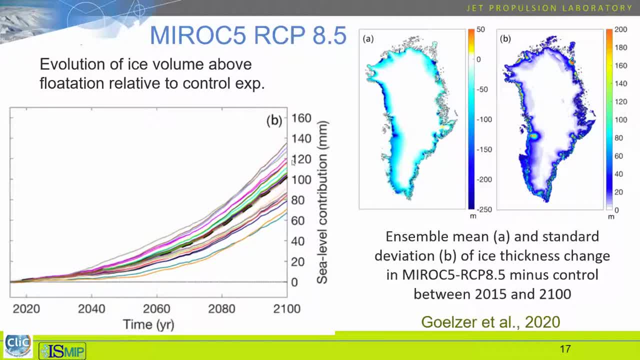 that scenario and it gives a large range in the projections. fairly large rain though they all project they're going to lose ice and you can see that the ensemble mean is showing the loss around the edge, But the standard deviation is also still quite, quite large across that, those scenarios. 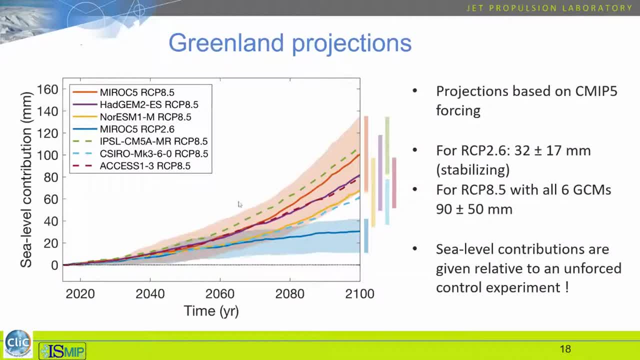 And so this was done for the different models and also for the 2.6 scenario. so you can see the 8.5 scenarios all show show large loss, less so for 2.6. so that is what we would expect, but it does vary a lot across the forcing models and the relative to an unforced control of the. 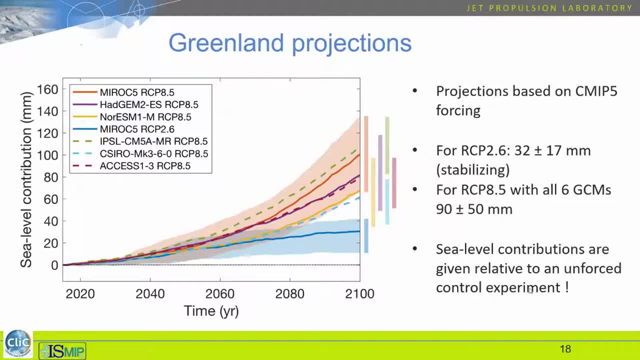 control experiment and that's that's quite important because there's some loss already locked in. but from the initial conditions, the 2.6 model projects something like 32 millimeters across the ensemble, whereas the 8.5 is projecting about 90 plus or minus 50 millimeters across. 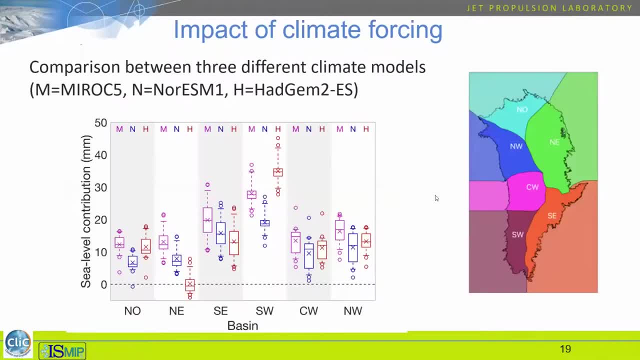 these six GCMs And then you. you know that in the ISMIT 6 community they've then looked at where the, how much variation you get due to the climate forcing, which is quite a lot and also quite regional, particularly in the in the southern areas and the central west as well. 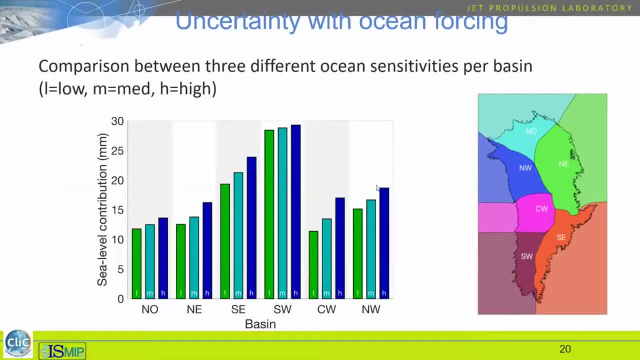 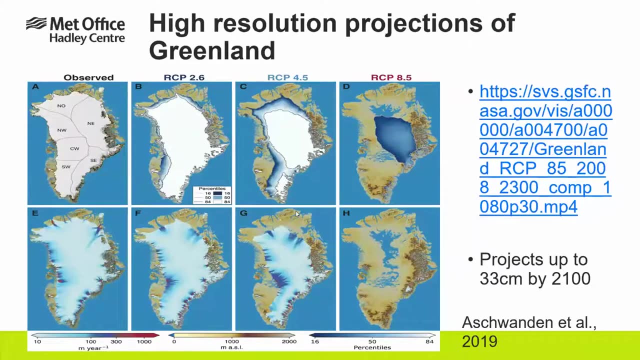 And there's also uncertainty associated with the ocean forcing, which is also regionally dependent: how much, depending on how much that area is influenced by the ocean. So those are these six projections, And then there are other projections which have been done. this is by andy and co-authors and this is a very high resolution model of of greenland and they actually ran this out to 3,000 years. so in the summer, When you think, is it daily? so we've got state trends 2017. 4, the 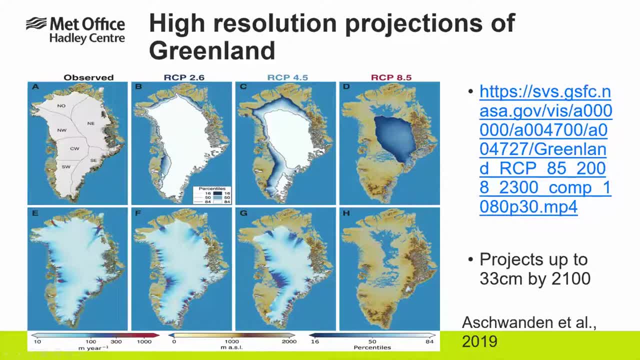 green countries and Andi shvon in and and co-authors, and this is a very high resolution model all for of Greenland and they actually ran these out to 3000 years. so in these Andism ex urged ours toати 30 years. 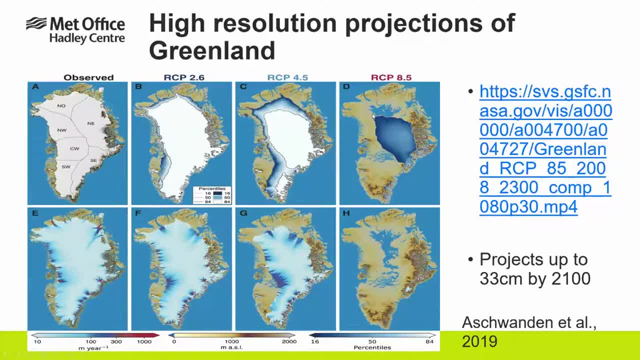 That's what some we do in the summer, when We just different In the spring gene and a five record. So in the spring That's got here 2300, perhaps it's year 3000.. And you can see very high losses in 8.5 and much lower in the. 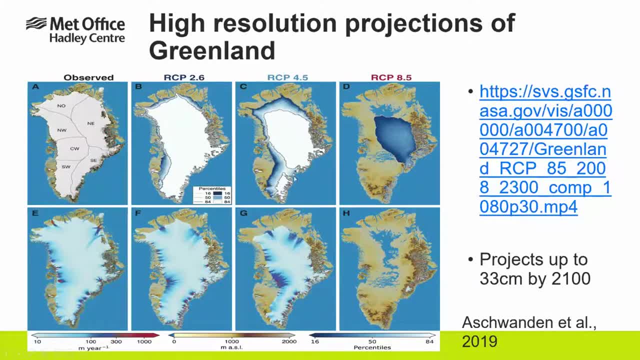 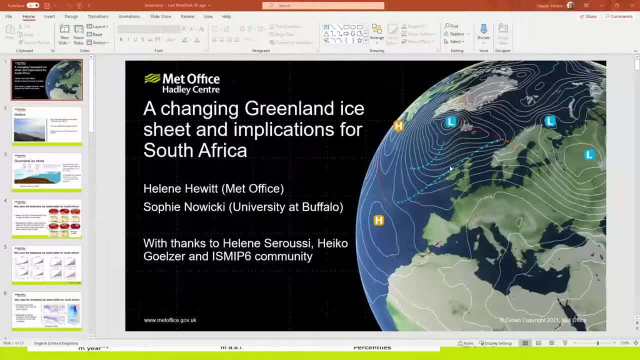 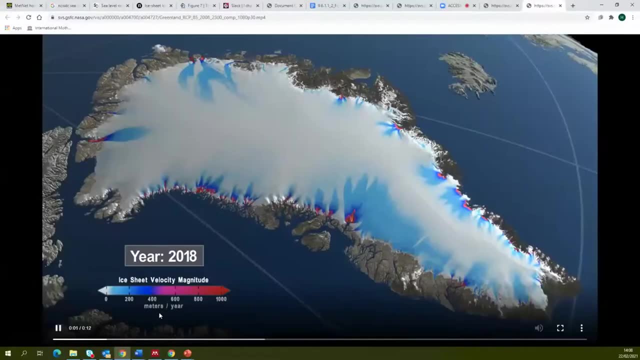 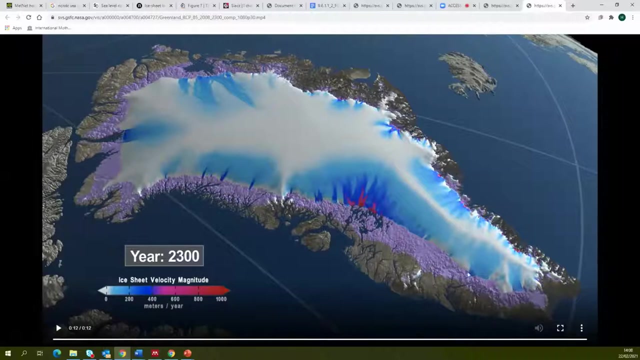 lower emission scenarios. And here is another video from NASA which hopefully will work, And you can see how that then evolves. So you can see in this- this is just a very short video, but you can see at this very high resolution the ice loss at 8.5, moving very fast along this, particularly in this central west, and 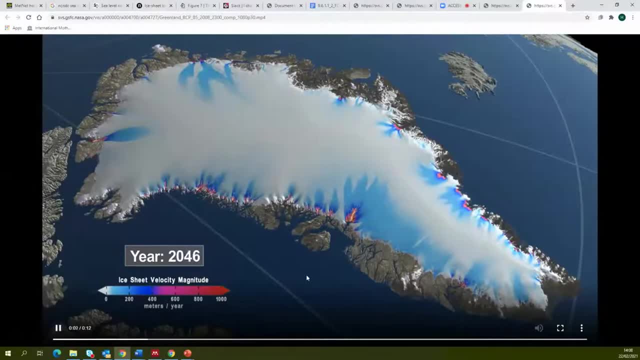 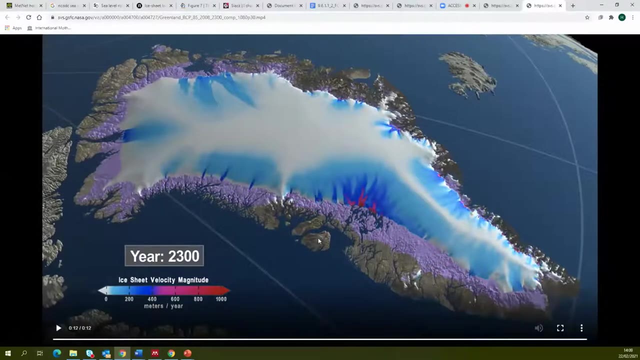 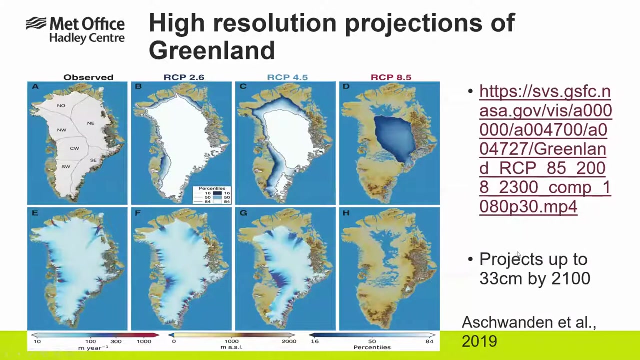 southwest coast here. So if you see it again, you can see these are these outlet glaciers here. And you know, compared to where we were in AR5, you see, ice sheet modeling has advanced dramatically in that time, And so this- this is this- is probably viewed as quite a sensitive model. 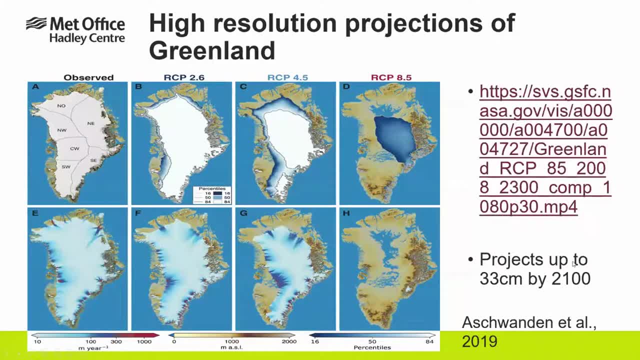 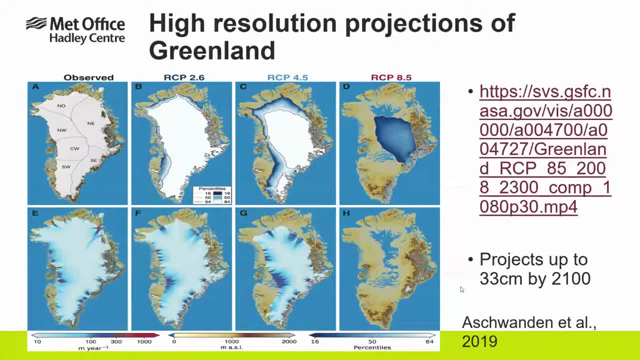 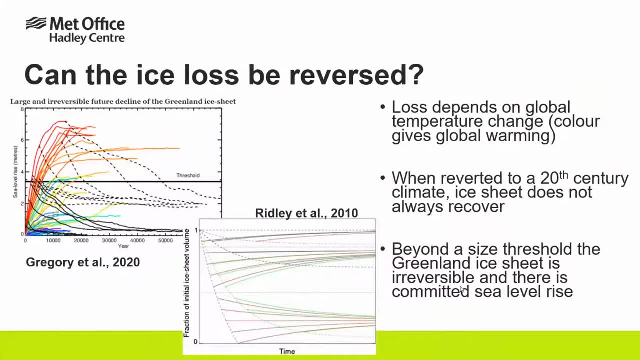 it's, you know it's, it's perhaps could be viewed as a slightly more upper bound estimate. And the final thing I just wanted to touch on is the question about whether ice loss can be reversed from Greenland, And so there's a an older paper here by Jeff Ridley, one of my colleagues at the 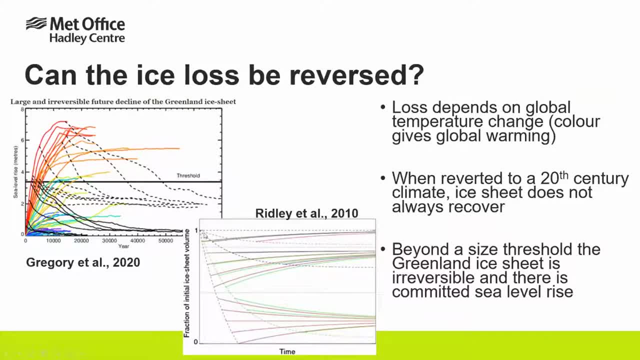 Hadley Centre And in this paper they looked at, at, at the ice loss and then trying to recover it. and so you see here that as time continues, this is the ice loss, and if they stop at a particular point, will the ice recover or not. 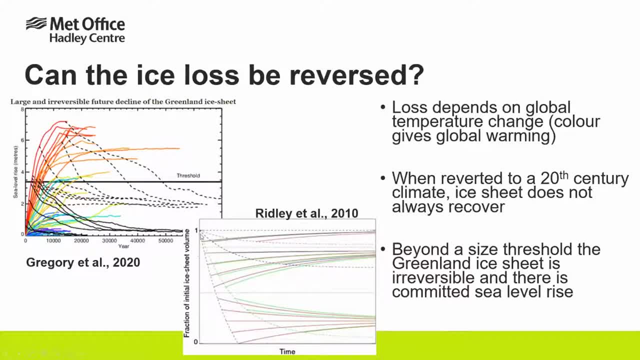 so this is the fraction of the initial ice sheet volume. so you can see that you get to a point, and before this point you can get back to a recovery of the ice sheet. but once you've gone past the threshold you seem no longer to be able to get some back to your original ice sheet volume. 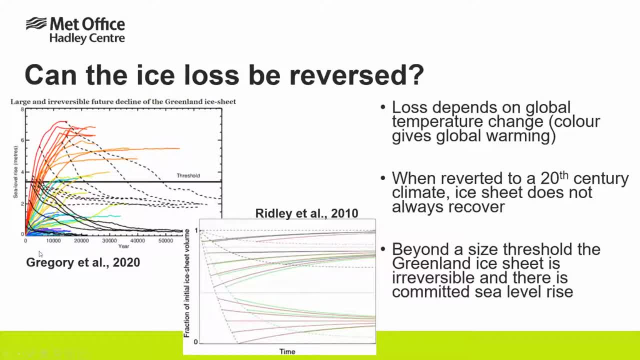 and this is here's another paper by Jonathan Gregory, also a colleague at the Met Office, and in this paper they ran the ice sheet model under different temperatures. so the warmer temperatures are the darker colours and then they, at the points where it moves to black. you reset to the 20th century climate and you can see that in some of these, the earlier ones, 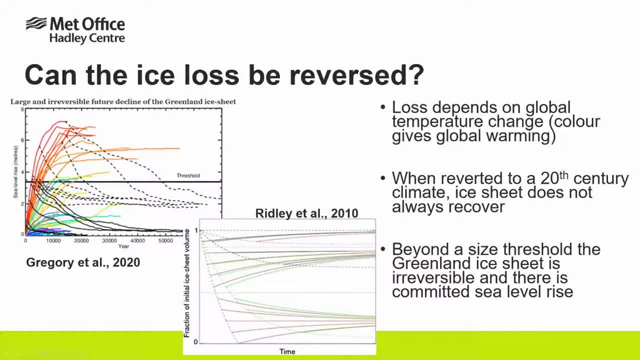 before it's past this threshold line, you've lost ice, but then the ice will then regrow. this is the ice regrown because it's the effect on sea level. this is shown as: whereas once you've passed this threshold and you've gone back to the 20th century climate, you can see that the ice 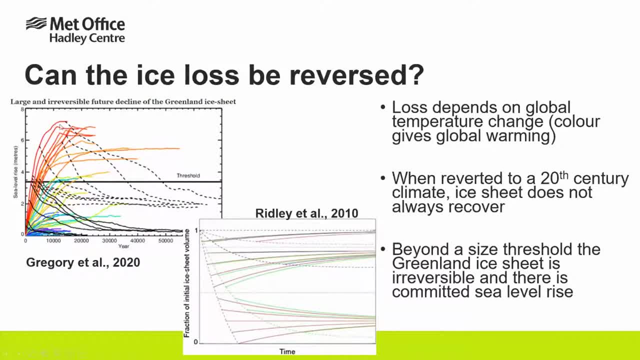 sheet can regrow and you've contributed, say you know, six or seven meters or past three and a half meters, in this case to sea level. the ice sheet can regrow, but not back to its original level, so it seems to reach some kind of maximum level where it's committed to about two meters of sea level. 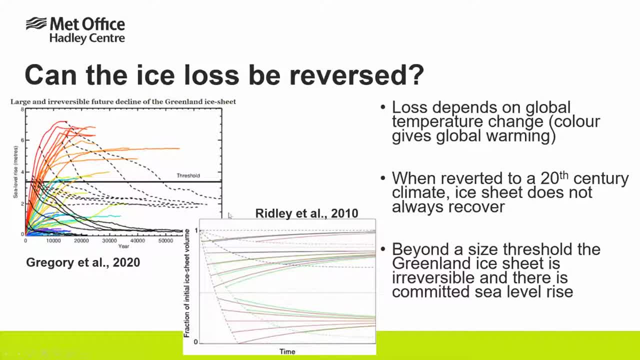 already so. in both cases, there appears to be a sign of this threshold, and that's true in other papers as well. So I'm going to move on to the next slide. So I'm going to move on to the next slide. So I'm going to move on to the next slide. 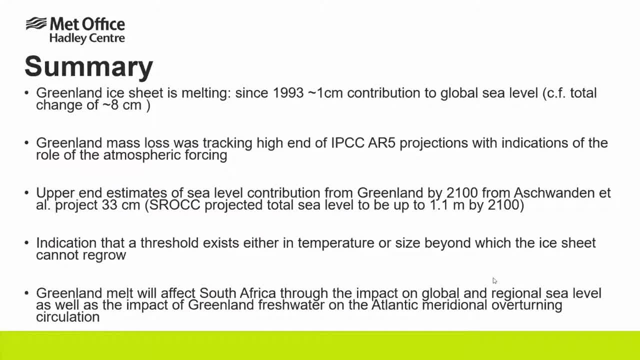 So really you know. to summarize, the Greenland ice sheet is melting, so since 1993 it's contributed about a centimeter to global sea level. compared for the total change, The Greenland mass loss was tracking the high end of the IPCC AR5 projections with indications of 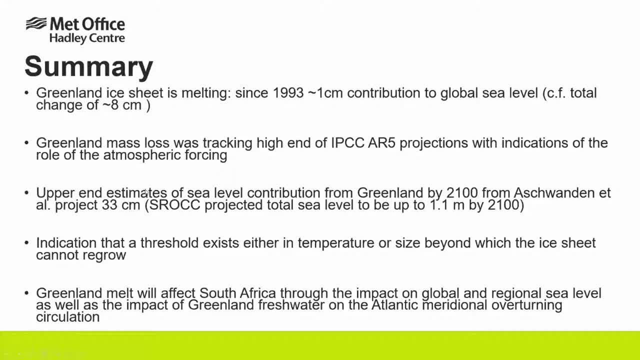 that there was a role of the atmospheric forcing. There are, there will be, estimates from ISMIP6 in AR6, but you know, I'm just saying here what the upper end is. so you know an upper end estimate could be 33 centimeters, although we know that's a very highly sensitive model. so you know, you can caveat that. 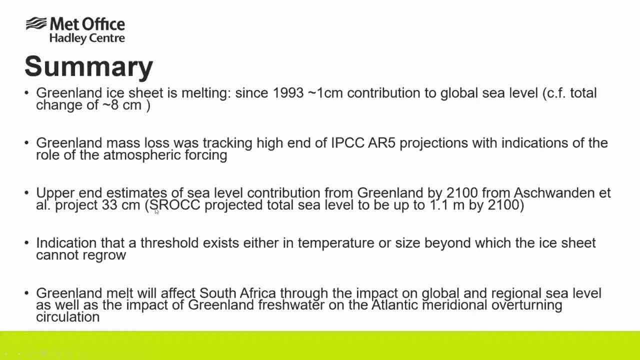 SROC suggested- I think it was closer to 20 centimeters For the Greenland ice sheet for the high end, and that's out of a total sea level of up to about just over a meter by 2100.. There's definitely indication that threshold exists, either in temperature or size, beyond which the ice sheet can't regrow. 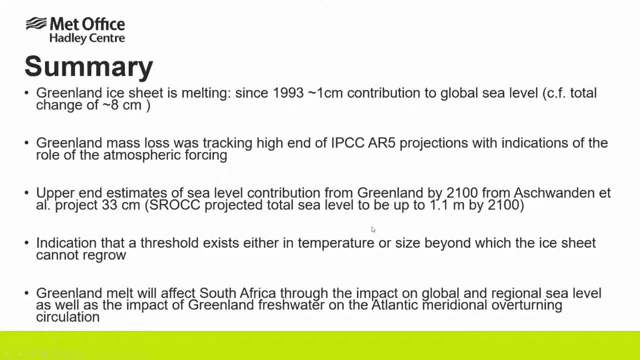 And I talked at the beginning of the talk about how it might affect South Africa through the impact on the global and regional sea level and the freshwater effect on the meridional overturning circulation. So it's a real smart pack And very happy to take any questions. 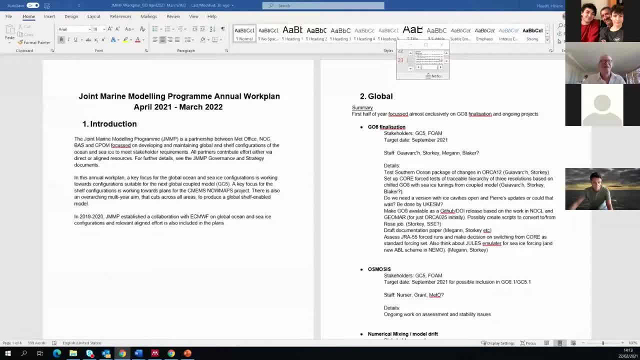 Thanks very much, Eileen, Thanks for that was a really, really interesting and full provoking set of ideas around us And it's it's, And we've got a number of questions. I just want to ask, Neville, what are the time constraints on the? 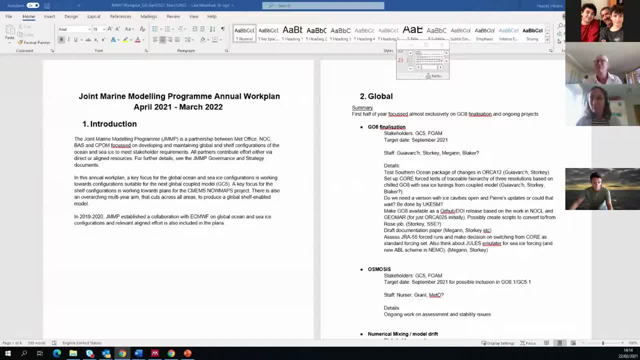 questions. Thanks, Pedro. Well, we are waiting for Antje Bottius to join us. I don't see her yet online, so we can at least continue until she does join us and perhaps a bit beyond that, And if we do have questions left over, I will undertake to record a question and answer session. 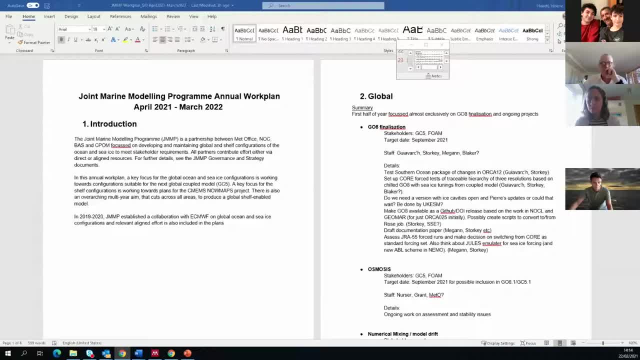 with Helene when and if that suits her. But in the meantime I'll progress to some of these questions. Would you like to read them, Pedro, or do you want to read them? So I've got them, thanks, Okay, great. So I think that just generally one of the sort of take-home, high-level take-home. 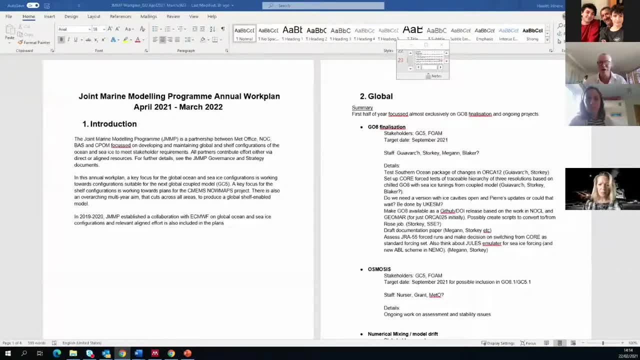 messages here is that we really do have a lot of questions, And I think that's one of the things that we have to pay attention: A- to the cryosphere and perhaps pay more attention to it from as a sort of science community in this part of the world. But B- we have to pay attention to: 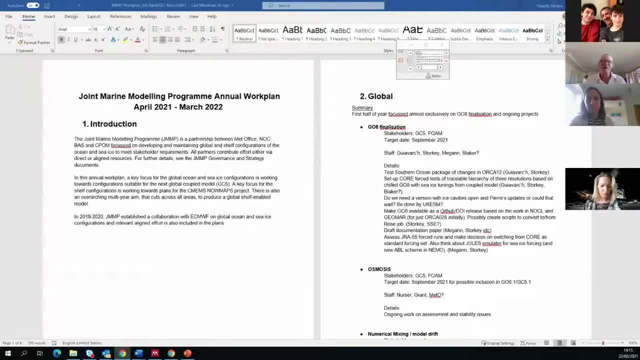 what is being done in the Arctic around these questions, around the cryosphere? just because those signals propagate to our hemisphere either through the ocean or through the atmosphere. So, and how it does, that is something that we need to have a clearer understanding and a capacity. 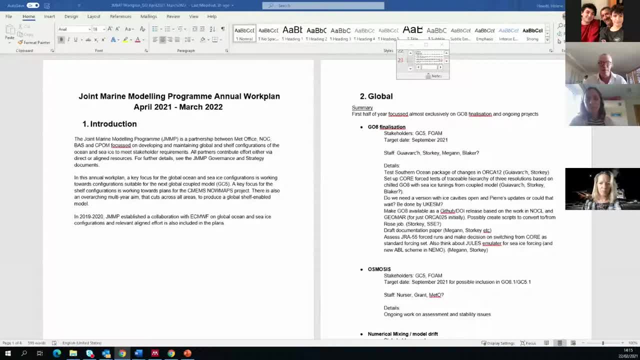 to project those. So, Helene, so we've got a number of questions here and there are two which are really part of the same thought, And the question is really: how is ice loss recorded, How do you determine ice loss And how do you determine ice loss And how do you determine ice loss? 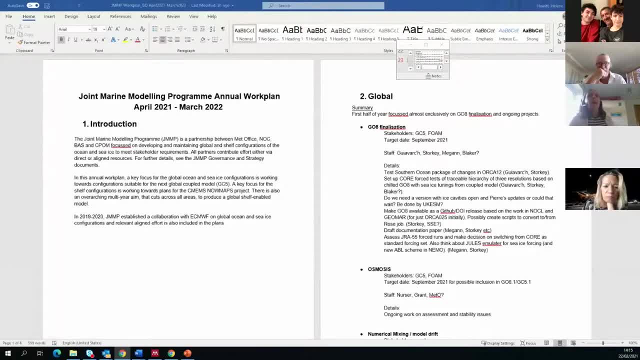 There's various different ways, but the obvious way is from the satellite altimetry. I mean, you can see that they can measure the height of the elevation of the ice sheet. So that's one way And you know you can. it's the different methods. 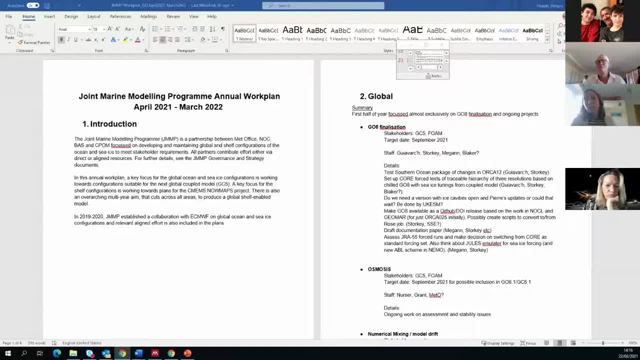 They use in the, in the Imbi data. So you know, that's, that's one way from satellites. Yeah, So yeah, read the details in the Imbi paper. But that is, that is the obvious way. 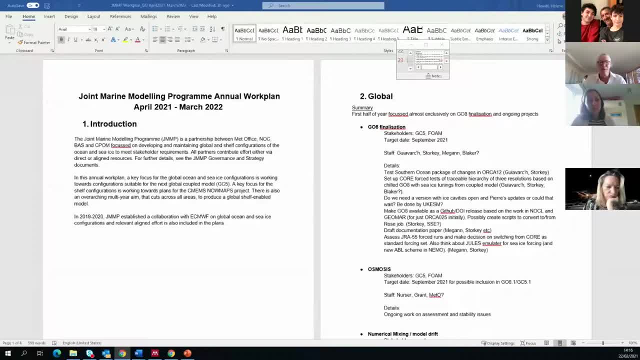 So, thanks, Thanks. So I've got a question associated with that. is that, in terms of sea level, the contributions that the ice sheets, the ice shells, make to sea level rise. how do you tell the northern hemisphere contribution from the southern hemisphere contribution? 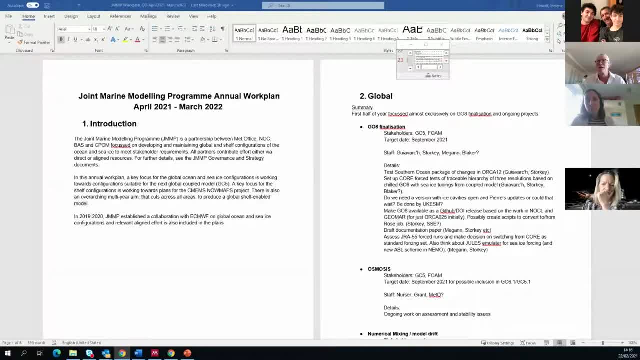 Is it just by measuring the loss through that same way And is looking at the loss from satellite observations? Yes, Yeah, Okay, Yes. So there's another question here, which is that you've really focused on um, although you 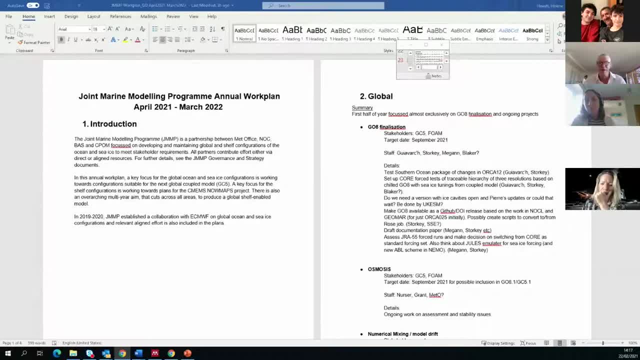 show a number of different scenarios, a sort of a high, medium and low mitigation. there was a sort of a this question saying, well, you were focusing largely on the results from rcp 8.5, but that that seems like an unlikely scenario, um is, is there a reason for that? yes, well, i'm i'm not on the 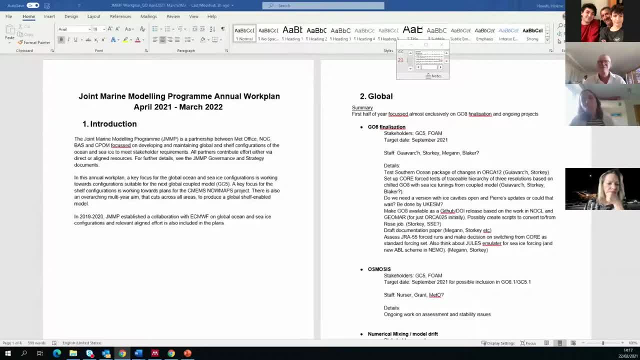 ismip 6 committee. so i i wouldn't know. i don't know exactly why they they focused on rcp 8.5 obviously. i guess one reason is there's a long lead time on these experiments and this discussion about rcp 8.5 being unlikely, probably the ismip 6 projections, probably. 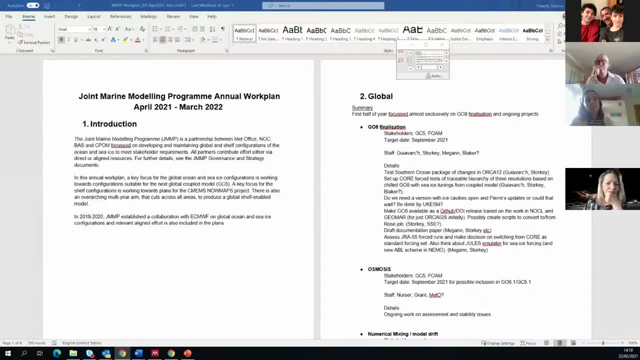 predated. that is one thing. another is: i you know we are limited in the number of experiments we can do, and and so, um, rcp 8.5 will give you the biggest signal and be able to understand better the sensitivity between the different forcings. um so, um, i definitely would take that. 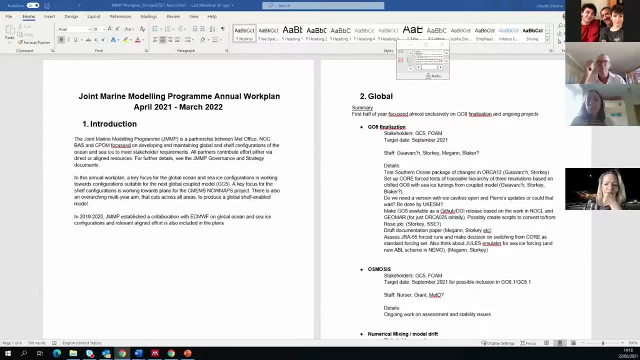 point and i'll um, i'll, i'll feed that. i'll feed that back to sophie and others and ask them what they're thinking for um for an ismip follow-on. great um. there was a question about um. are we, are we in a period in which glaciers are forming more slowly, or are they melting faster? 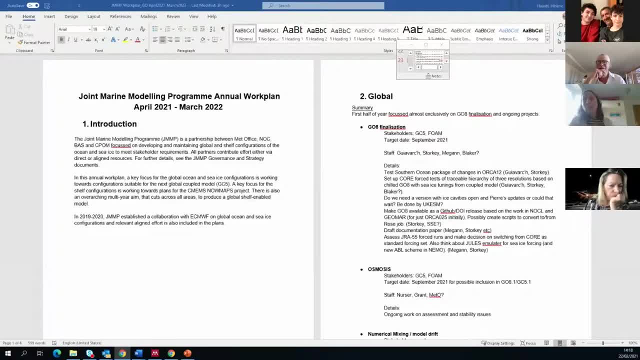 um, oh, that's a good question, isn't it? yeah, well, i think that i think they're melting faster, basically, at the moment, i mean that's not true of all glaciers. i mean glaciers regionally is a very complicated, complicated, uh topic. so i don't think you can say: 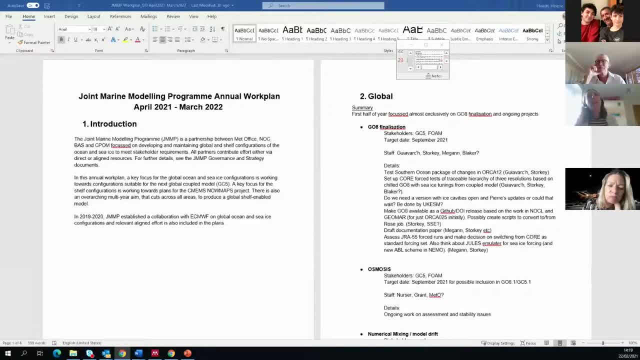 something. um, you know, i- i think you would say globally- glaciers, um, you know, both mountain glaciers and the peripheral glaciers are melting, but there can be, you know, very strong regional differences where some glaciers will buck the trend if you like. so, uh, you have to, you have to. 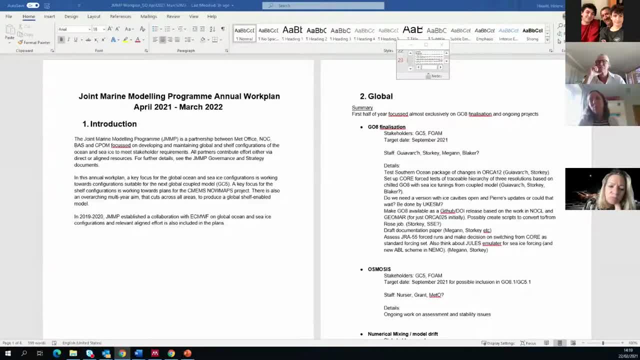 look at individual ones, and you have to some, you know, make the global sum, i think as well. so here's another one which is kind of along that line as well. um so so how did the ice sheets grow in the first place if they need to be beyond that threshold that you were talking about? 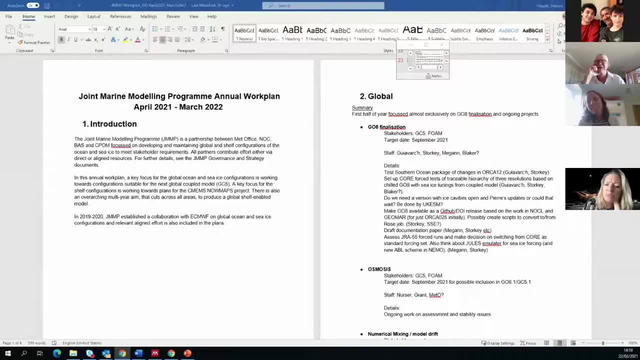 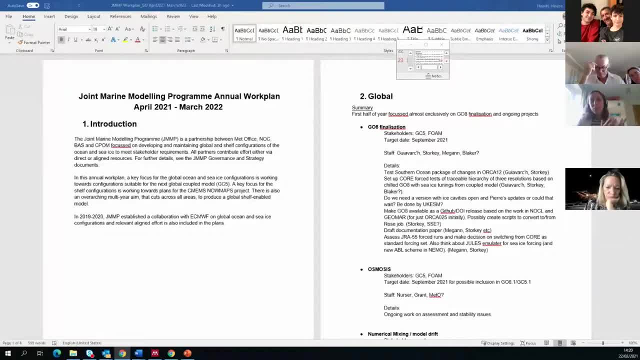 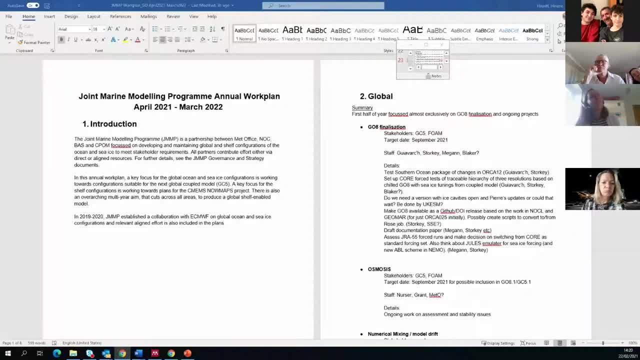 again, people ask questions and it's things you hadn't really thought about. so, um, i i guess it gets cold enough that it that it gets, that it gets beyond that threshold. so i i have um one additional question for you. so so ice sheets, ice shelves and sea ice, i kind of 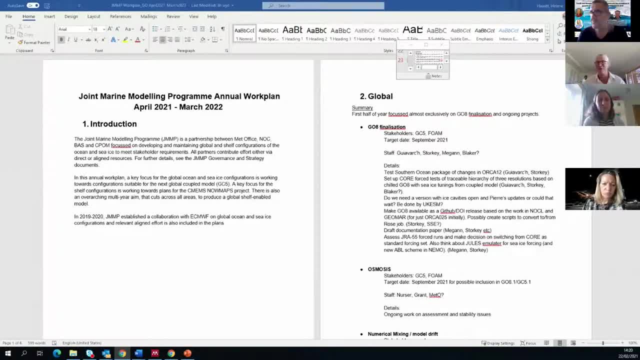 think about them as in this sort of a continuum. i probably shouldn't think about them as a continuum, but anyway, that's uh um. is there a feedback between them, you know? in other words, do changes in the sea ice alter the dynamics of the ice shelves and the? um and the? 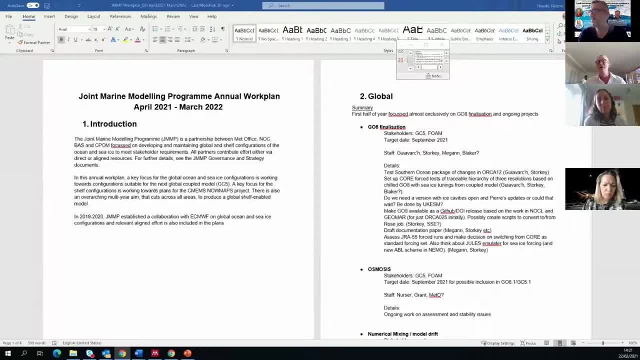 ice sheets and vice versa. and you know, and can the ice shelves and ice sheets influence the dynamics of the sea? ice, yeah, i mean, i think people talk about this more in the southern hemisphere, around antarctica. uh, you know, it's, it's perhaps. yeah, i think it's probably possibly. 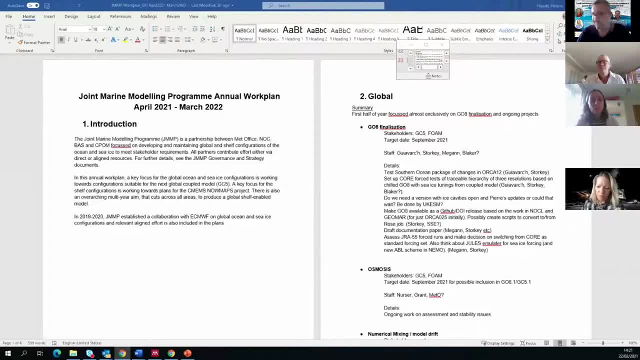 less true in greenland, but in antarctica there's a lot of work on looking at the interactions of the sea ice and how much that buttresses the ice shells and stops the outflow from the from the ice sheet. so there it is believed there's a. you know there is an interaction between the two and 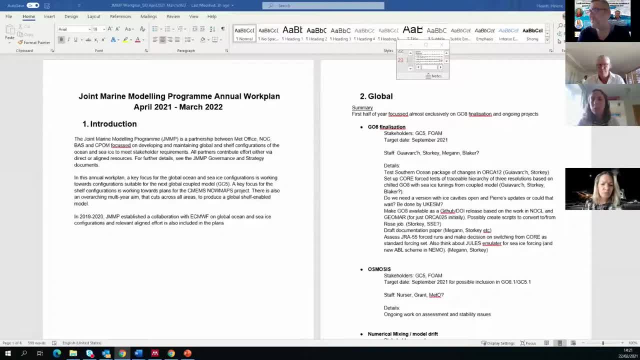 that is a that is definitely an active topic of research. right, interrupt by saying there are maybe some other questions and, helene, i will come back to you about recording and a quick exchange with you on some of the questions and answers that might remain. um, thank you, yeah. 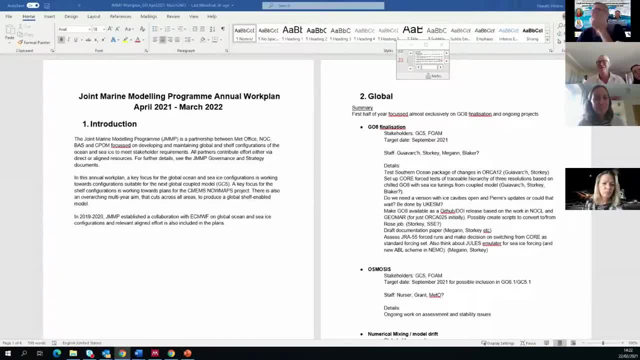 great, you're welcome. thank you very much, helene. that that was great. thank you very much. okay, so i see that anchi brisius has joined us, and a warm welcome to you, anchi and um. and without further ado, let me introduce you and um open the floor for you. so. 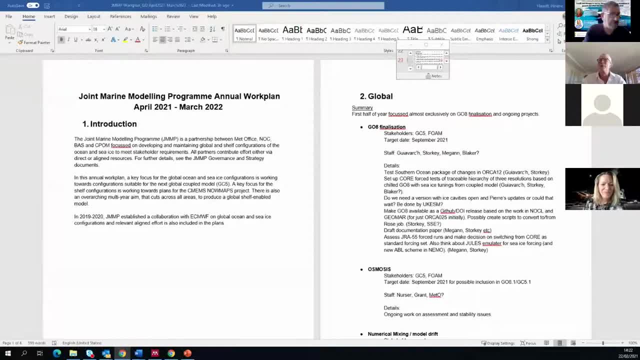 and she's our second distinguished guest today and, um, as i mentioned earlier, she comes at this uh cryosphere, uh issue from a completely different perspective, but and in fact, um, she's our second distinguished guest today and, um, as i mentioned earlier, she comes at this uh cryosphere. 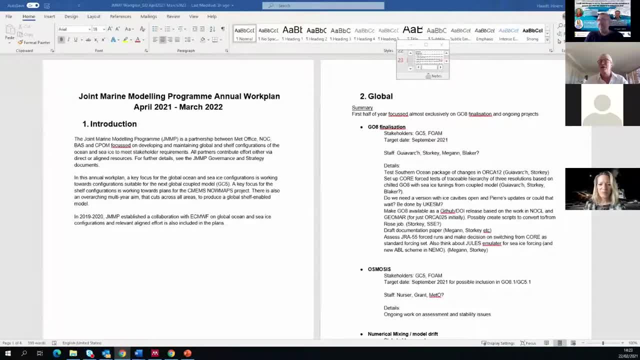 from the perspective of um, the ecology and and the processes around the microbiological communities associated with the cryosphere. of course she also thinks much more broadly than that about the so large-scale implications, et cetera. but uh, and she's a microbiologist with a sort of ocean. 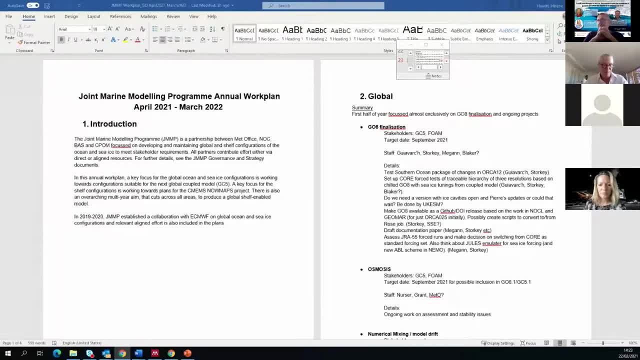 focus more broadly. she's probably better, has a sort of lot of interest in the questions that are asked to her. but sorry, i'm afraid i just wanted to add that there's a lot of work on a very broad overview of what's on the us and the sponge and ocean. but i think that has to do with the 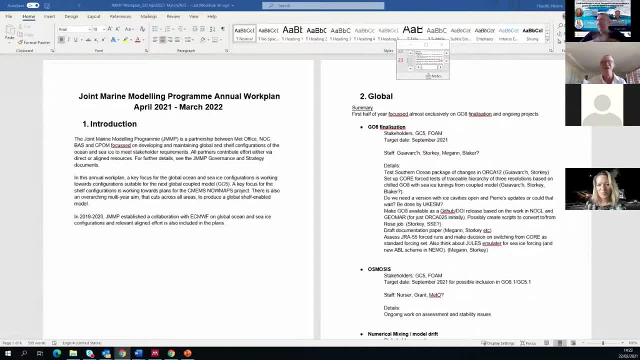 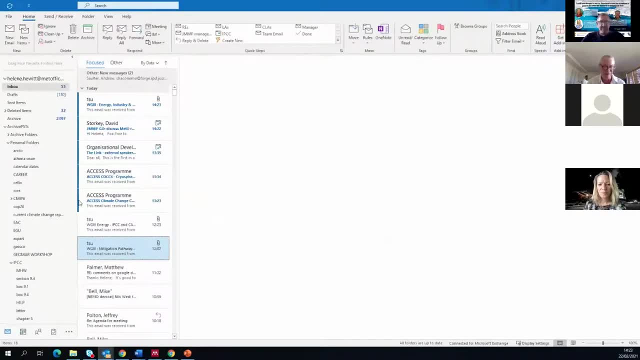 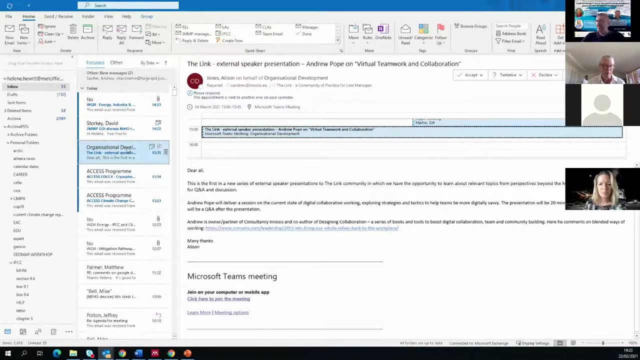 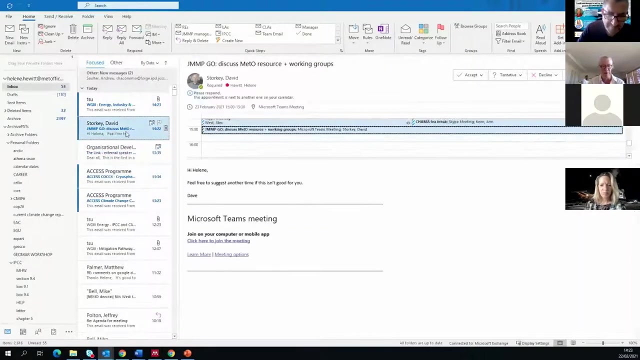 has a sort of a longer history in deep ocean microbiology and more recently is taking an interest in the cryosphere dimension of the microbiological biomes. So Anqi is a professor of geomicrobiology at University of Bremen in association with the Max Planck Institute. 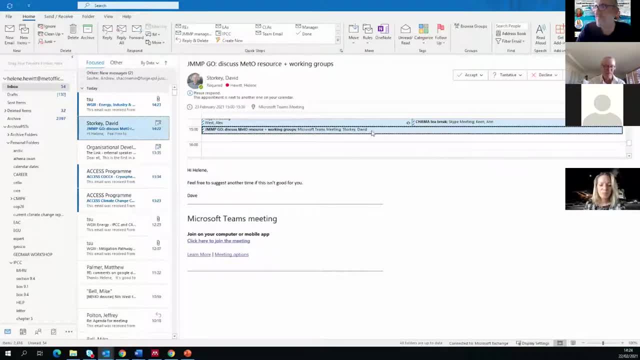 She's also the director of what's generally called AVI- it's the Alfred Wegener Institute, which is the premier German center for polar research, and a more recent association with GO Meyer in Kiel, with an arctic focus around the ecological effects of warming and sea ice melting. 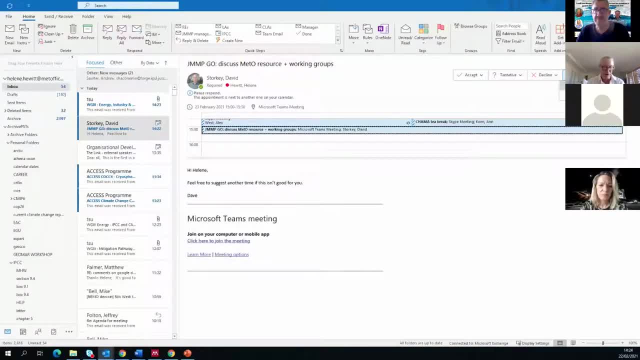 She has earned an enormous amount of money in her early 20s as a professor at thefuels. number of awards, and I'm not going to list them all as simply to say that a good metric of that is that for the past 12 years she's won at least one international or national awards. 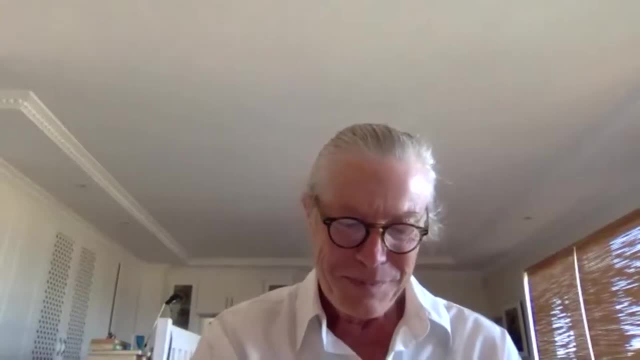 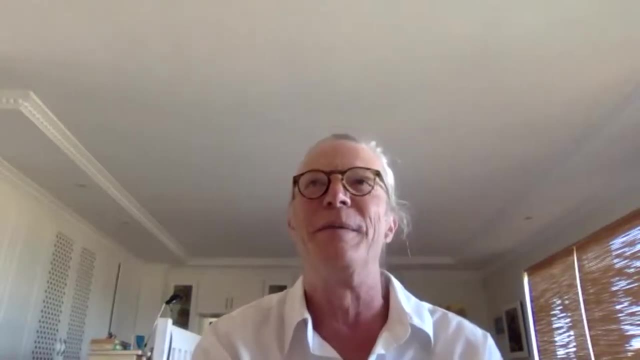 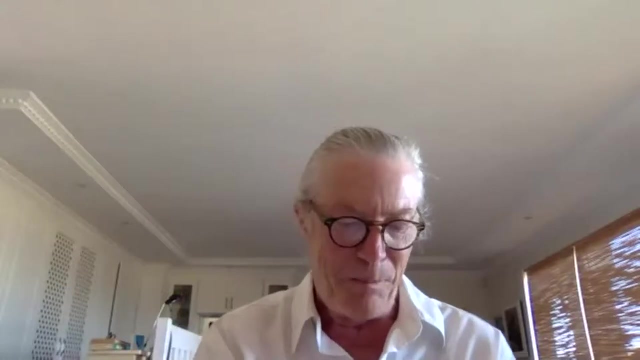 so, but most recently, and she was also the co-lead uh scientist for the mosaic experiment and that's, I think, is going to be really the focus of her engagement with us today- and I mean, the mosaic experiment was really an audacious idea, that, and it was audacious both. 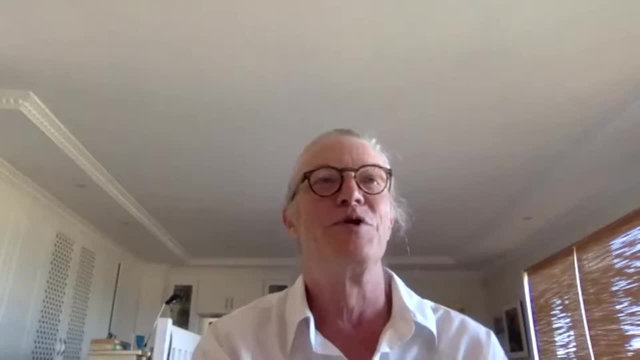 intellectually and logistically, and I'm sure we'll hear a little bit about it and it's it's actually gives it gives one a sense of at what scale do we need to plan our understanding of these processes, when you're thinking about the links that really explain the variability and 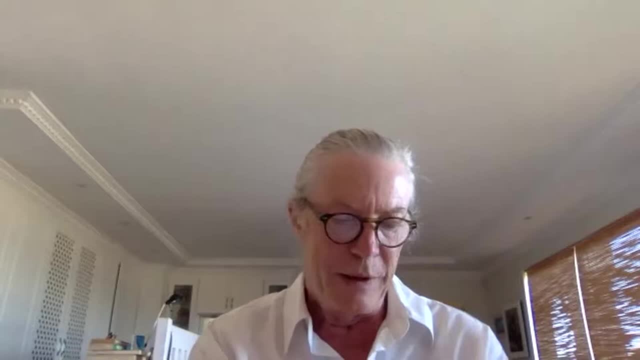 so these systems are going through and the mosaic experiment was really a seasonal cycle experiment and uh, and it provided uh unique, uh synchronicity in observations from physics to ecosystem. I think that was certainly one of the things that we you know. that was really fascinating about it. so the topic of her presentation is into the ice, the coupling. 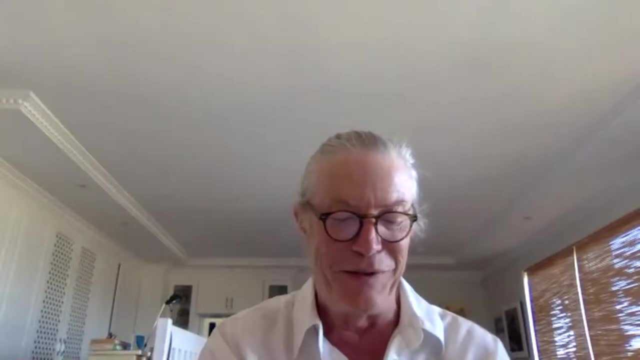 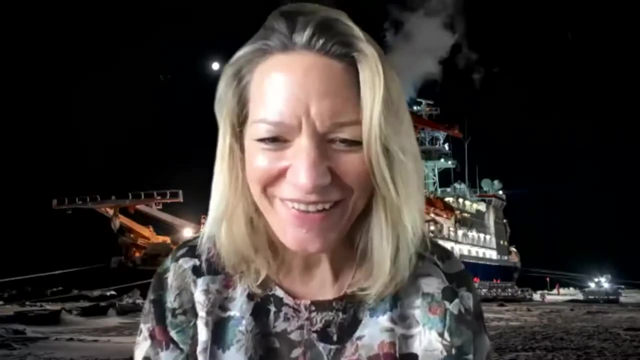 of climate, sea, ice ecosystem states and the mosaic experiment was really a seasonal cycle experiment at the time of the mosaic experiment. so we are going to get into a little bit more about that in just a few minutes and we'll talk a little bit more about the mosaic experiment. 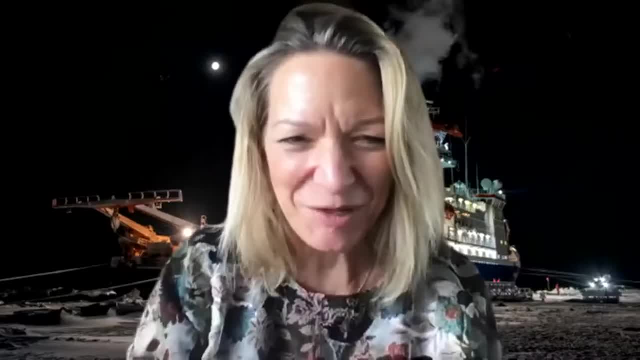 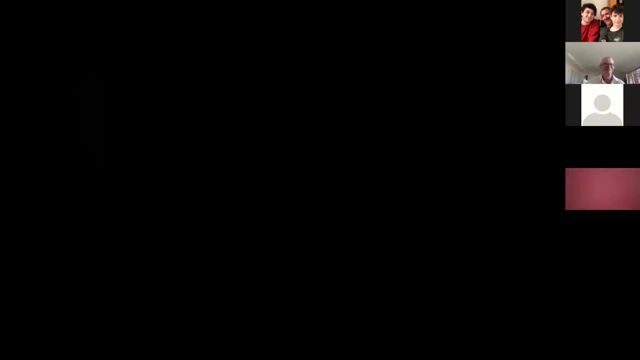 and how it relates to the climate that's in the Arctic. Anqi, over to you. Thank you very much and hello to everyone here. I'm very happy to be with you and to discuss a little bit of everything that Pedro has just mentioned, and still aiming for finishing the job in time. so let's start. I hope you will see in a moment the screen. 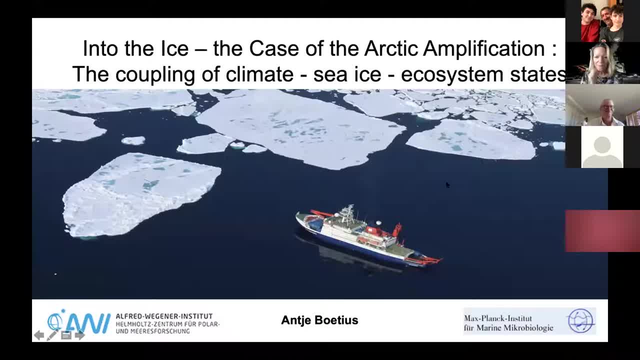 I hope you will see in a moment. the screen is that good, thank you okay. so, um, i would like to discuss a bit more about the christian, christian changes and the relevance for life on earth, including us humans, and, um, i'm also happy to say a few words about mosaic, our latest large mission, but also in general, as beto mentioned. 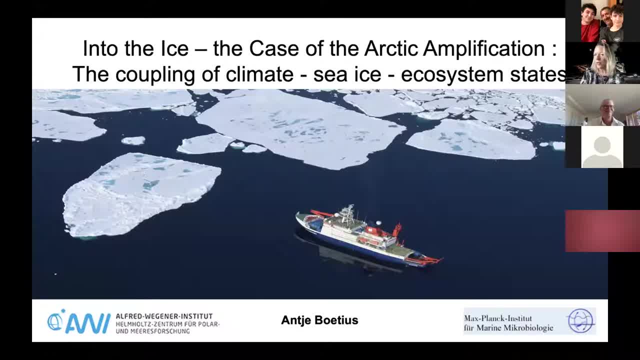 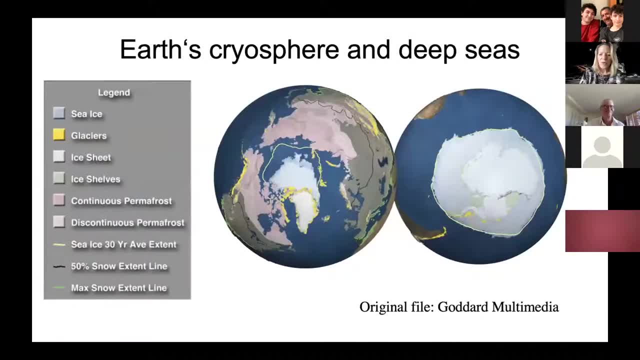 this whole question of how important is it to observe, to study, to analyze processes and their connection to our human behavior. so what i'm so fascinated with- or always was since i'm a kid- is actually: what does the cryosphere and the deep oceans mean for planet earth? 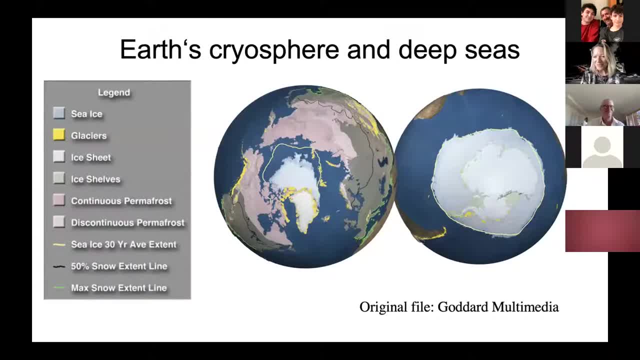 and and life on earth, and so i love this picture, this depiction of earth, when you cut it in half and you see, on the one hand, the arctic, on the other hand, the antarctic, and you see they are really different systems, though they represent our polar regions. the arctic is basically a deep ocean, an ocean that is linked to the 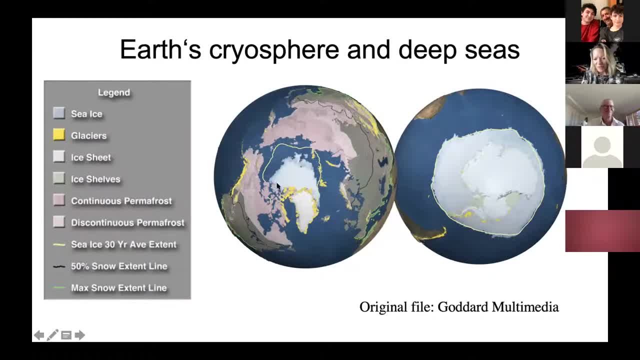 atlantic and also to the pacific, and is covered with sea ice. has a continent covered with ice masses- greenland- but much smaller ice masses in total than antarctica. and the arctic. has this huge area of frozen ground called permafrost that you see here in pinkish. that's an area where 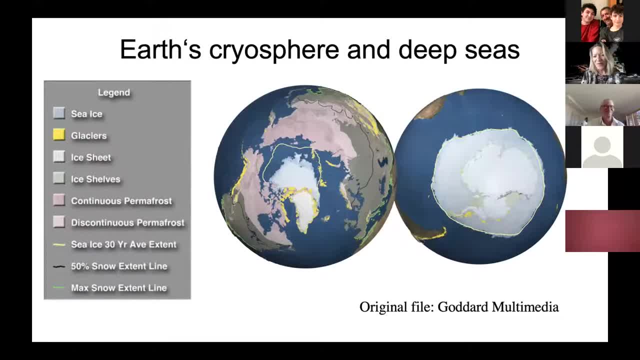 in the old days, so to say in the holocene, earth was permanently frozen and covered by snow. and when you look to the antarctic then you see it's a continent. here in the south pole is in the middle of a mountain range. basically you have two to three kilometers ice, ice mass that has built up as 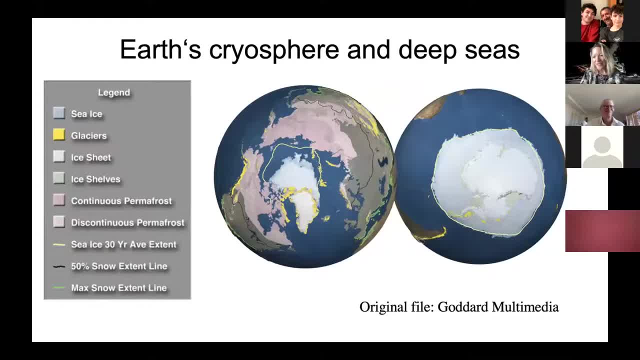 you've just discussed before me. and then you have to see ice around the continent and arctica and you have to see the ocean, which is this vast, huge deep ocean that connects all oceans together with the circumpolar current. so two very, very different systems and one of the most interesting questions. 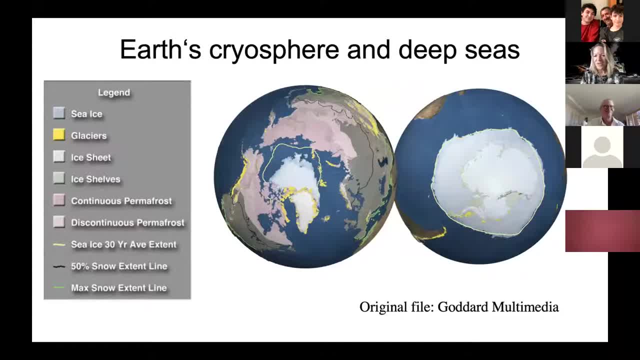 of of the geosphere and the history of earth is really, how did these two polar regions actually function together in shielding the earth from warming, warming by their, by their whiteness? so today we still struggle to answer the lead and lag functions of both polar regions, like when earth 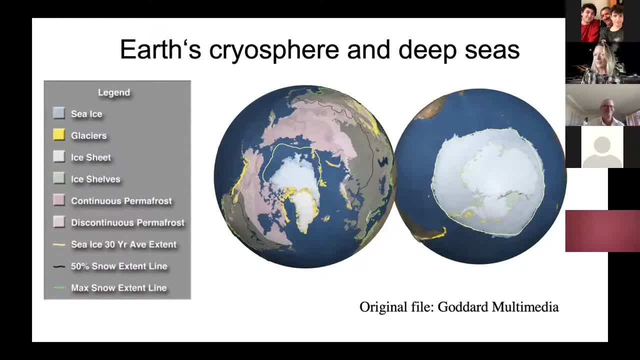 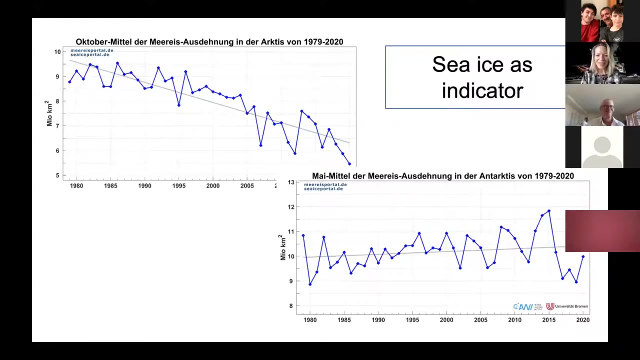 got closer to sun and started warming, how did these two polar regions respond? on which time scales? those are all very important questions, but the the difference between the the both has always also been a struggle for the public to understand. is there really global change? is there global warming? so here i love the sea ice indicators. here you see again from our sea ice. 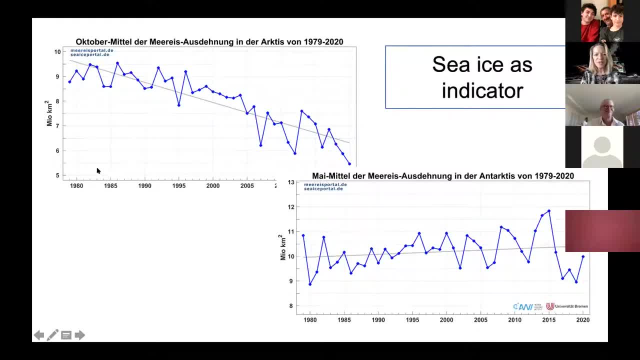 portal that we host at avi together with the university of bremen, just the sea ice in the arctic from 79 to 2020, and that's the october mean and uh, before, like, let's say, the the last 20 years, we've always used the september mean because that was the time of the sea ice. 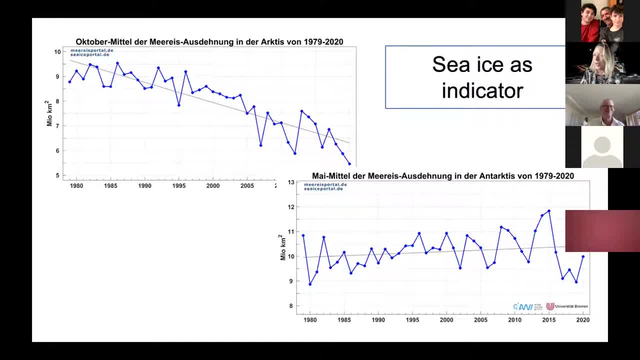 minimum in the arctic, but now it's october actually, so it's delayed to autumn. and there you see what, what is so striking to understand? that the sea ice is shrinking with a very clear trend of, meanwhile, 13 percent per decade, and you can see that in the last few years there have been these huge 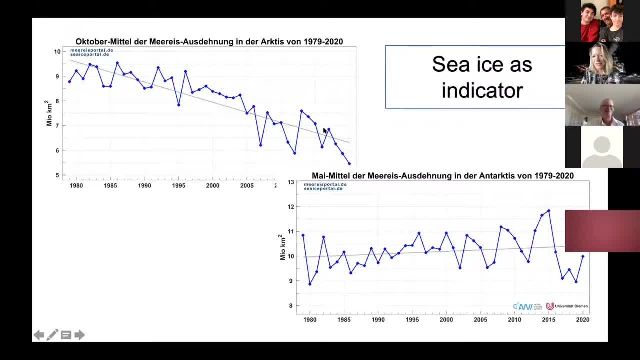 for example, 2012, but also later now this year, there have been really a rapid decline again and when you look at the trend and the current trend, it might well be that in the next five years we will have to adjust the statistic trend for sea ice loss. then below, here you see an arctica, the 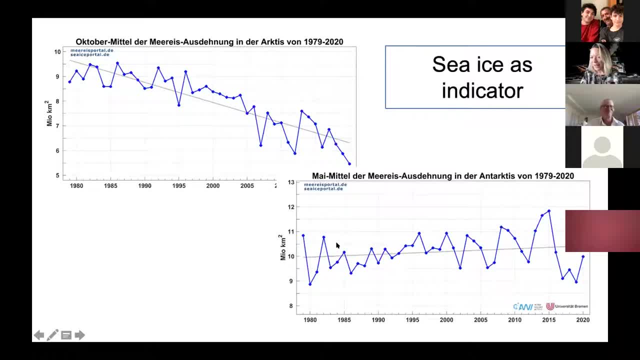 sea, ice of an arctica, and this time it's the may, so it's the opposite. six months, uh, reflection of the season, and you get the impression that cs is actually increasing. but it has a huge dynamic in the in the recent years, and for some years it has been also. 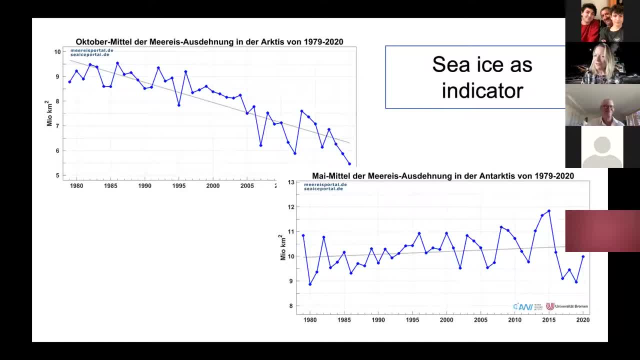 shrinking a little bit, then now inclining again. but one of the big struggles with the public and with the media to make people understand that global change is real has always been this argument: how can you say that cs is shrinking when it's actually growing in antarctica? two: 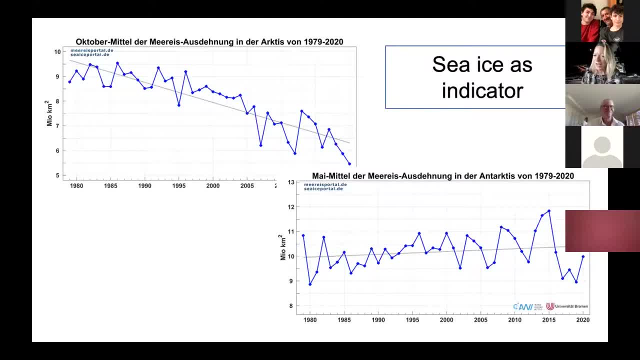 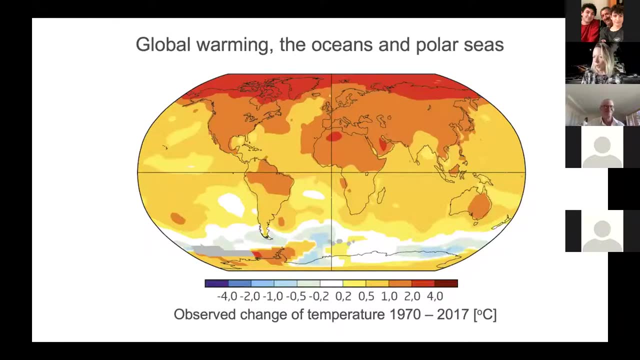 very different systems. we need to understand both of them. but today i'm going to focus on the arctic, which has this enormous amplification of sea ice loss and warming. so why they are so different we can explain scientifically. it's not just one factor, it's many factors all together. but when 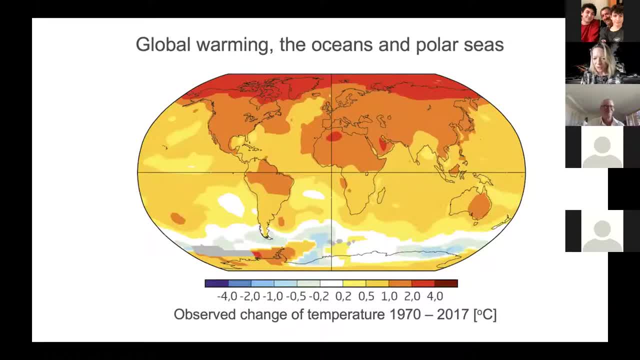 you see the global distribution of temperature change between the the 70s to today. you see what we mean by arctic amplification. the north is warming a lot and very rapidly. in an arctica a, we've just said there is this: the ice mass on the continent. so when you measure ground, 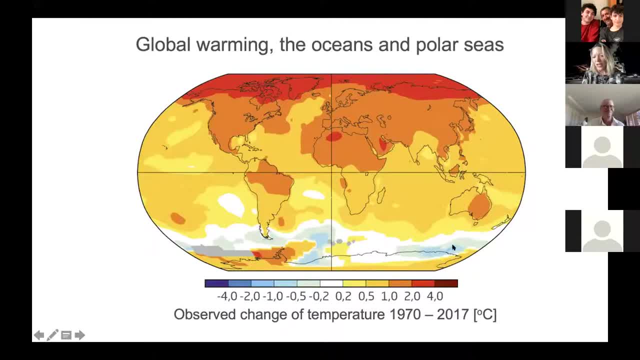 temperature is already very high and it's very cold. plus you have the circumpolar current that actually protects the ice masses and the sea ice. so it's the same, or it's sometimes even a bit colder in some areas, but there are entire areas of an arctica where sea ice is also shrinking. 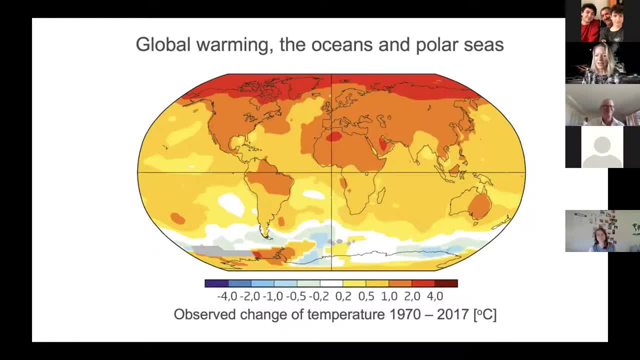 like where we work, in antarctica, parts of the weddell sea, we see that, but in western and arctica so it is so that we really have to understand there is a regional, very regional difference that we have to look at. in the arctic, however, sea ice is shrinking everywhere. 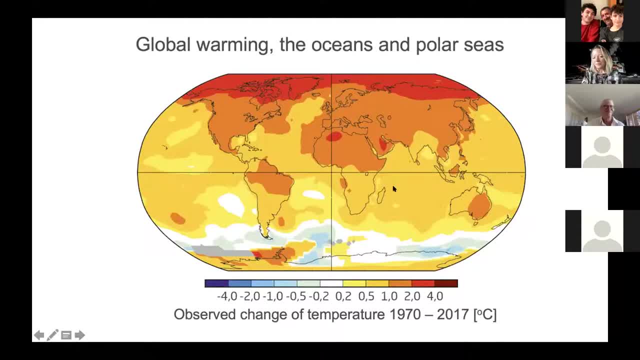 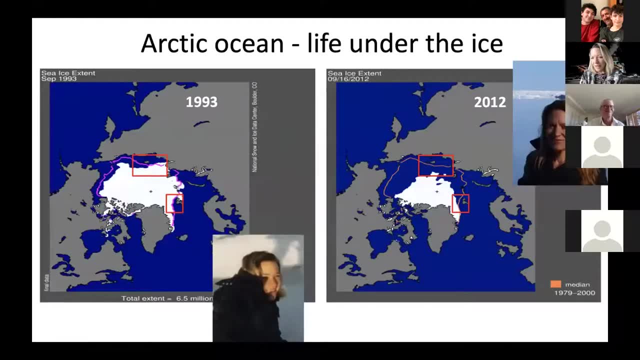 because of this very rapid warming. um- and i come back to this- temperature differences in a moment. myself, i, as a deep sea researcher and geomicrobiologist, as i was introduced, i always thought much more about being able to look under the ice, discovering all kinds of new 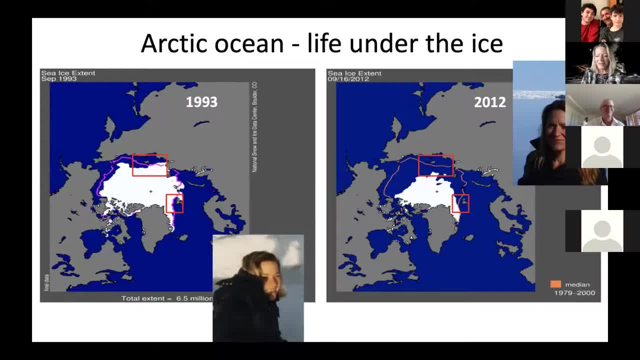 life forms that no one knows about. when, by chance, uh, after doing my phd in the arctic in 93, going with the sea ice breaker, polar stern to the siberian seas and the seas around spitzbergen that were fully ice covered with multi-year, 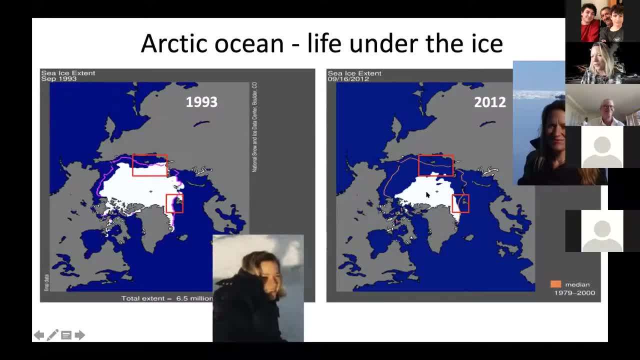 thick sea ice at the time, and then coming back in 2012, where i was expedition leader, and being there in the summer where the sea ice melted at the most dramatic rate we know since the onset of satellite observations, and so that has really changed the way i looked at sea ice, because i was there and i literally saw with my own eyes and all. 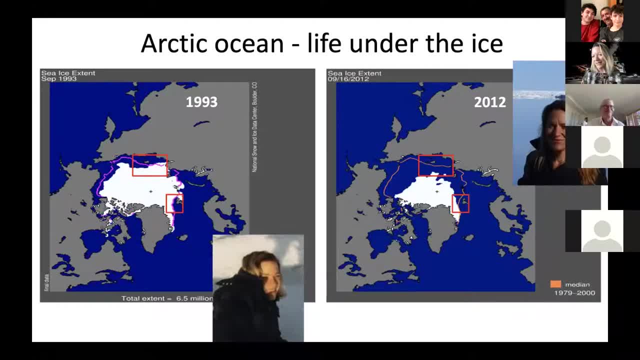 the expedition members too, what it actually means when sea ice is melting so fast and all the life in the ice and on the ice loses their habitat. it's, it's a striking process. so one of our senior polar researchers, marcus rex. he's a very calm physicist, but when he saw that 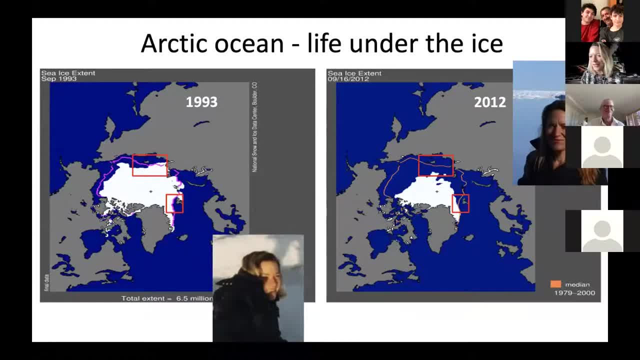 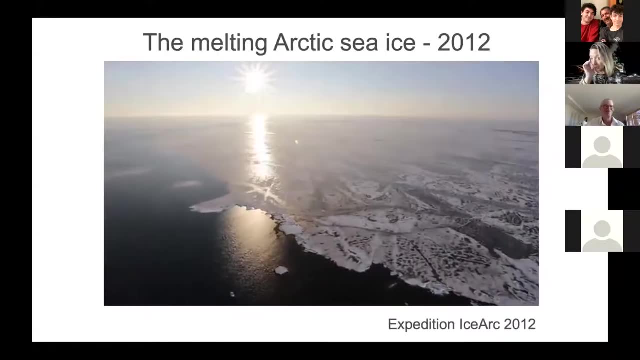 rapid ice shrinking, he said. he wrote to the media and said to the media: i saw when the ice was dying. of course ice is not dying, but still the impression of that rapid melt is just amazing when you see it with your own eyes. here you see a glimpse of what i've just talked about. 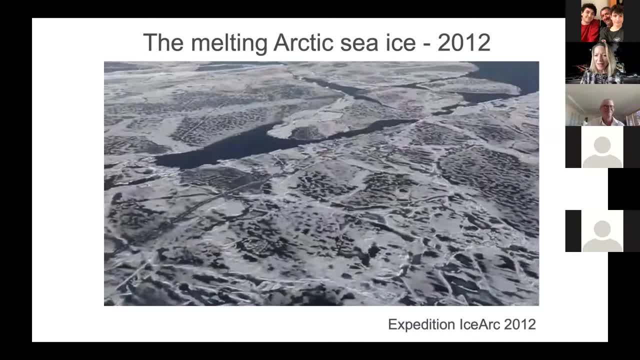 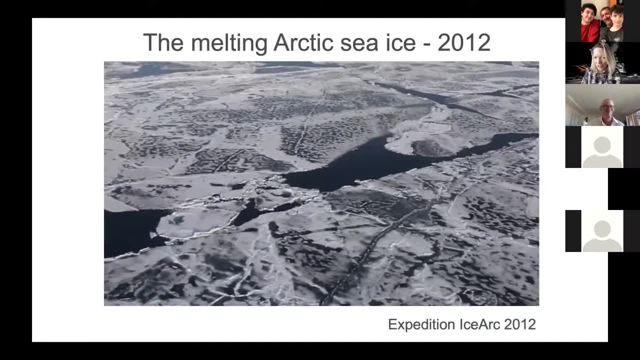 i don't know how many of you have been to the ice, have seen sea ice, but these years, these summers, this is what the north pole looks like, and so, even if you have never seen sea ice or walked on it, when you look at this ice surface here, when you see how the icebreaker is now steaming through, 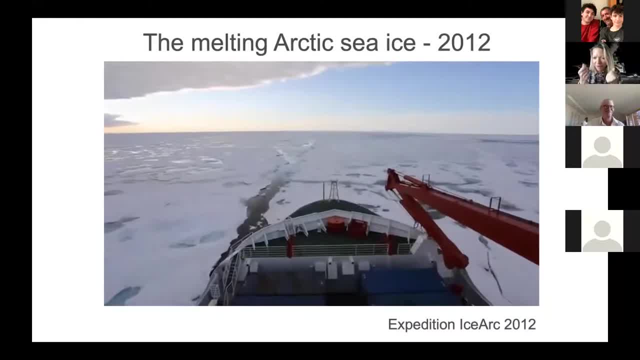 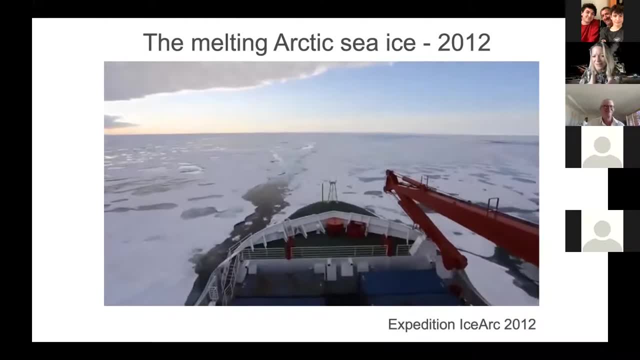 the ice as if it was spiking. the ice is now steaming through the ice as if it was spiking. so just a very porous, thin sea ice- less than a meter left in summertime. everything covered with melt ponds, huge cracks and leads to which the ships can go. 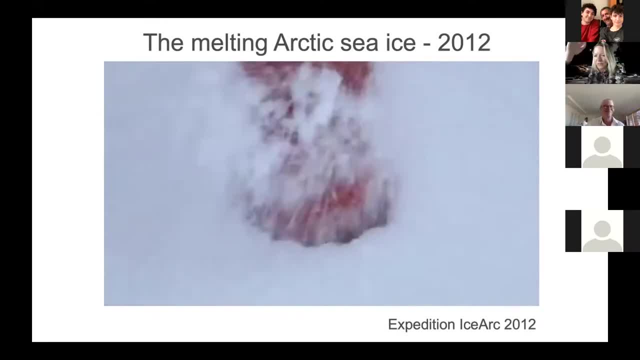 and in fact also drilling an ice core just takes like one hand now and in a few centimeters. basically, you see the warming ocean waters coming up through the ice, melting it from below and above. then you understand what it means that ice is rapidly melting from warming of the atmosphere. 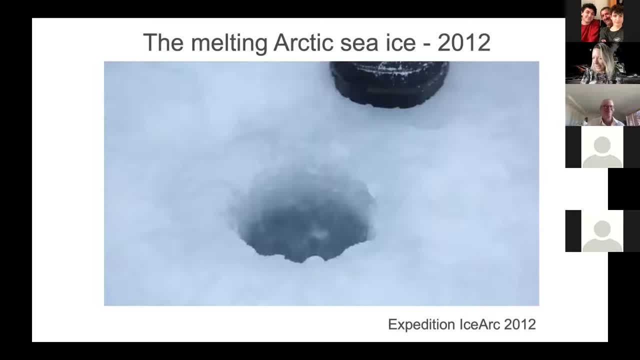 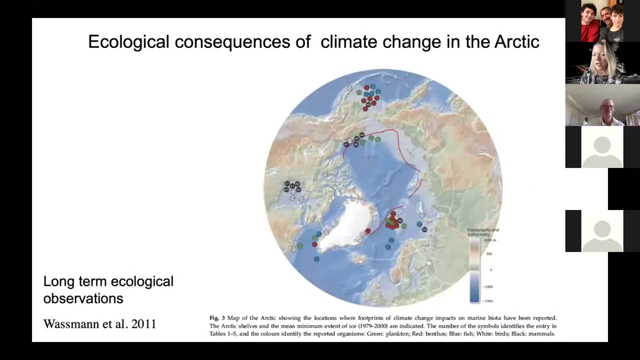 and warming of the ocean. so this state, the antarctic, has not reached yet. but that's the arctic state and from earth history we know it can be times when the arctic looks like that. eventually it will get to the antarctic, with the arctic which is so different because it is surrounded by pan-arctic states, in fact. 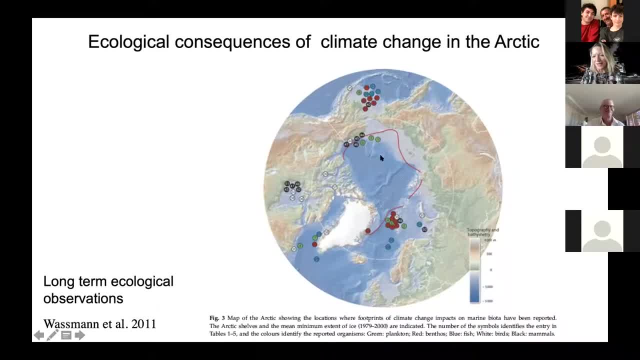 civilization is relatively near to the arctic. the arctic is a giant shelf sea and has has a deep sea in the middle. basically, the arctic is a giant shelf sea and has has a deep sea in the middle, basically. still we fail in giving it enough attention, all of that change that i've just described merely. 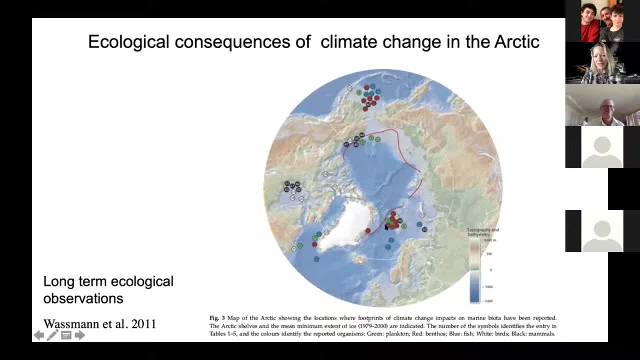 from the perspective of sea ice. this map that you see here, in red was, is the area where we have sea ice or had sea ice in the past 100 years. the dots that you see are those places where we have observations, long-term observations of ecological parameters, sometimes only phytoplankton. 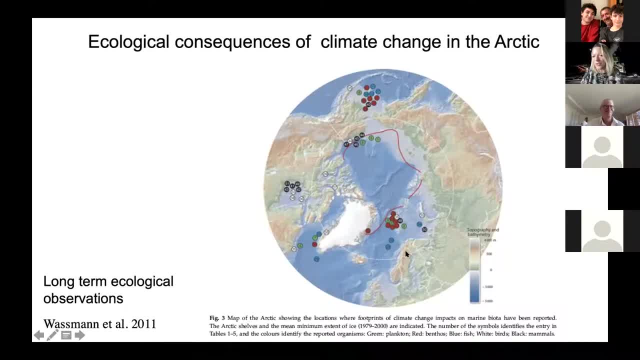 sometimes a bit more. but you see our problem as human civilization: we have barely enough mountain of land to achieve this sort of camellia thing. and then you also have to make it the problem where we have very little land, so basically it's not even sustainable all of the time. you can have a lot of more land. 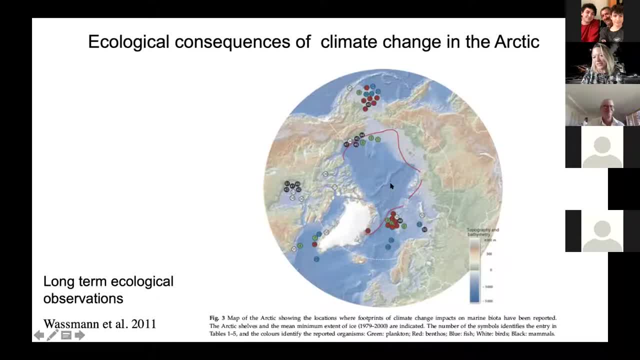 but as human civilization we have barely enough land right now to support our survival. and when we have a lot of mountain around, we can influence natural development around water, and we cannot find it. we have barely any long-term time series in the inner arctic ocean. we have barely any stable. 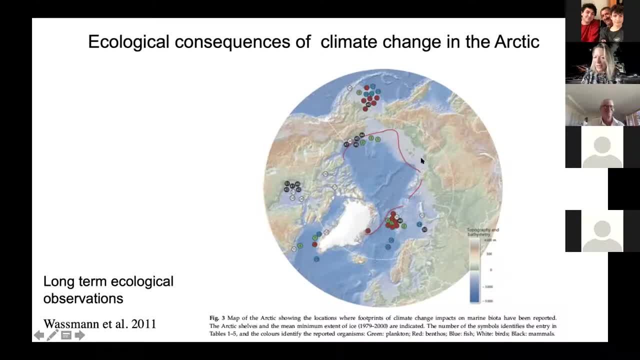 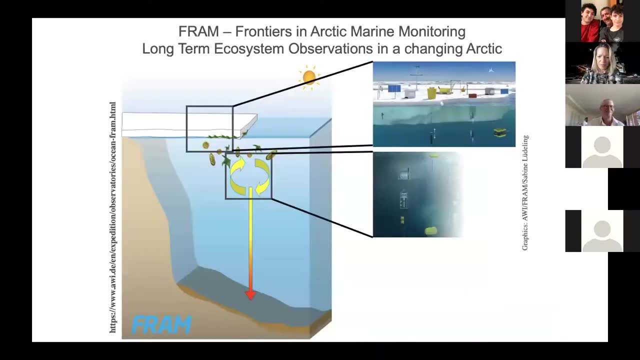 long-term time series. in huge parts of the asian continents and also in the north american ones. we have some, but there are whole areas where we just have no observations. so we really have still a big data gap in the arctic, even more so in the antarctic. so when i started becoming more and 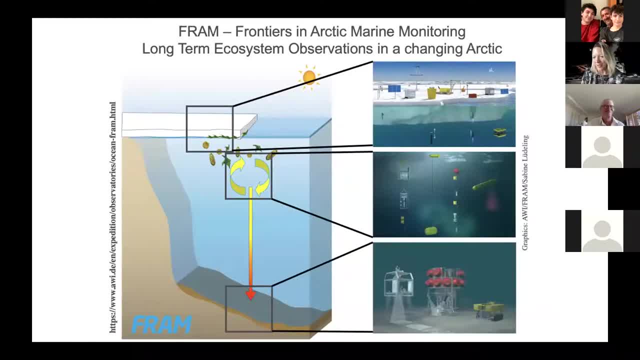 more focused on polar research and the arctic change, arctic amplification. i wrote several proposals to have a large project funded to be able to observe the arctic year round, from the sea ice surface to the vast water column. mind that the deep arctic ocean is on average. 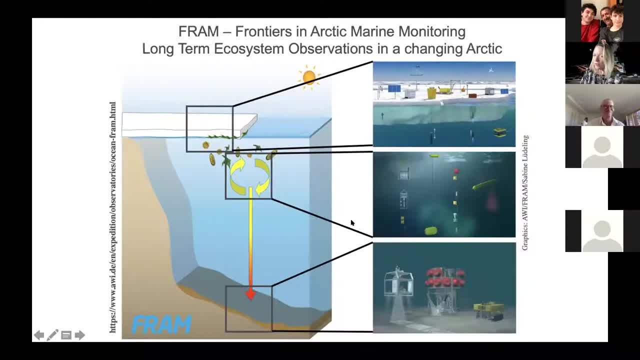 above four kilometers deep to the seafloor. so i really wanted to be able to observe, even when the ship is not there, changes in the ice and how would they be reflected in the water column and also on the seafloor. so i really wanted to be able to observe, even when the ship is not there, changes in the ice and how would they be reflected in the water column and also on the. 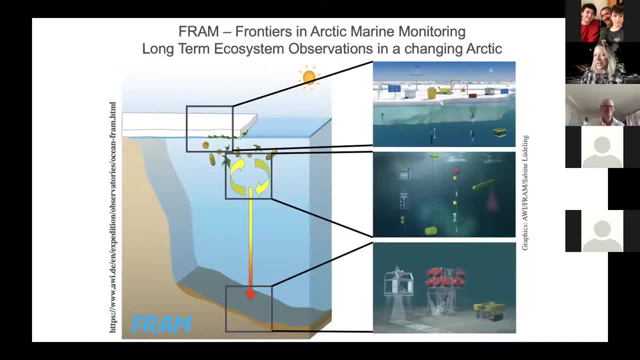 seafloor, because from deep sea ecology i know that the deep sea life that lives so deep in a dark, cold ocean where it depends on the surface born nutrition, the surface-born algal growth, there is no way that plants can live down in the deep ocean, so whatever food is like at the surface, 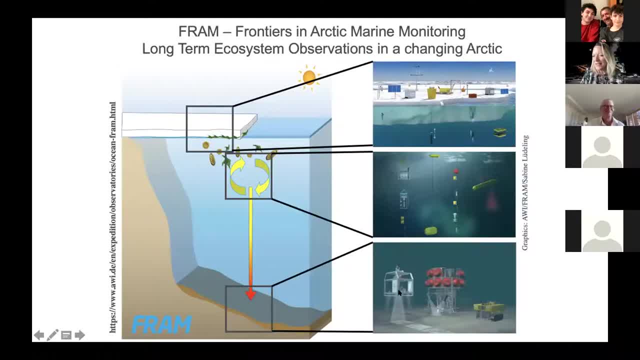 this is the food, of which a little bit will get to the deep sea, and that's how deep sea organisms are coupled to the surface oceans. so i wanted to be able, for the first time, to have year-round observations of changes in the sea ice and their potential impact on deep sea life. this we can only 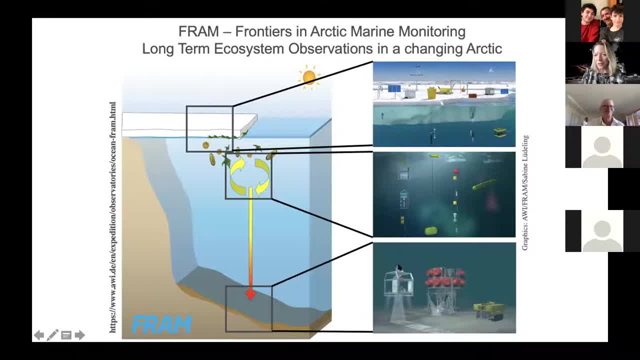 afford, and even germany, which is a rich country which has long-term, stable research funding for observations. these coupled sea, ice, deep ocean, ocean seafloor observatories with modern sensors that can last for one or two years are immensely expensive, and we just have this one observatory. 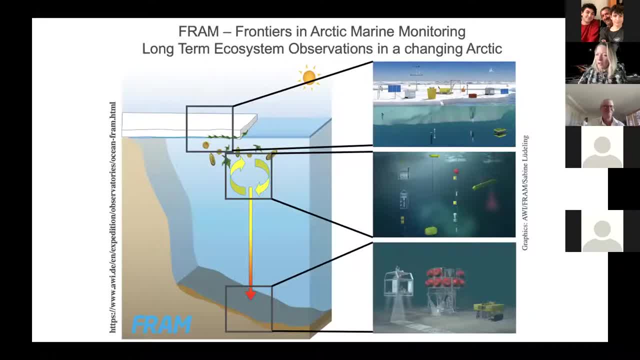 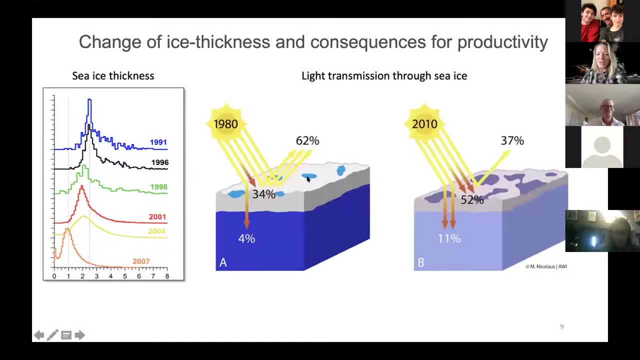 approach to the arctic and we'll struggle also in the future to maintain it. so the first thing we need to understand: when sea ice is shrinking, when it develops these melt ponds, or when it just has these leads and gets thinner and thinner, one of the changes that will occur to the sea ice and the ocean life we know beneath is the 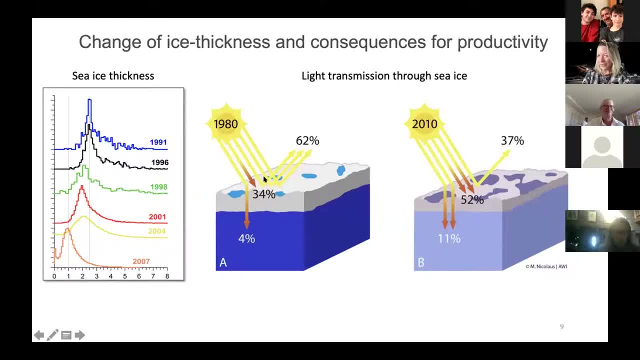 reflection of the sunlight will decrease. there will be more sunlight penetrating through the sea ice into the oceans. we know from our measurements at the avi that the each time you get slightly thicker sea ice. the飛geye to the mid-s COSTA study shows that. 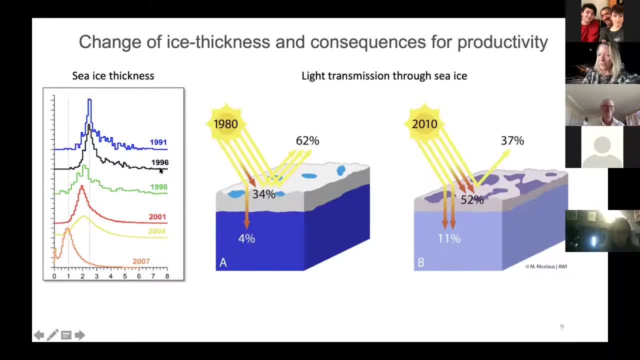 between the time when i was a phd student in 1992 to 1996, sea ice was much thicker than it is today- several. it was several meters thickness on average. uh, at that time when i was a phd student. today it is um one and a half meters, maybe, so that shrinking thickness means more sunlight into the. oceans and you would, per se say, okay, that might be an advantage to ocean productivity. if there's more sunlight getting to the oceans, that would be more thickness than you would per se say, okay, that might be an advantage to ocean productivity. if there's more sunlight getting to the oceans, there will be more, more. 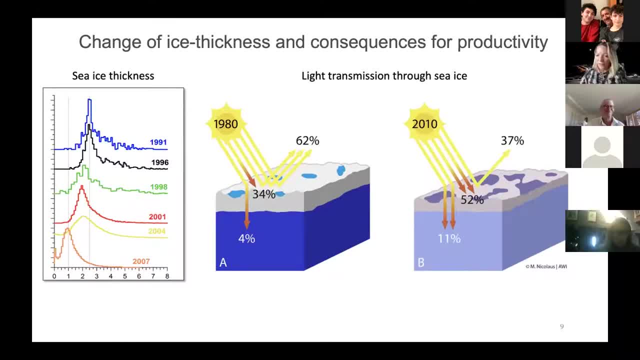 phytoplankton growing. eventually there is more food also for the fish, for the polar bears. it could actually be a favorable story for the arctic ecosystem. however, that was exactly the question of our research: what effect will more sunlight have on the local populations in the arctic? 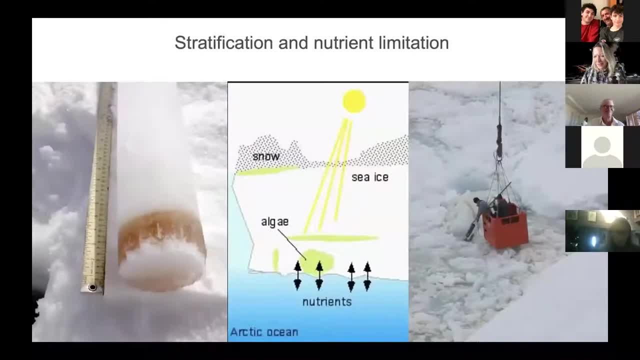 so you have to know that the life and the sea ice is very specific. it is adapted to the sea ice and the. when you take a ice core, as you see here, and you see that brown layer here at the bottom of the ice core, that's where the sea ice diatoms sit and that's those are phytoplankton, specific types of. 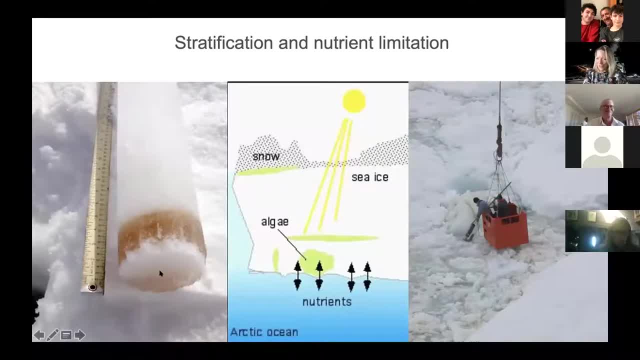 phytoplanktons. and the amazing thing is, what you find in the sea ice is different from what you find in the ocean, and so sea ice communities are highly adapted to the sea ice. they develop proteins and they develop all kinds of enzymes and other things that make them stick to the ice. they 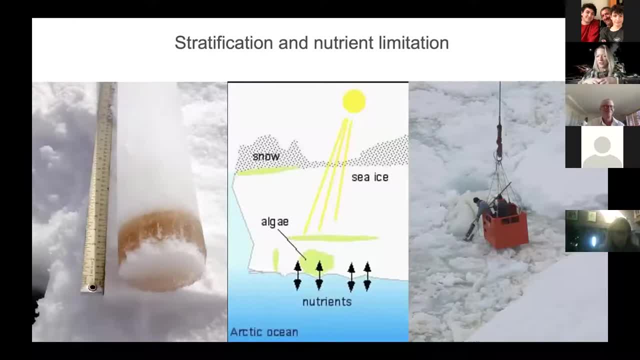 shape the pores of the ice. they live in symbiosis with certain bacteria and other critters, and so that was one of the issues and our hypotheses in the studies. if the multi-year ice, the thick ice, is shrinking away and not growing back again, that might already be a dramatic change in sea ice. 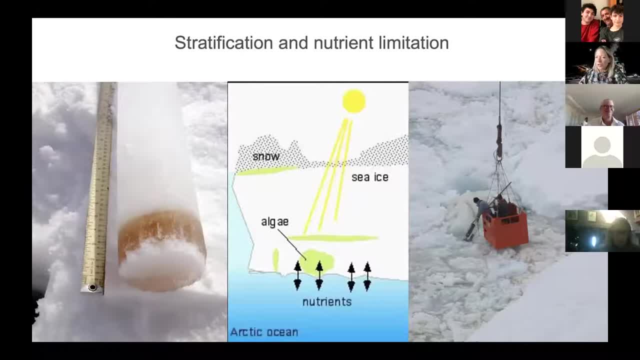 species and and that's what we found, but i will not talk so much about this today. i will try to connect you from the ocean surface to the deep sea. so the question that we had was if there is this rapid melt and there is a rapid melting of the sea ice and there is a rapid melting of the ice and 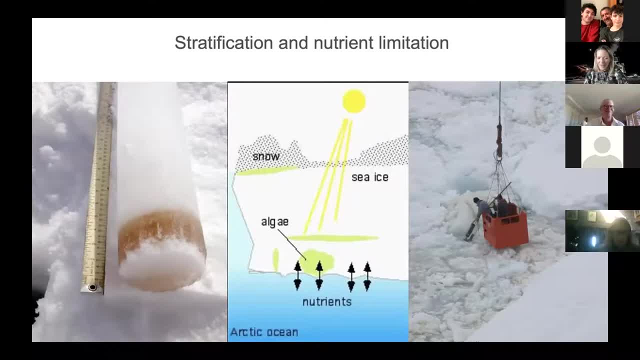 if the ocean is warming from below, then it is likely that we might lose this active productive layer of diatoms that sit at the bottom of the sea ice core in contact to the ocean to get to the nutrients, because nutrients are fastly depleted in the arctic when ice melts and 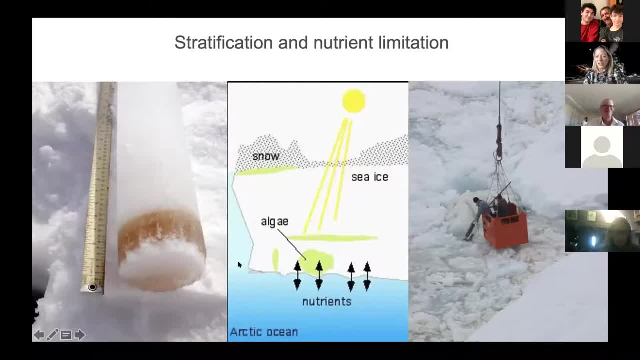 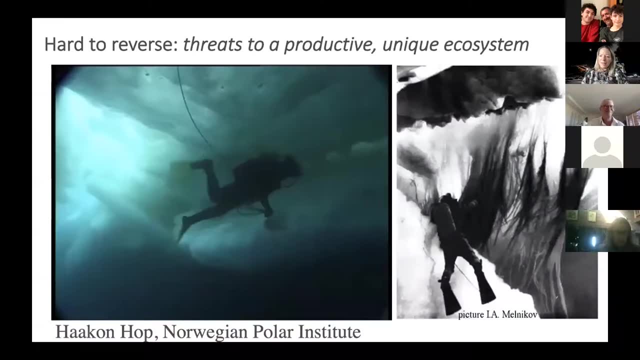 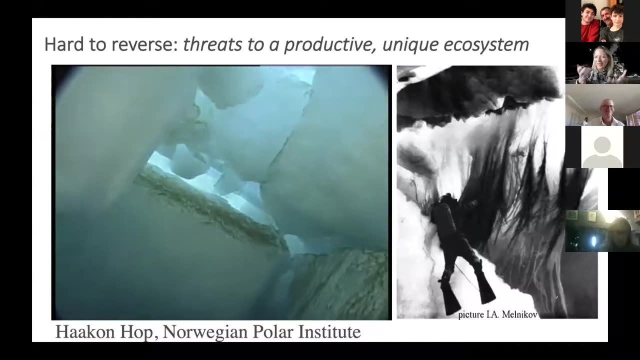 the rivers from the continents come in, you always have the situation that the arctic service water is very fresh and sits on top of the warmer atlantic water. so we will talk about that in a bit, but first let's talk about the sea ice. so you understand that sea ice when you look from it, from below, and that's true for an arctic as well. 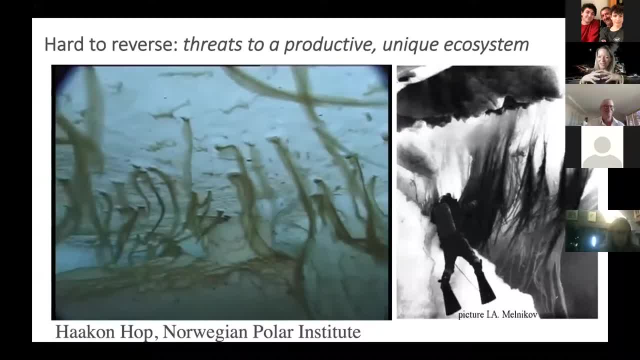 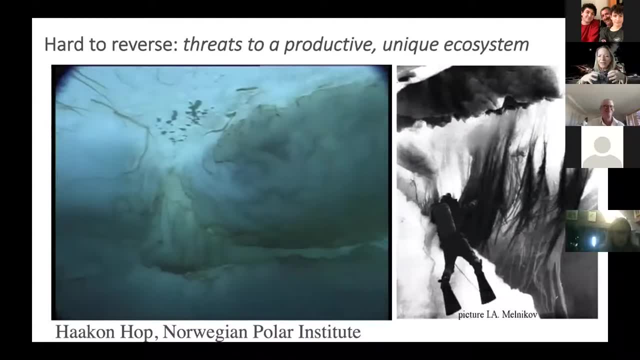 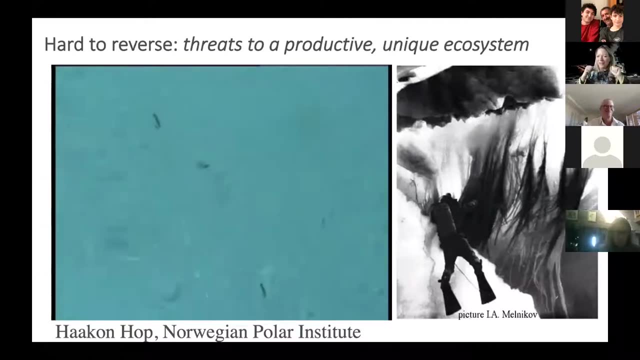 as for arctica sea, ice is actually like a reverse sea floor. it is full of life, really, and the way that the phytoplankton unicellular organisms tend to form these mats, which are then a habitat and food and an area to hide for crustaceans and larvae of fish and all kinds of life, then you. 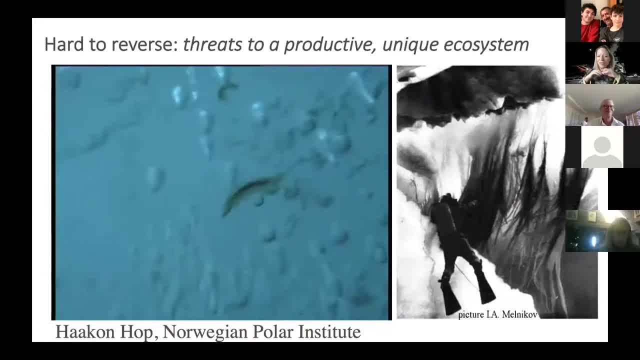 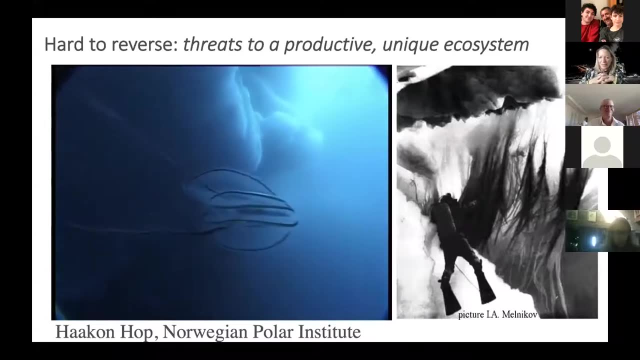 and so on. and, in fact, when you have these observations, you also understand how tightly adapted all kinds of of animals are to manage to feed from the under ice life. note that in both oceans and arctica and the arctica, a lot of the ice- the sea ice- adapted life is actually. 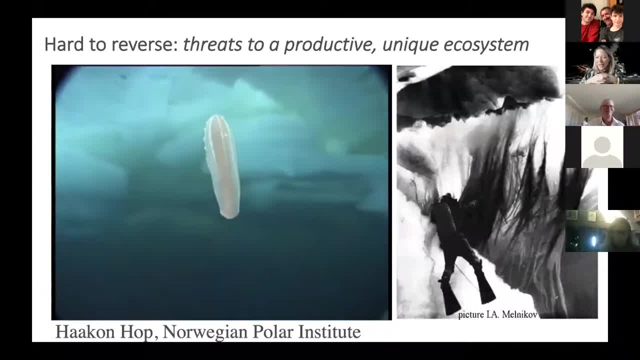 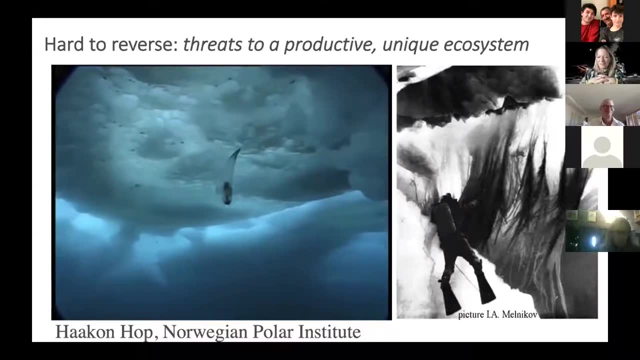 gelatinous jellyfish life like you see here, and this one is really hard to get to. you cannot catch it simply by nets, because it's like jelly. it will fall apart in pieces and when you you have to use robots or divers to actually observe the immensity, the diversity of sea ice adapted life that feeds from that phytoplankton growth. 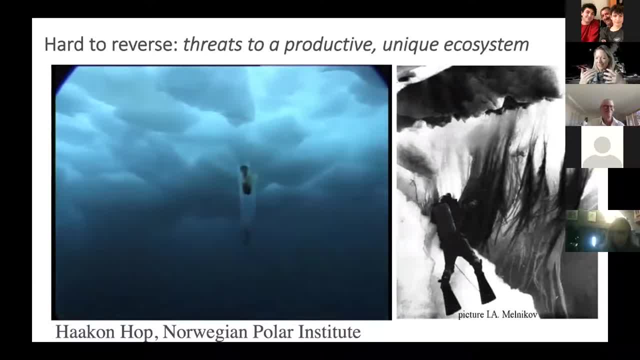 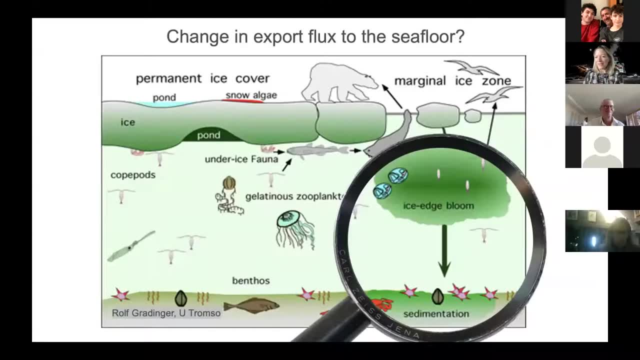 now imagine that sea ice goes away. sea ice is melting away, and then it is clear that that will change, of course, food webs, and that's that was the second part of our studies in the in the recent years. we wanted to know exactly that when the sea ice is shrinking and melting. 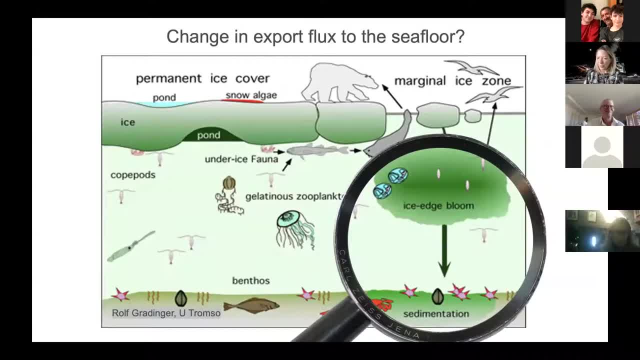 is there maybe a balance, because thinner ice means more productivity? or if the sea ice goes away, does it actually mean less productivity because you do not have the normal food webs that you usually have in the arctic? for that we needed to put up traps in the oceans to catch what? 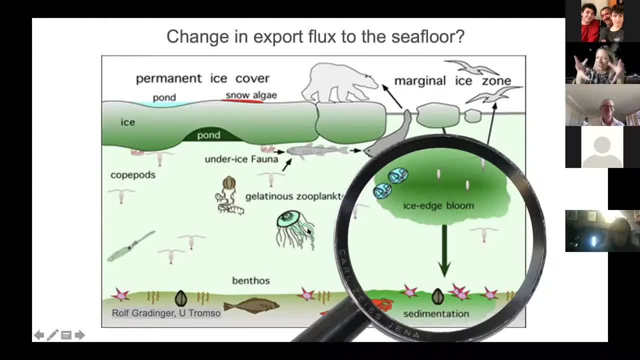 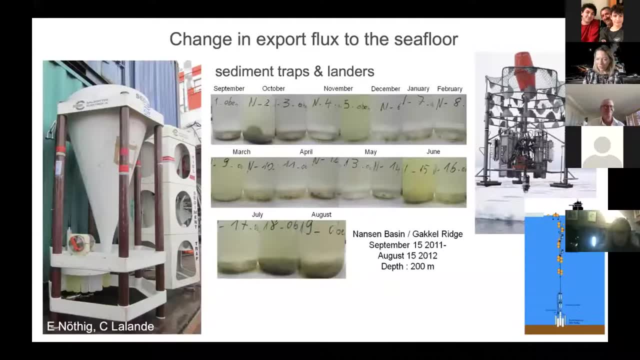 falls from the ice to be able to know how is actually the export from the primary productivity, the feeding of animals, down to the deep sea. so for that we use sediment traps. sediment traps really are traps. they are like these big fish, funnel-shaped cylinders that you moor, that you anchor in the oceans and then whatever falls they. 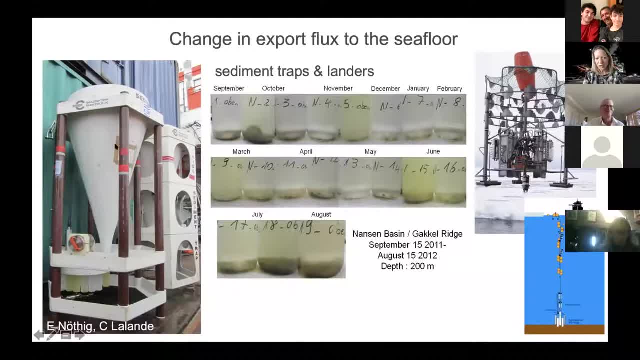 have standardized sizes. whatever falls from the ice, from the ocean surface, maybe to depths at 100 and 200 meters, or down to the sea floor, is caught in rotating and revolving bottles, and then you know for each month. here you can see the difference between the months, you can see for 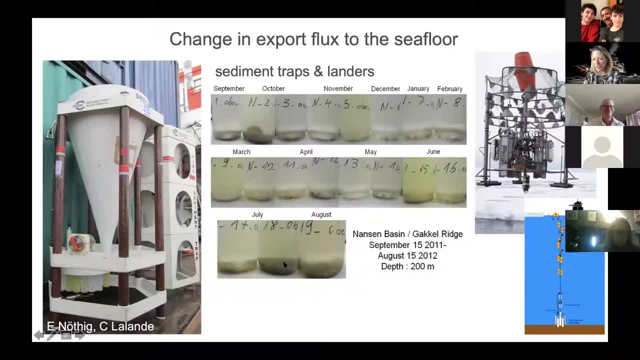 example, in summer time is much more stuff caught than winter time, of course, because in summer time there's light and primary production, in winter time no light, but still some stuff falls from the ice into the deep sea. so we did these observations and you can imagine that it's. 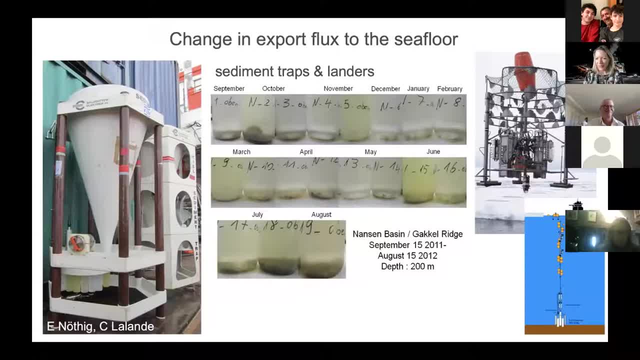 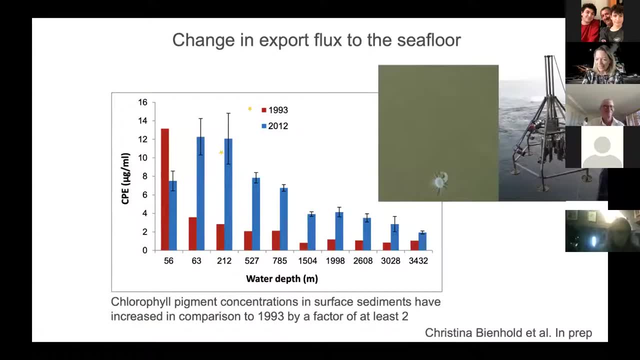 really hard to anchor such moorings in the ice and get them back from the ice, but we've managed to do a kind of a time series with time and we were able to see that, yes, there is an increase of productivity and an increase in the amount of carbon of export of phytoplankton detritus. 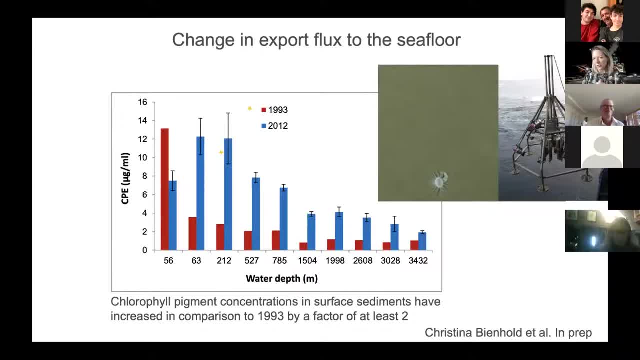 from the, the surface, from the ice, into those traps, and we also saw that on the sea floor. what you see here in this graph is a comparison of my phd studies, data 93, to the mission i was on in 2012, and you see plant pigments. we call them chloroplastic pigment equivalents. that just means. 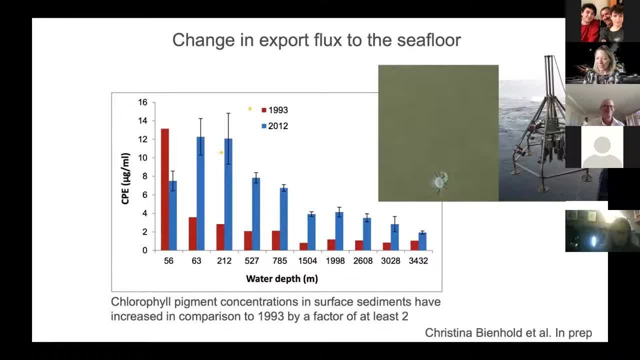 the, the pigments that that algae produce to catch sunlight, chlorophyll- and you can see, when you compare the red bars, that in my most water depths of the arctic, in fact, the amount of plant pigments that are exported to the sea floor have increased, speaking so confirming the hypothesis that thinning cis will allow for more. 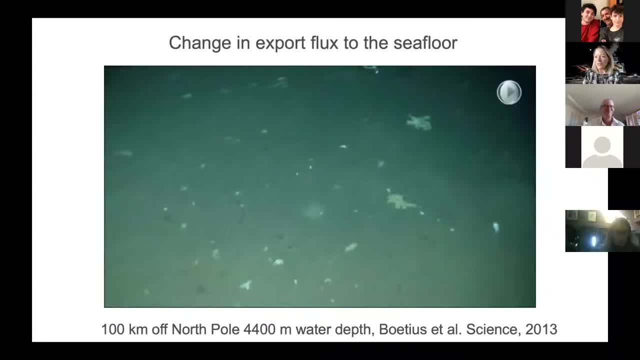 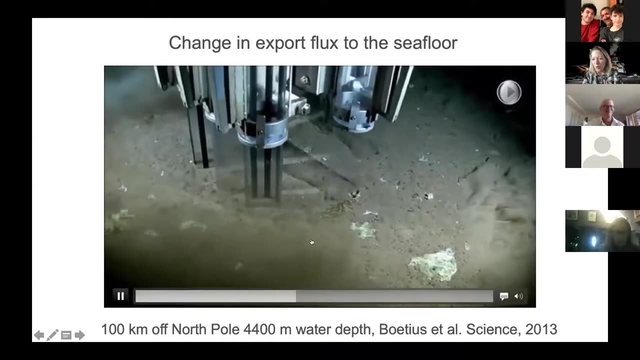 productivity. but what we were really surprised to find when we used cameras to the ocean floor in 2012 was that it wasn't all about the small rain of marine snow, of small phytoplankton detritus, but actually on the sea floor, around the sea, uh, the north pole, at 4 400 meters water depth here. 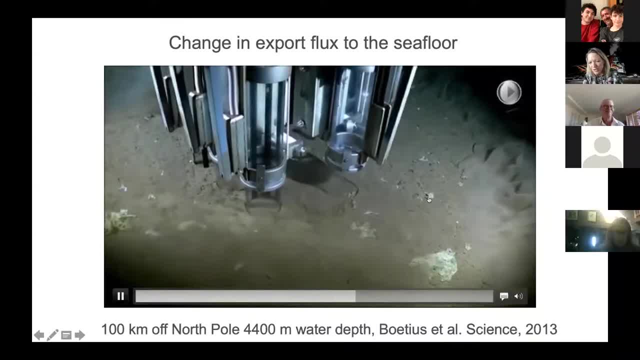 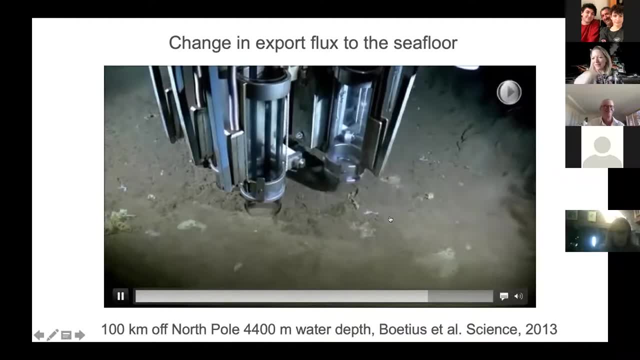 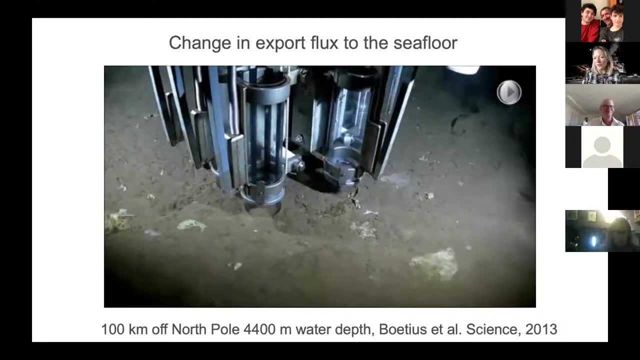 we are catching some of the sediments. you see these greenish, whitish dots here, and these larger blobs of material are actually the the decaying big sea ice algal mats that i showed you before from under the ice. so what we observed was that when ice is melting away, basically it's not only 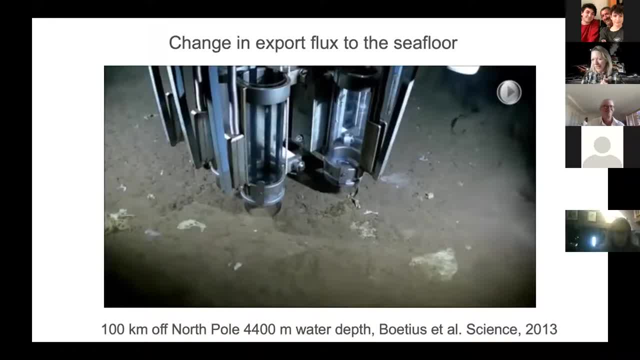 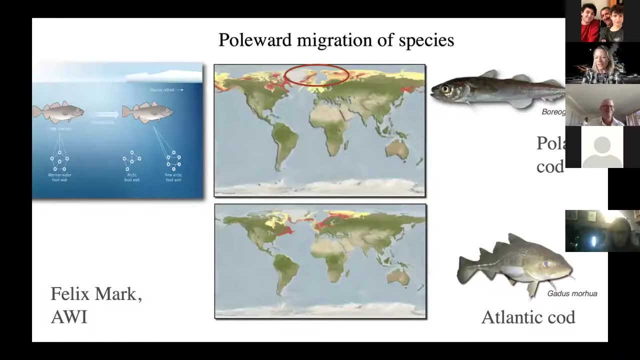 the normal export of little bit of detritus that is left, but basically everything that lives in the ice when the ice melts away falls to the deep sea. so a completely different nutrition of deep sea organisms and it was really amazing to see that many of the deep sea life 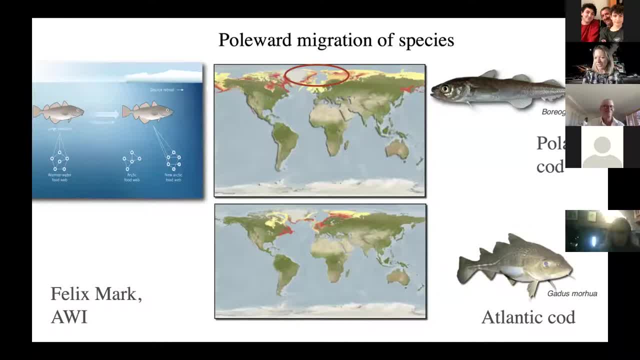 weren't even able to use that new food source because they were not adapted to eating gelatinous mats. we found a few sea cucumbers, a few um of the ureth, so starfish that could eat from it. but we are just at the beginning of potentially seeing a transition into a whole new deep sea ecosystem. 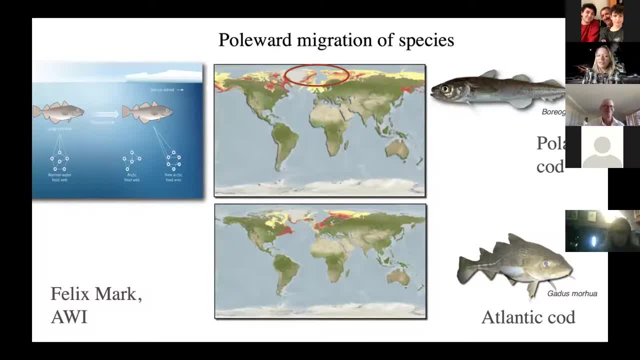 in the arctic we saw more. for example, what we're seeing in recent years is the poleward migration of species, because european waters in the atlantic are becoming so warm that the cod- so fish that we fish also for industrial commercial purposes- have to migrate to colder waters to reproduce. 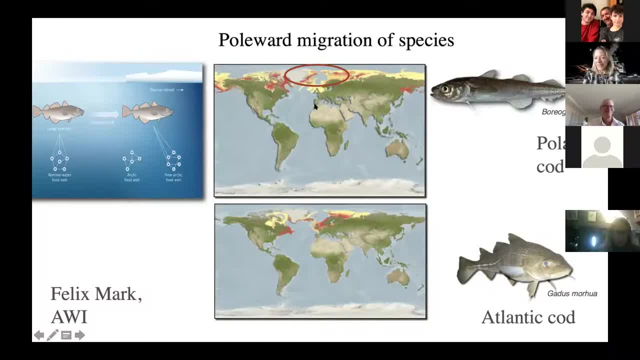 so the atlantic cod has moved up quite far into the arctic and in fact from the few service that we took us with ocean robots and cameras, we saw the haddock and we saw the atlantic caught reaching really far up, almost to the north pole. we don't know if they reproduce there yet, but we can see that. 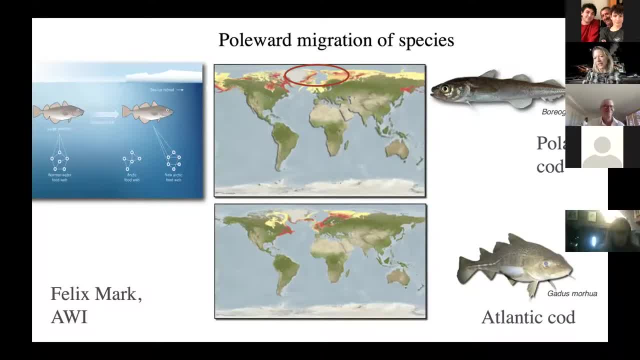 that's what we call atlantification, that with the warming of the atlantic waters, with the shift of the climate zones, we'll get a whole migration of organisms, and that, together with what i've just reported about the food web, that will probably change everything in the future. 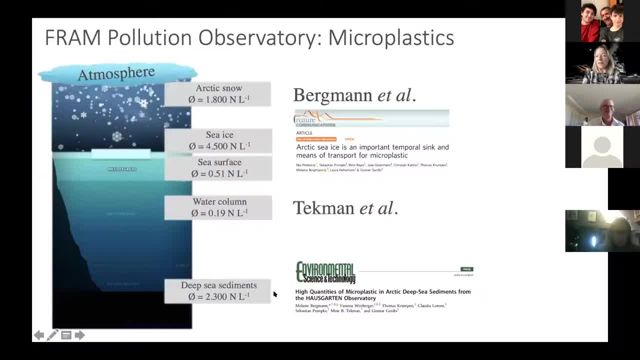 and there's even more when, in the past 10 years, we were alerted by our camera pictures from the ocean and the sea floor. we found out that the arctic, the way that it changes, the way that snow precipitation, sea ice formation, sea ice melting and access to the arctic by ship changes that of 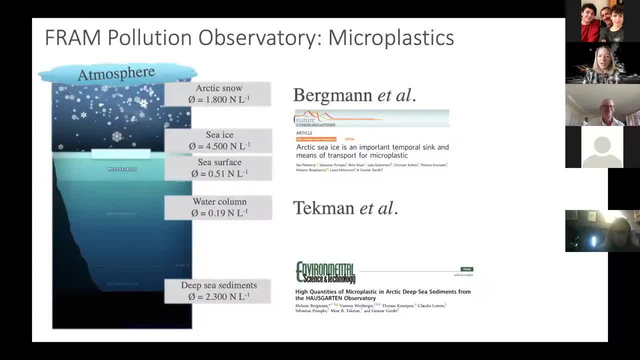 course we were also able to see, with our observatory, a rapid increase in classification. you might be surprised that i call it that, but in fact today we know that in all ocean regions we have an accumulation of plastic particles from human civilization. some of it is far range. 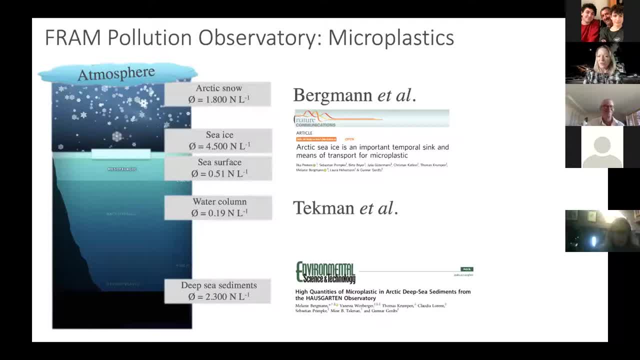 transport. some of it is local transport, but we were able to show with our observatory, from the atmosphere, sea ice to ocean and deep sea life, that already now, in these times, there is a huge accumulation of microplastics, so plastic particles as big as maybe a few feet long, and so on. 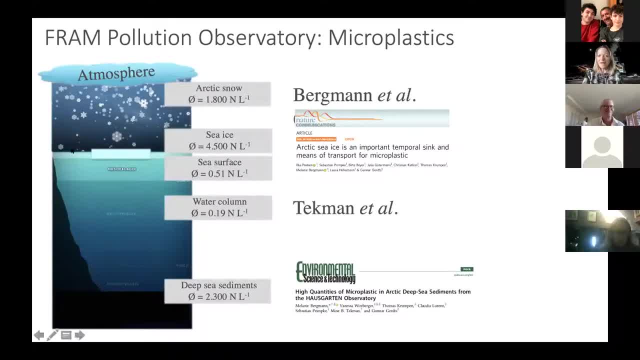 millimeters or smaller. they come through the atmosphere with snow, they rain down on sea ice. when the sea ice melts they are exported to the sea water, to the deep sea sediments and in fact the sea ice is actually focusing and concentrating those particles so that we really have high 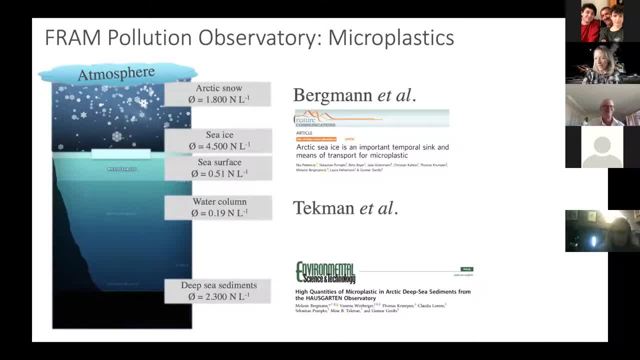 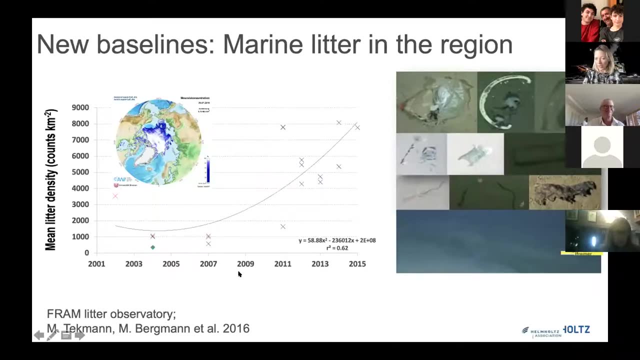 numbers in the arctic, deep sea sediment in antarctica. we have been beginning to study this. we are not so sure yet, because the distances to continents is, of course, far greater. also, where the sea ice recedes, we get an increase in macroplastics, so the remnants of civilization. 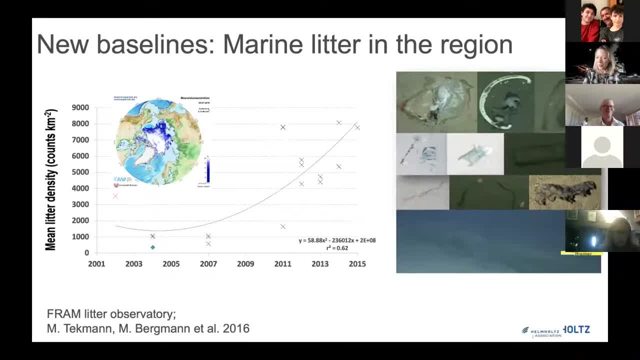 be it fishery nets, be plastic bags, be all kinds of disposable items. here you see our time series observation from the atlantic: uh, deep water access to the arctic. in the recent years there is a huge increase in large plastics and actually where you see that, that the sea ice is receding, where 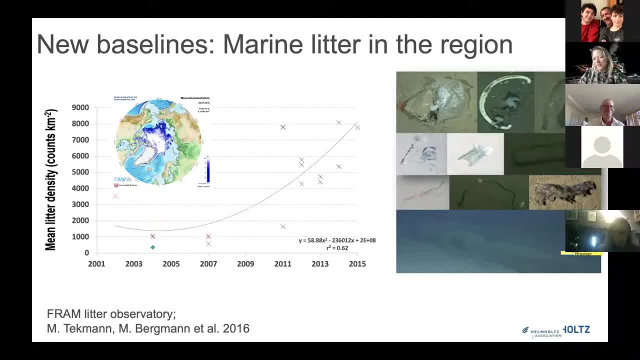 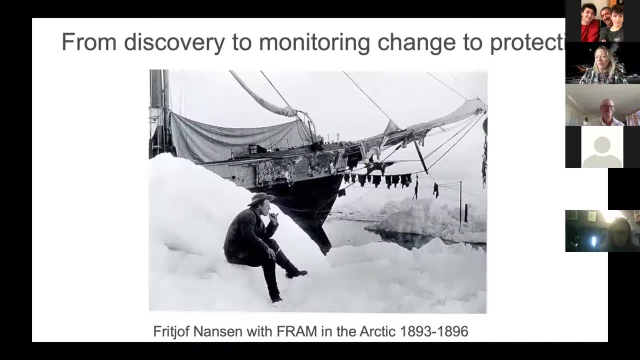 more tourist boats and fisher boats go. we have this increase of life and we have a lot of large plastics. i will now come to the story of mosaic, now that i've told you a bit about my own research and trying to get year-round spatial and temporal synchronous observations with long-term observation. 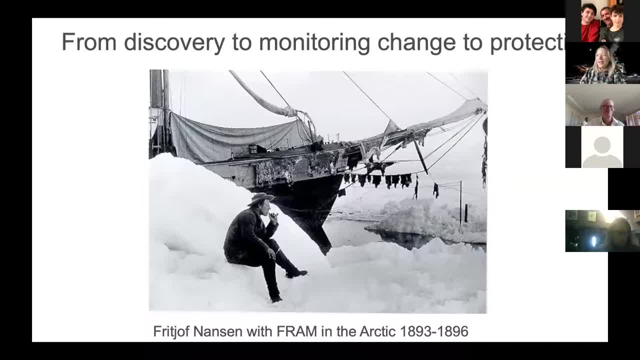 connecting eyes to the sea floor. in 2011, a wild group of atmospheric researchers came together worldwide to propose one unique mission to the planet, basically to explore this wide area, and this is one of the most complex and exciting scientific and science activities that we have seen so far. this is a very interesting experiment that the scientists 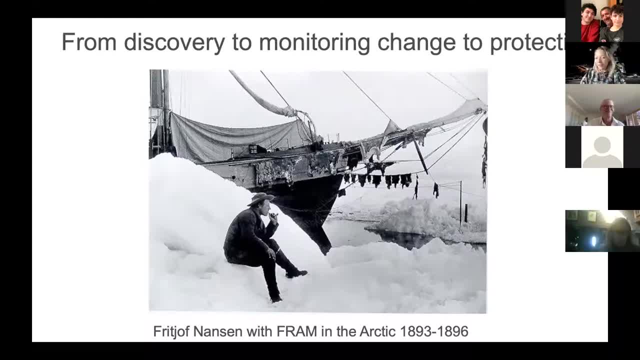 ね did in the early 1990s. they were doing in the marine science and that was to go and have their ships frozen in for an entire year, just as fiti of london the norwegian did. he did it actually for three years, which is wouldn't ship the farm some 125 years ago. 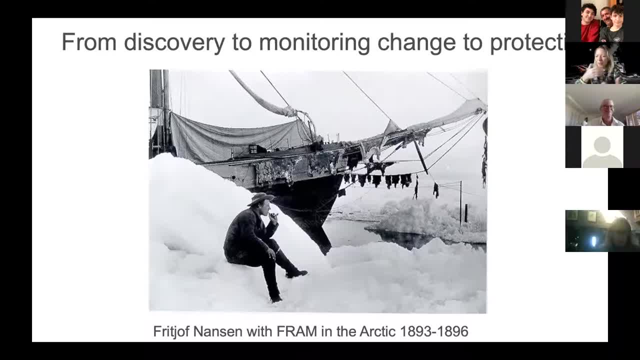 but thought it's impossible to do such a thing because you have to exchange people, you cannot keep them for a year, and it was deemed a great idea but unlikely that it could happen. but eventually, with the knowledge of arctic change and arctic amplification, enough support got together. 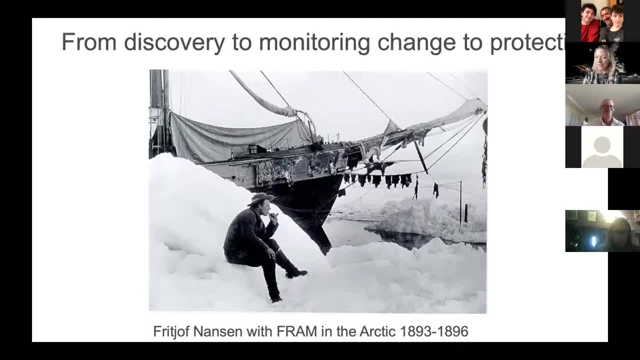 that the mosaic mission actually took place and they returned last year in october and i'm very proud to say that we've managed- the arby was the coordinator of that mission- that we've managed even to carry on expeditions throughout the entire pandemic. what did manson want at his 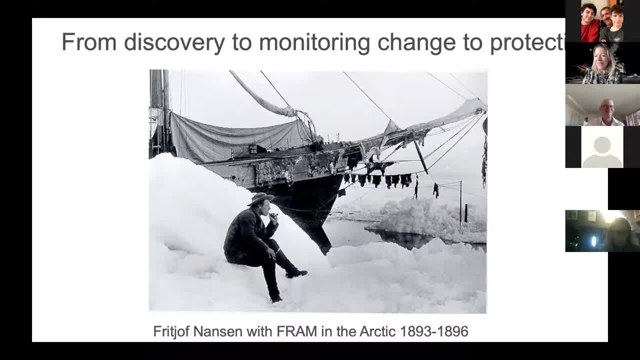 times you see him here sitting, smoking and thinking, and he was actually the one oceanographer that showed that sea ice is drifting, that there's no continent in the arctic, it's just an ocean with ice on top, and also he wanted to show how deep the arctic is, but he didn't have enough rope. 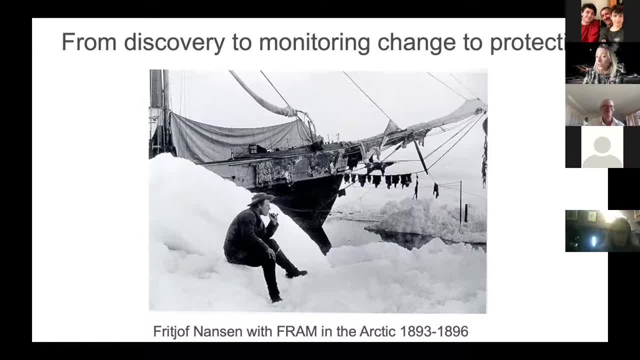 he also wanted to show that, how cold it can be. he forced other physicians to calibrate the temperature so that they could really determine how cold it can be. hence we have his data for a comparison. so this was a fantastic mission that he did. he wrote great books about it and uh, but 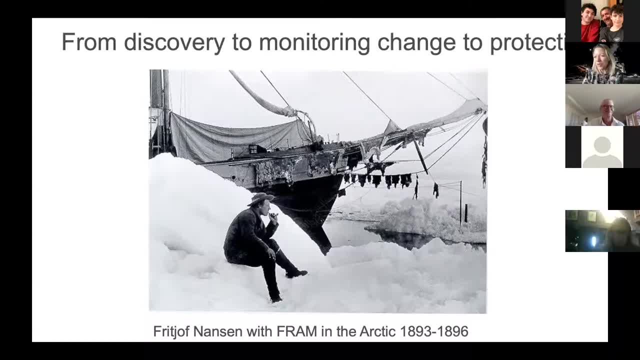 we were the ones challenged by this idea that we would manage it with our polar research icebreakers. mind that some other people have managed to stay in the arctic for a year on a sailing boat doing some research. others stayed there with the research expedition closer to the shelf, the famous shiva. 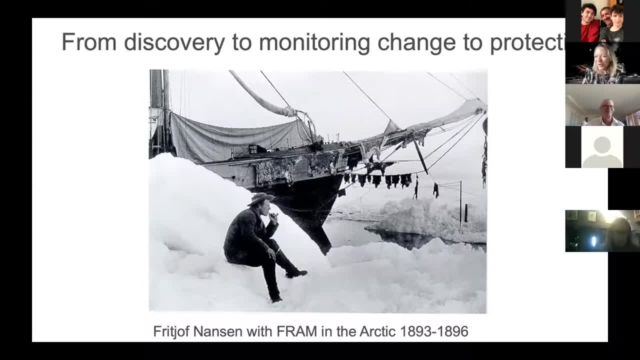 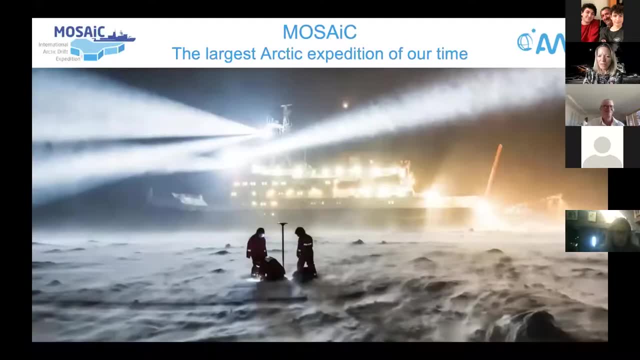 was able to actually camp out for many years out in the arctic, drifting on an ice flow, but since a few years this is no longer maintained because the ice has gotten too thin. so how did we do that Expedition and what did we want to see? it was a mission that brought together 450 scientists and 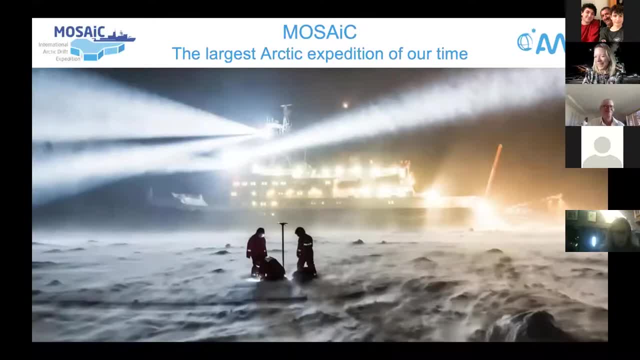 crew throughout the year and the scientists came from more than 20 Nations. it was really a international experiment. there were PhD students, scientists of all ages and disciplines together, and I don't have so much time to show you a lot of the eyewitness reports, but I would like to show you one small video clip that explains once more. 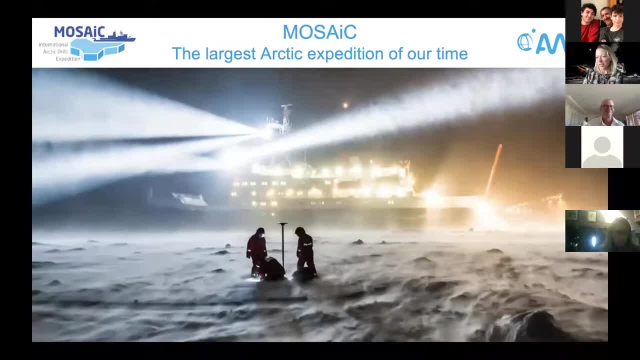 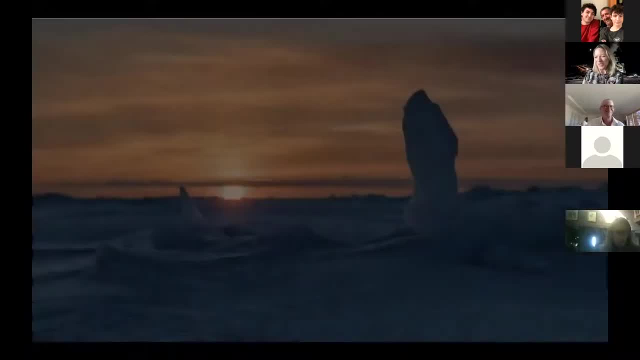 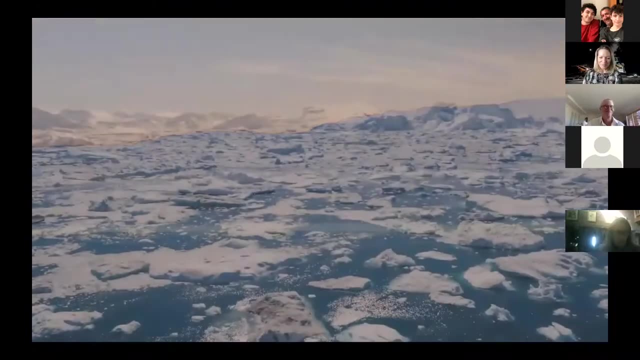 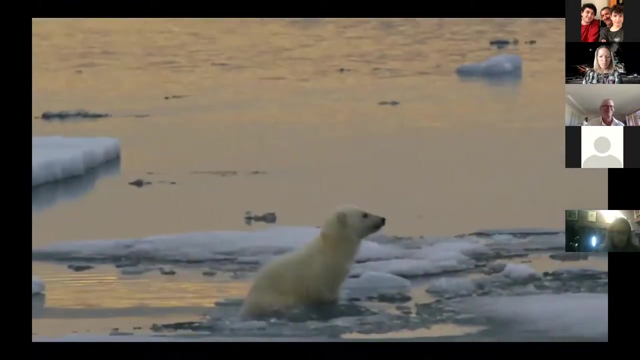 what methodologies were brought together to be able to do a synchronous year-round measurements. so I'll be quiet now for three minutes and please enjoy this little clip that should explain to you the technologies of the mosaic machine. Arctic, the northernmost region on Earth, cold, remote. even here the extent of global warming can clearly be seen. 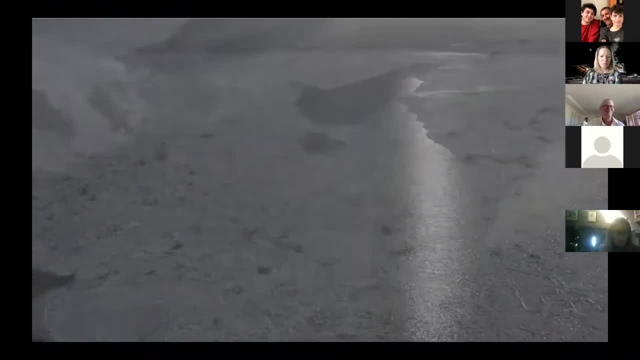 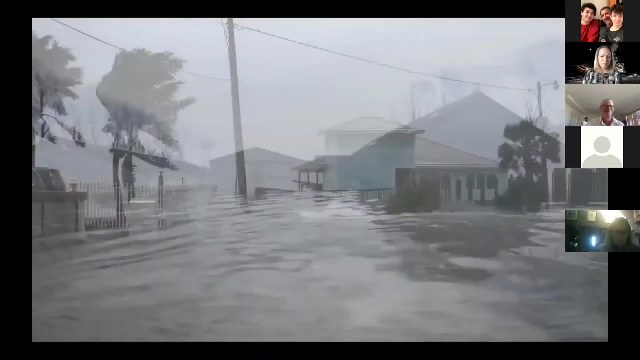 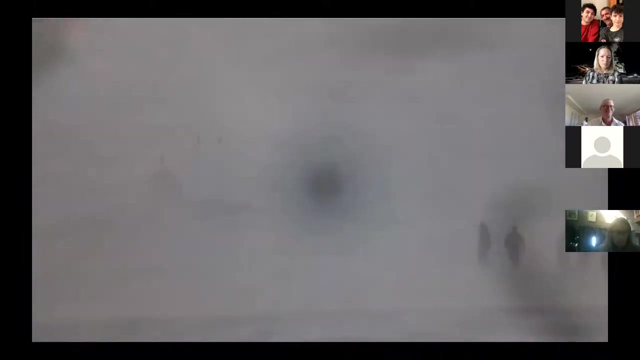 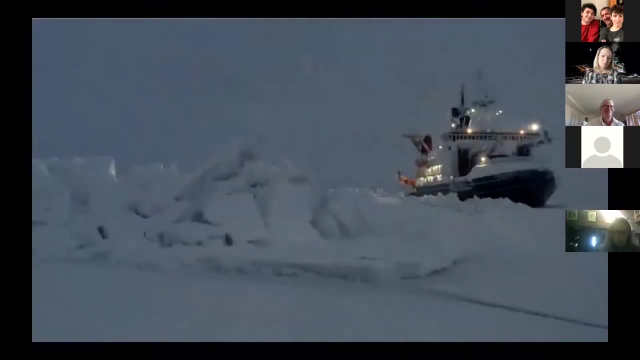 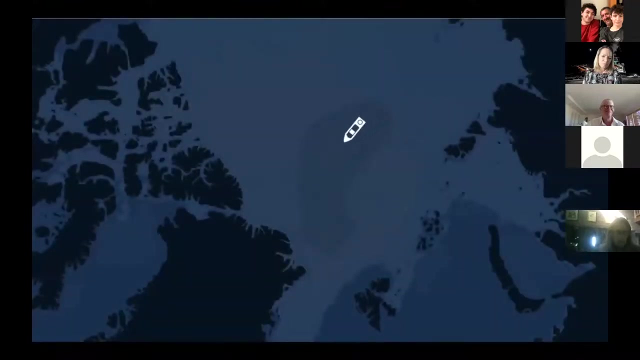 the Arctic ice is rapidly thawing, with dramatic consequences for our climate. in order to better understand the climate processes in the Arctic, we need to take measurements year-round. to reach the Central Arctic in winter, the Polarstern must freeze herself in the ice and take the natural ice drift all the way through the Arctic Ocean. this is the mosaic Expedition. 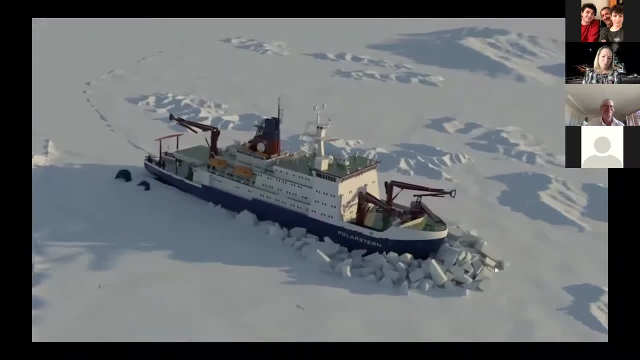 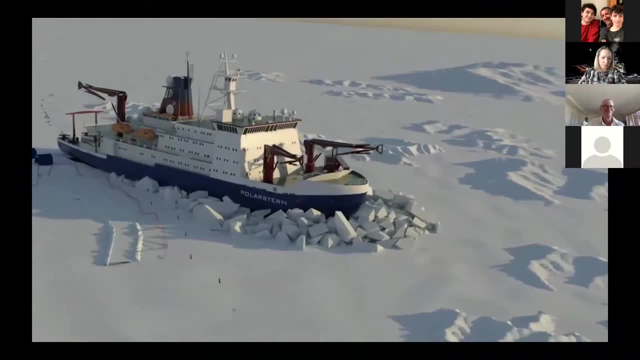 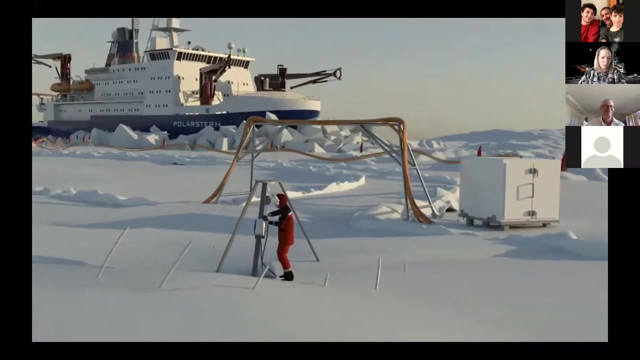 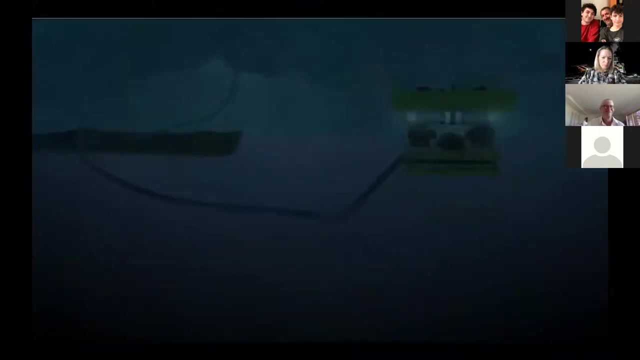 under the direction of the Alfred vegana Institute, scientists from all over the world are working together and have set up a research camera on the ice. this includes an rov City where researchers use remotely operated vehicles to collect observational data under the ice and transmit it back to the surface. 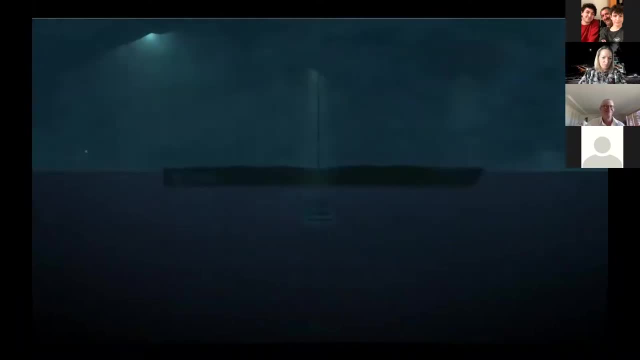 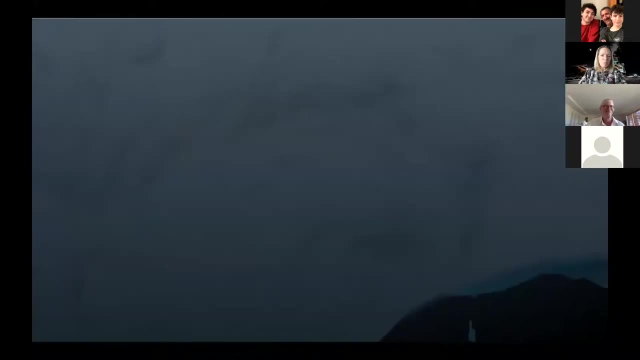 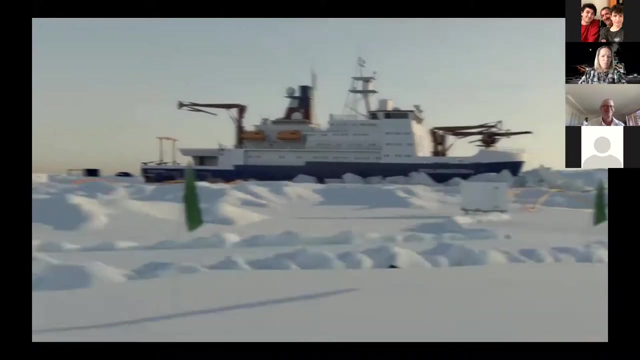 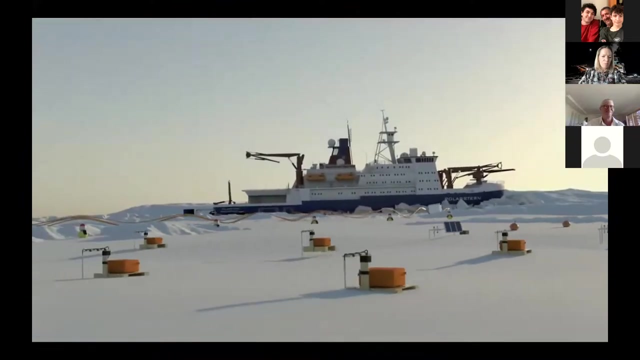 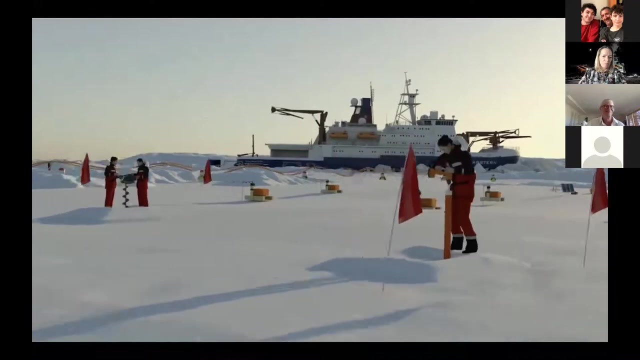 there's also an ocean City. foreign experts lower measuring equipment through hosu D ice and haul water samples to the surface. there is an ice research camp where researchers study and observe the sea, ice and snow cover. there is a met city and balloon town where the researchers collect data on. 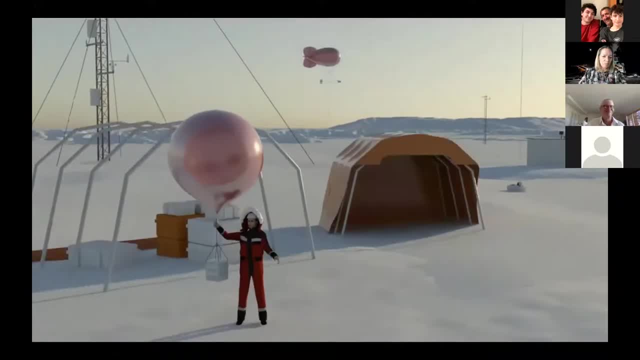 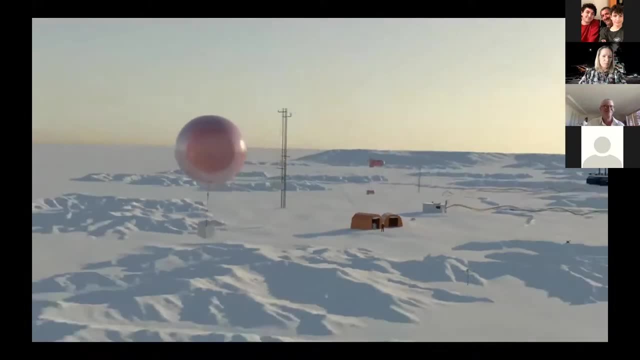 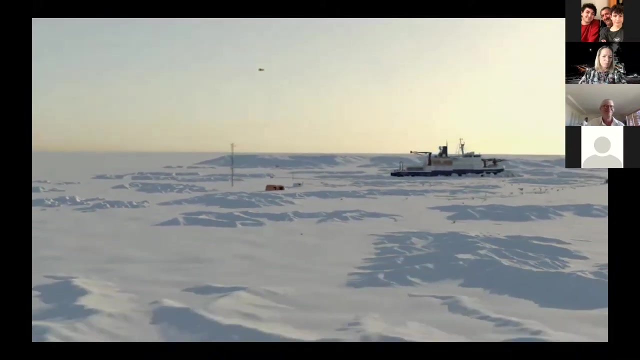 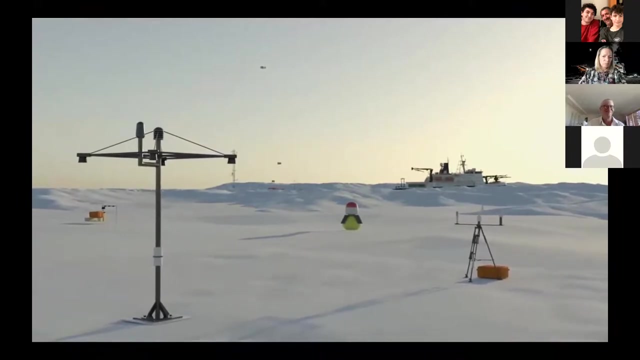 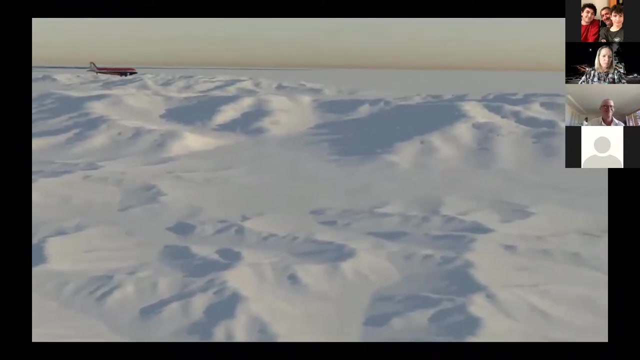 the atmosphere and air composition up to 50 kilometers around the central observatory. several dozen ice monitoring stations have been installed. they drift with the camp autonomously, recording and transmitting measurement data along the way. additionally, aircraft augment the study of the ice atmosphere and clouds by taking measurements. 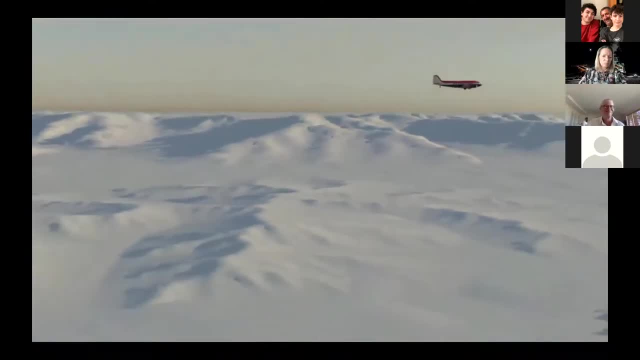 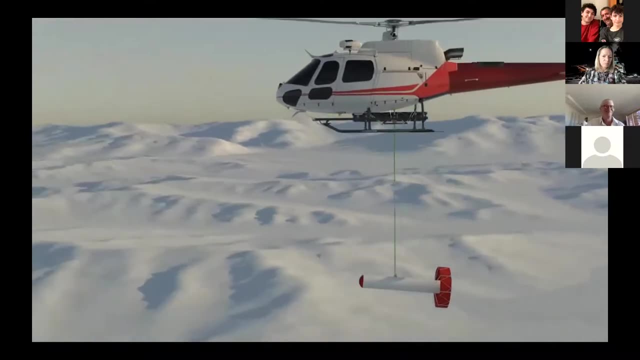 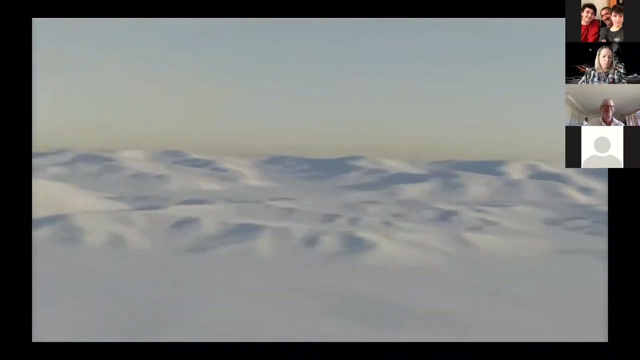 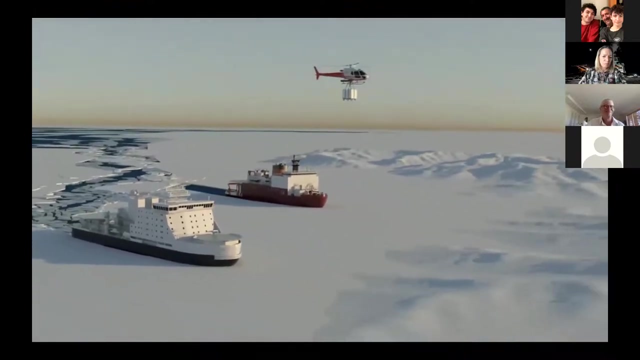 from the air. icebreakers from international partners are available to exchange scientists and crew as needed. the overall structure of the ice breakers is made available to scientists and crew as needed. the overall structure of the ice breakers is made available to scientists and crew as needed. 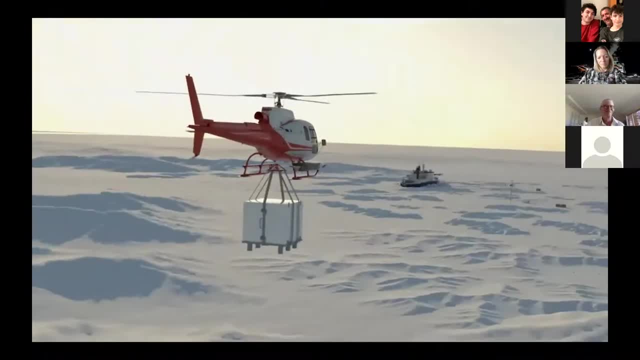 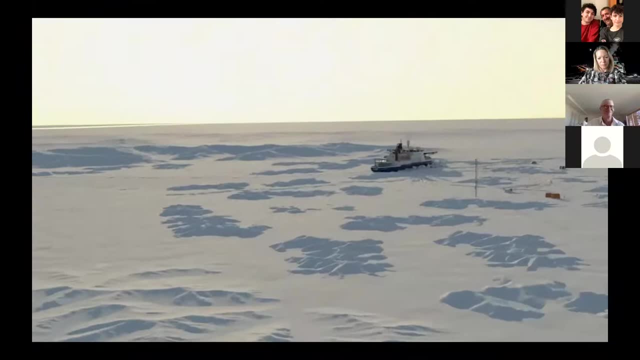 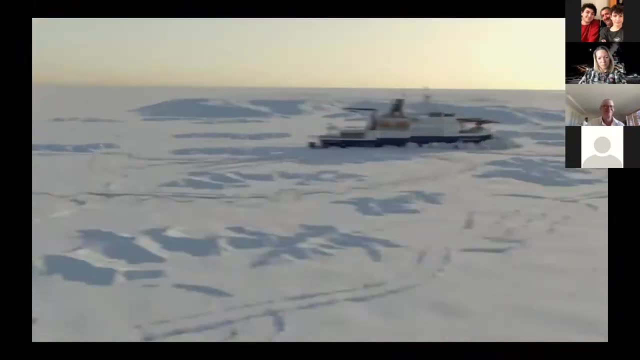 the polarishtian research camp and surrounding measuring stations. the polarishtian research camp and surrounding measuring stations will all drift through the arctic for an will all drift through the arctic for an entire entire year, collecting valuable data. this data will be vital to understanding the arctic climate. 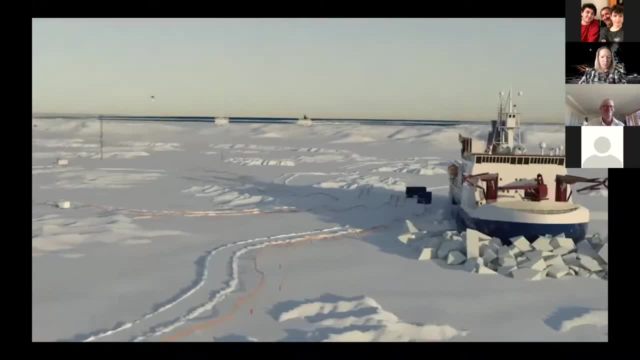 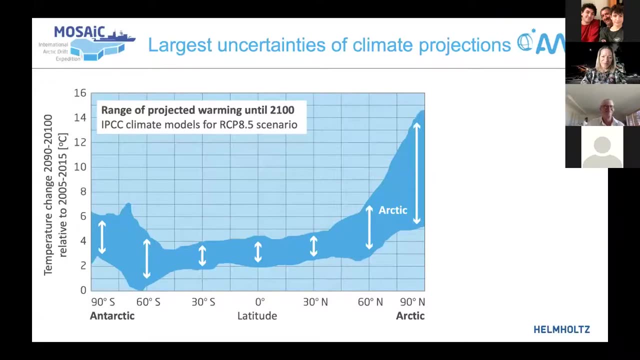 and how it will impact the rest of the world, world. so exactly that, um that, those are the last few minutes of my talk now before we will discuss exactly. that was the great uh part of the mission. that is not ended just because the expedition has ended. but now you have to imagine, all of those researchers are back with their observations. 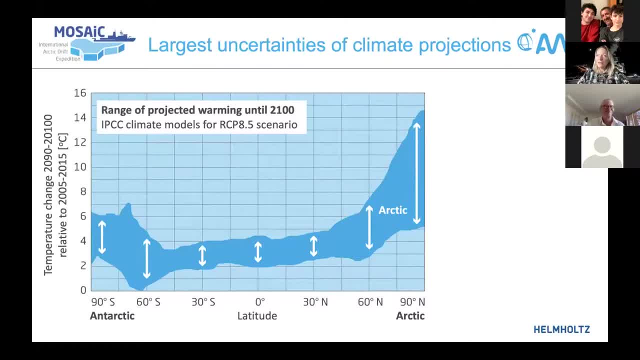 measurements and we were able to have for this year synchronous measurements from as uh high up as as 30 kilometers in the air and as deep as four kilometers or almost full bottom range, and we need to put from all disciplines that we had so: ecosystem, physics, atmosphere, sea, ice, oceans. 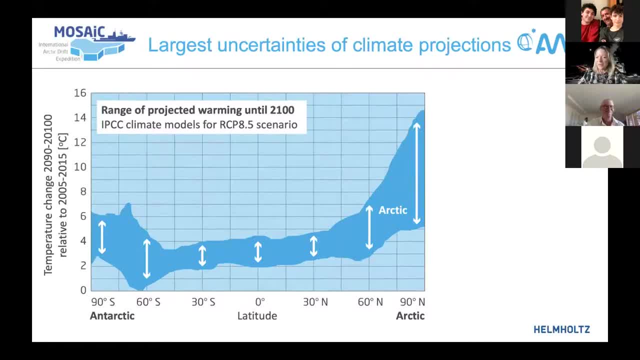 everything together, um, so that we can answer this urgent questions. how can we better predict how the warming in the arctic will develop and how the seas will develop? um, it is quite dramatic when you look at the range of projected warming. so i just heard the end of your discussion and 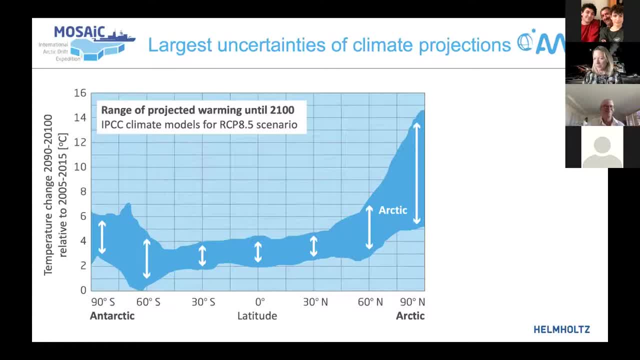 you just discussed uncertainties: how. how will they better be? better knowledge, better prognosis of the question of future ice mass loss and this exact question we have for the arctic. not many people know that with the um rcp 8.5 scenario. so business as usual scenario. 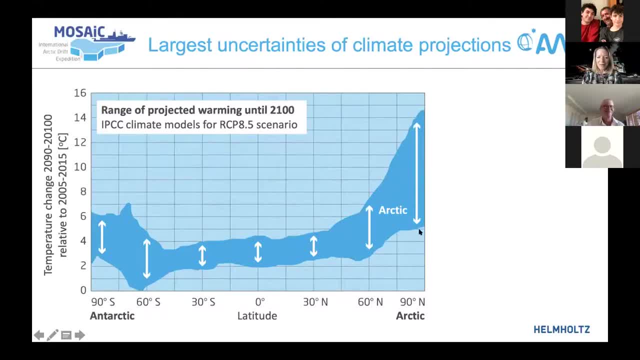 will have this quite um inquiring problem, knowing how the arctic will change. we always discuss, like two, three, four degree warming, global warming, but in the arctic, as you can see here on that graph, the uncertainty is much, much higher due to the amplification effects. so by various effects, it 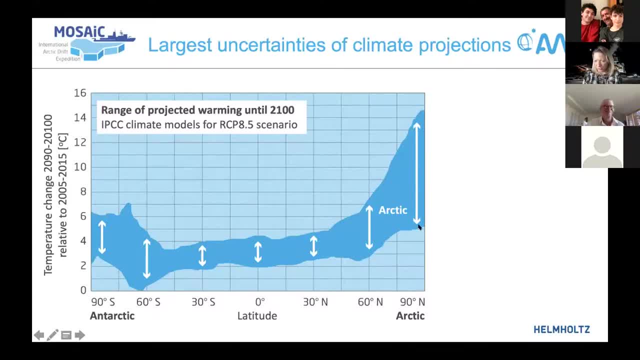 might well be that what we currently would think is a four degrees increase in arctic warming might end up to be a 10 or 12 or 14 degrees increase in warming, and that uncertainty is, of course, dramatic for the cryosphere because it could mean- and there are- self-perpetuating 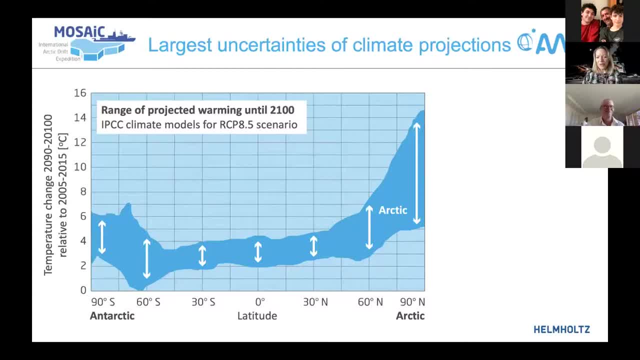 feedback cycles. when it comes to ice, it could mean that we are losing cis much earlier than we are. and then there is also the big scientific question of what does it change the way? does it change the way we live? so what does it mean if the north pole changes of sea ice is lost? what 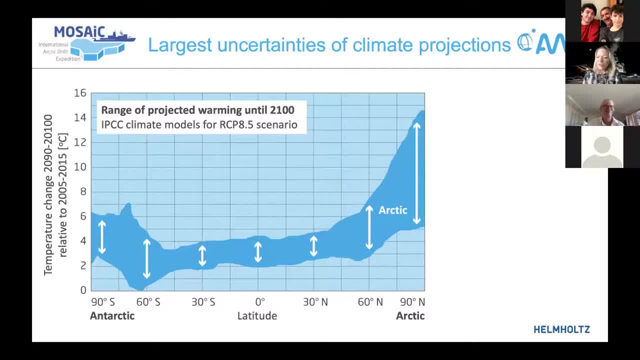 does it mean to the rest of the world? those questions were tackled in various ways by mosaic. just to say what we already observed: comparing the temperature measurements of fritjof nunsen 125 years ago to today, we were really struck to find out that the north pole region has warm. 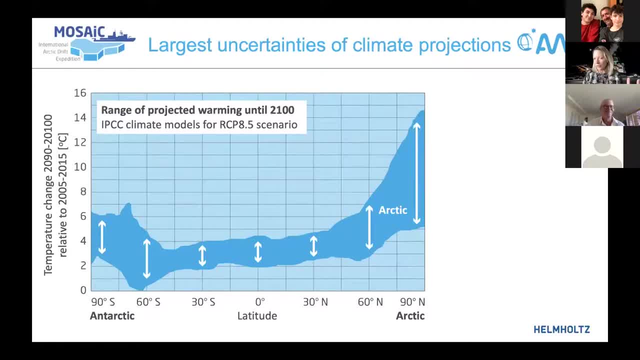 already by 10 degrees, comparing the winter of nunsen's expedition to the winter that we witnessed. so normally there is no meteorological station and no observations, except from a few drifting buoys, because there are no ships in winter time. and you see this to even make people 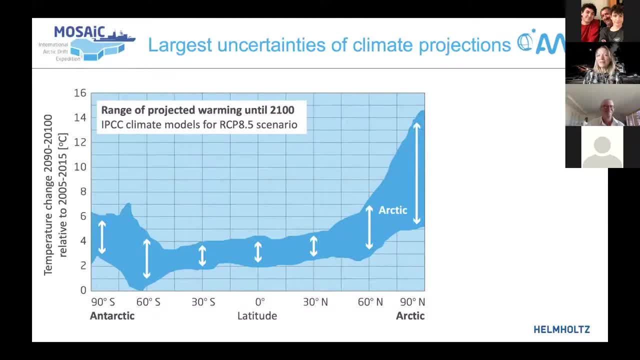 understand that, why we all know how dramatic planet earth is changing. in many areas we have no observations, we are blind, and so, in that regard, i'm hoping much that this mission will change the way we understand the arctic. but we need to connect everything: atmosphere, ice, oceans and life. 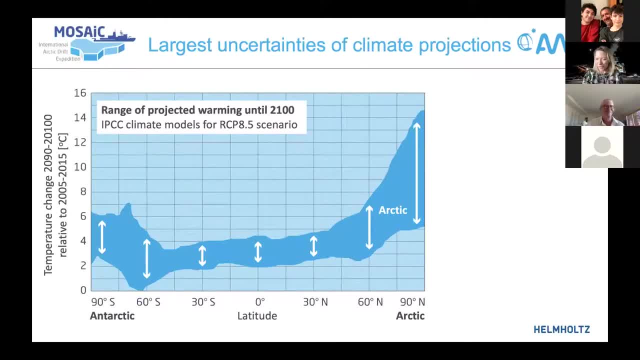 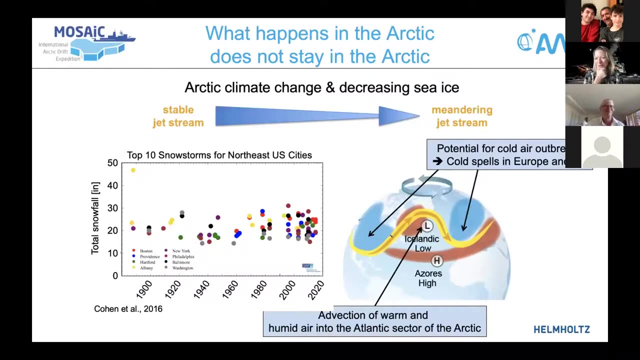 and that is still a mission for years to come- to bring all data together to be able to change also the algorithms with which we do the climate modeling. what i also wanted to discuss is the what is currently in the media a lot in germany because we had this weird end of the winter where 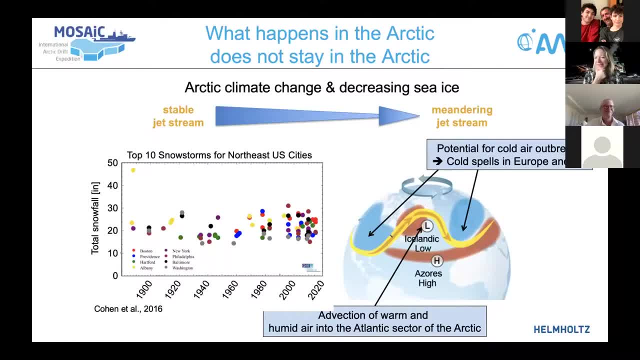 just a week ago i was ice skating at minus 20 degrees and now that i'm speaking to you, it is plus 17 degrees outside. so we have just in germany- and that happens now all around the world- in the northern continent we have these effects of very dramatic shifts in the stability of the jet stream, the polar. 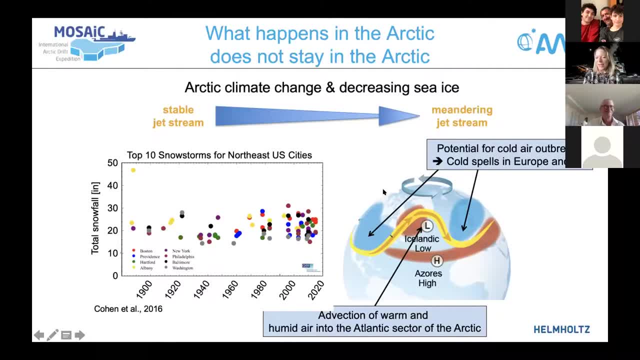 vortex and the jet stream. what does it actually mean? it means that- and that's the hypothesis that we are analyzing, also with those data- when we have sea ice present, the way we had for the past ten thousand years, we have a relatively stable polar vortex that you see here on this little depiction. 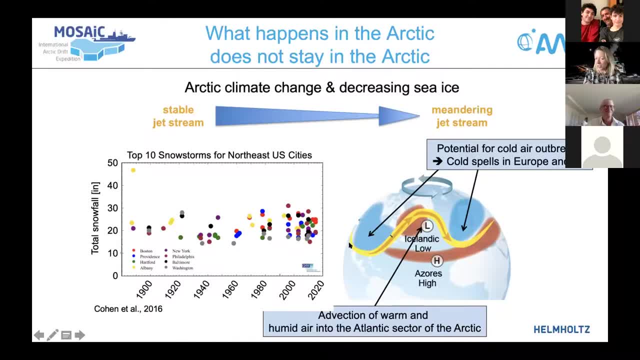 on the earth and then you have a relatively stable jet stream, and both are stabilized by temperature gradients and, of course, by many other physical factors. but once the temperature gradient decreases- and there is this idea that sea ice is part of that problem- shrinking sea ice, the jet stream, the polar vortex can get weaker. 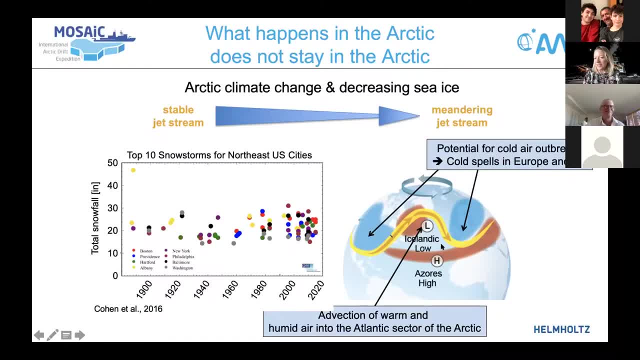 And that can lead to the meandering of the jet stream, causing situations as I've just described, that in one week you have this cold North Pole air coming down to the continents And in the next week you have the warm African air coming up to the continents. 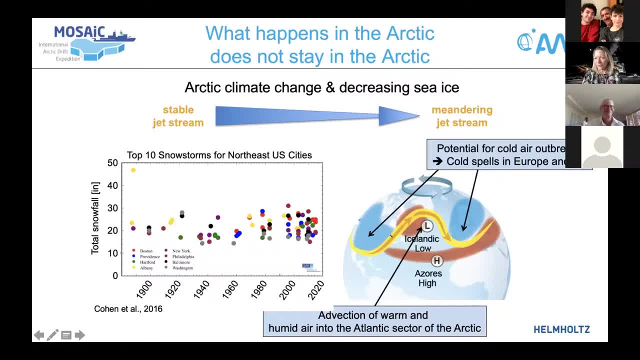 We just had amazing pictures this winter. I don't know if you saw the snow on Madrid. now the terror in Texas with the snowstorms, And so these risks that we have, they might well be connected to the Arctic amplification. It's still hard to prove that in evidence with the models we have, but there are so many factors that we have not well depicted yet. 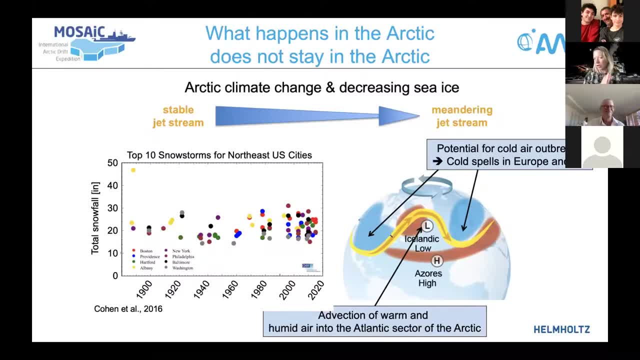 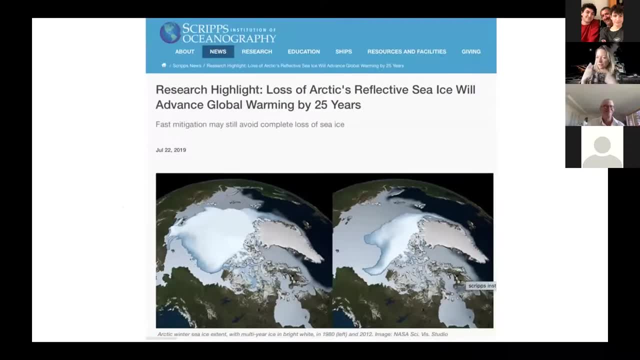 that we think that all of that knowledge, the value of putting all the knowledge together, is, of course, better prognosis for such situations. There is also the self-perpetuation, the reinforcing feedback loops that I've mentioned. For example, there is research out there that says the loss of the Arctic's reflective sea ice will advance global warming. 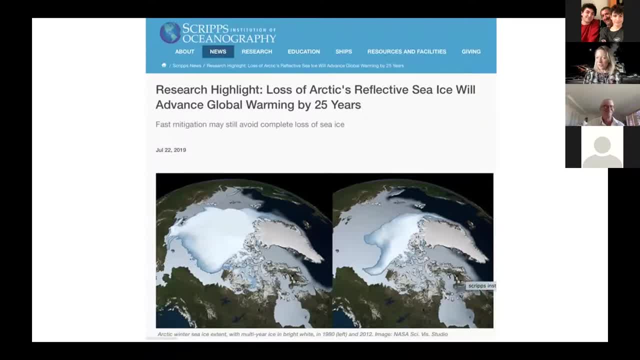 by much more And we have considered that we are considering today, when we are having this prognosis of warming in our regions and many more. I can- I don't have enough time- to list you all of those feedback loops that we think that are out there and that are connected to our lives. 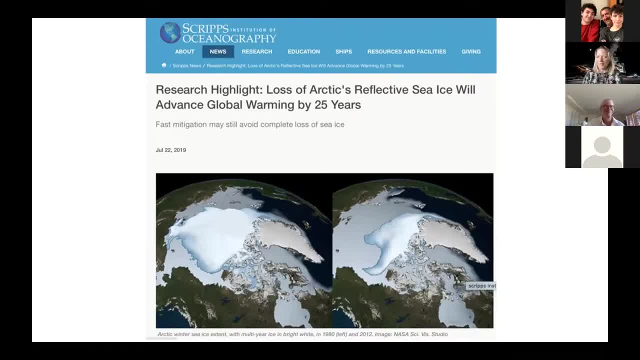 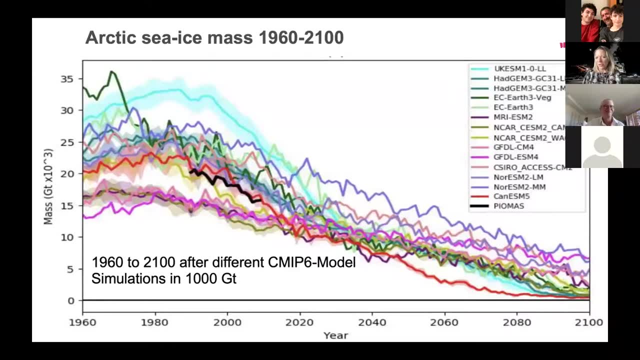 Note that, for those reasons, sea ice- Arctic sea ice- is considered a tipping point in the Earth's system. Now I'll end with this outlook of how. how will sea ice develop Exactly? that is one worrying point. That's the current six models that we have. the simulations that you have here for the ice mass are strikingly different. 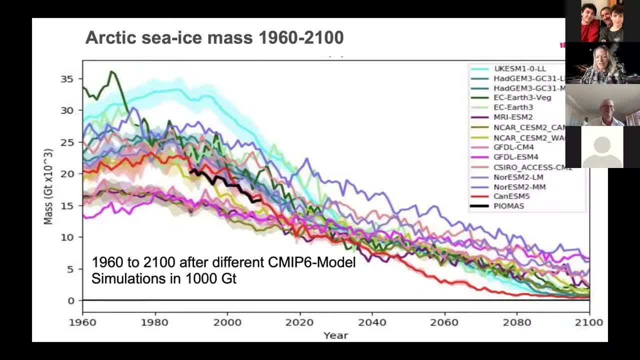 So some of the models predict currently that there could be ice-free summers as soon as the 2050s. We have new models even that predict the first ice-free summer could be there in 2030.. Some say no, it will never be ice-free. 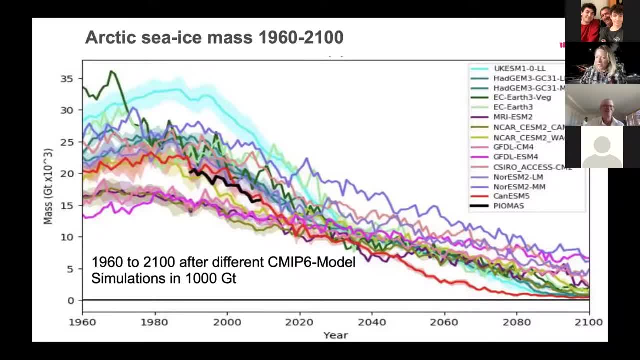 Some say no, it will never be ice-free. So this uncertainty means a lot to life in the Arctic, but also to people living in the Arctic, to businesses in the Arctic and all of that. That's really our big goal: that we will be much better in predicting the physical world. 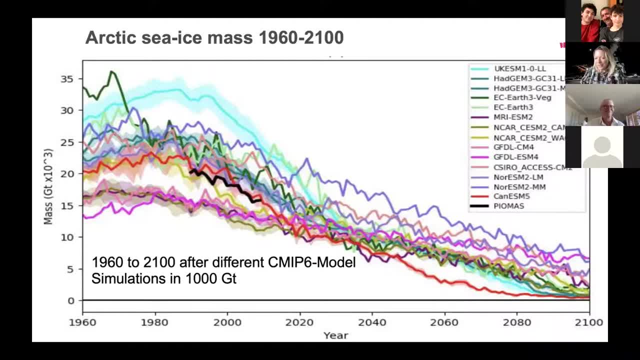 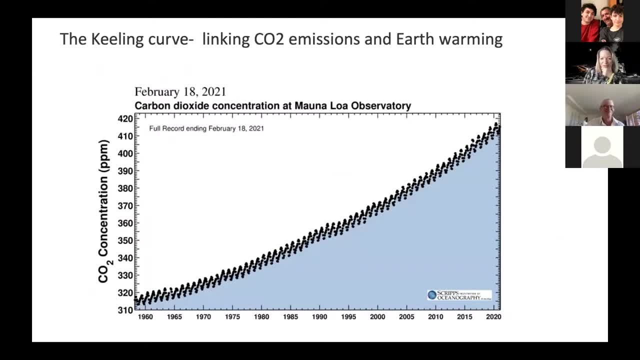 And hence we will probably also better understand the biological world and also us. But- and that's what I'm going to end with- Despite all the knowledge that we have connected for both polar regions that we can connect, And despite all that we know already how to do it, 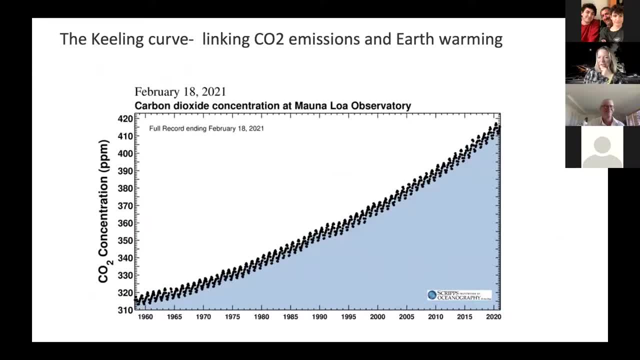 Despite all that, we know already how rapid the planet is changing. We see that CO2 concentrations in the atmosphere are ever increasing and mostly due to continuous human emissions, human uses of fossil fuels. So some people have expected that we can see the effect of the corona pandemics on the CO2 concentration in the atmosphere. 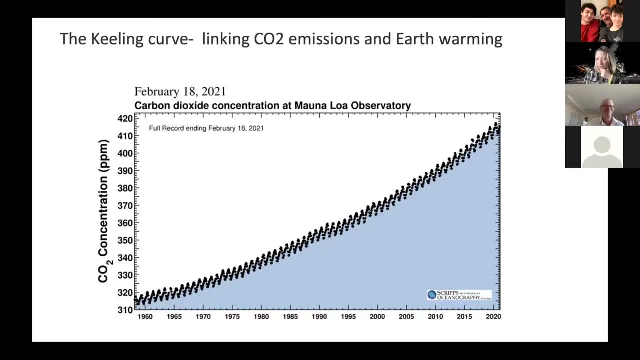 But we can see it in total emissions, total global emissions. They have dropped by 7% or so, but we are not seeing that yet in the atmosphere And that's not only because of the global warming. We are also seeing it in global warming, also from the natural warming. 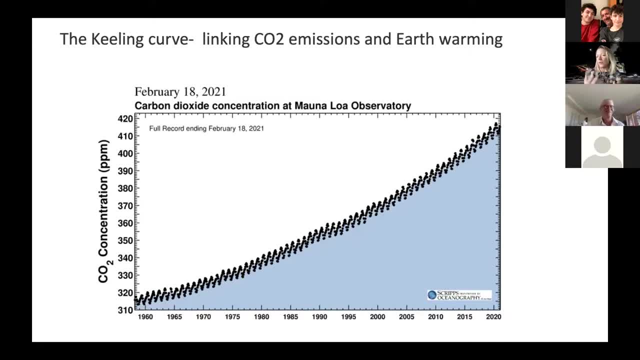 For questions of slow mixing rates, but also because there are so many processes out there in nature where warming of us means there will be an enhance CO2 emission, also from nature itself, From forests, from all kinds of processes, and that's worrying news. 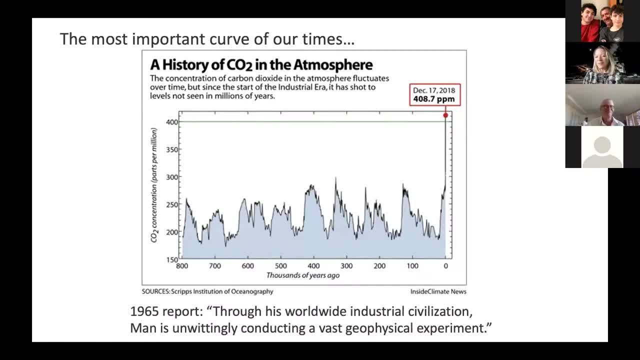 Note that when this picture was drawn in 2018, where humanity crossed for the first time in wintertime, 400 million lives were lost: 409 410 parts per million, so really a range that has not been present on earth since the. 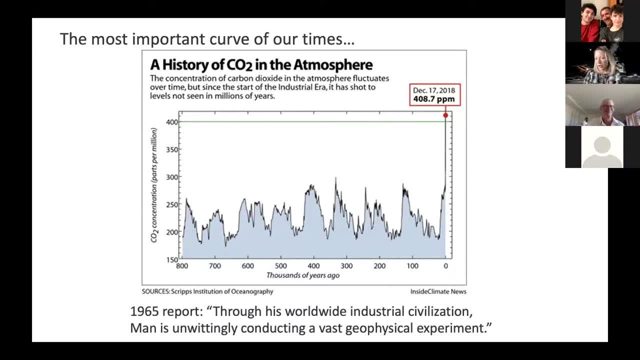 holocene we have now crossed 415 parts per million and this is once again a reminder that, knowing our history, we are completely outside of the range of nearby geological processes. geological knowledge we have on earth, as you can see here on this graph that takes you back 800 000 years. in that time you see earth's natural variation with co2 in the atmosphere. 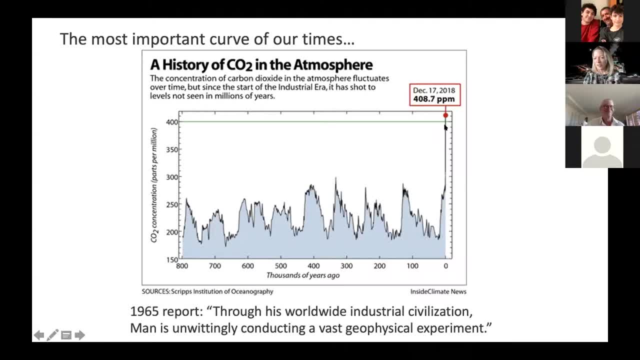 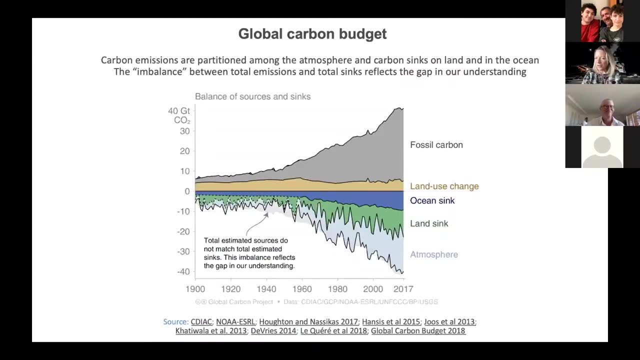 that have to do with angles to the sun and so on. but you see that us humans have completely changed the way that that we live today. the climate warming that we see today, it is not natural by whatever means. so the big question is: what does it mean for the cryosphere? i like this graph and 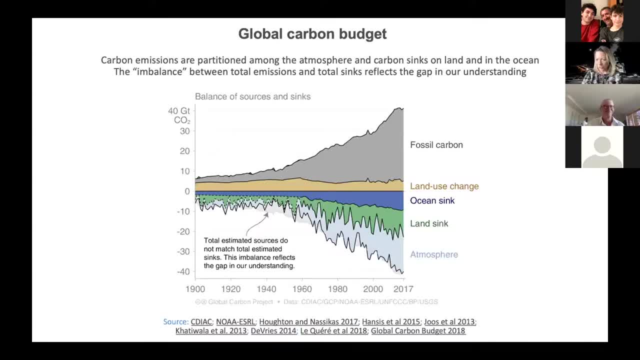 this investigation of the global carbon budget and the future of co2 in the atmosphere, and it is directly connected to that future of the cryosphere, both in arctic and in arctica. what you see here is along a timeline of our human behavior. basically, you see here above: 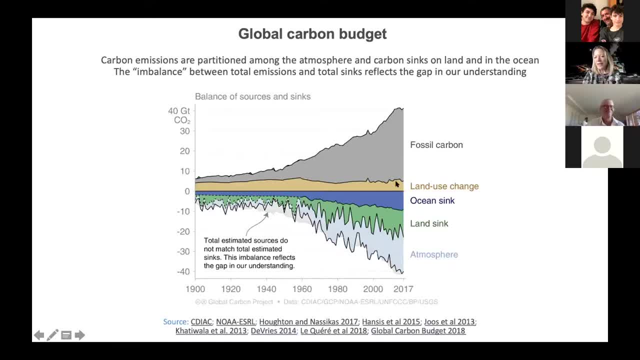 the zero line in yellow and and gray, land use change and fossil carbon usage, and you can see that we have much increased in the past years the emissions from fossil carbon uses more than from land use change, and you have to understand that nature is of course helping us in some ways to. 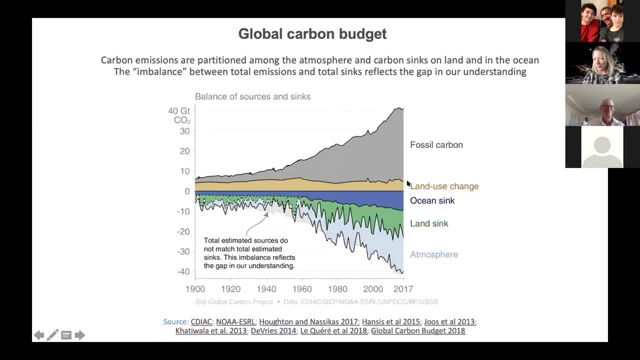 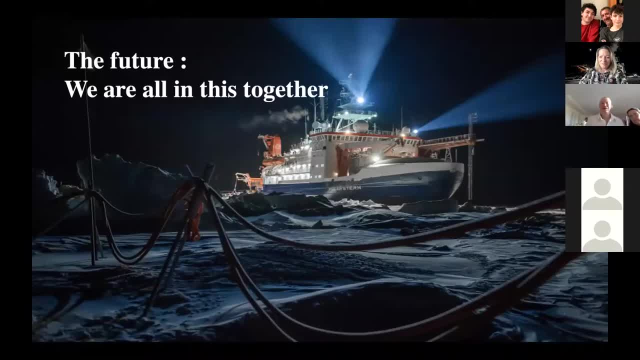 we have to understand that nature is, of course, helping us in some ways to change the way that we live today. We have to understand that nature is, of course, helping us in some ways to change the way that we live today. Thank you so much, Anshar. That was really inspiring. 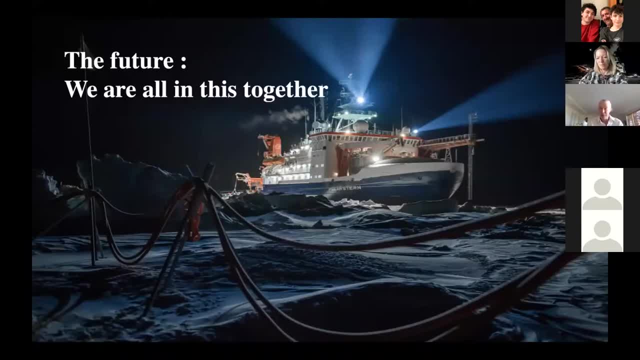 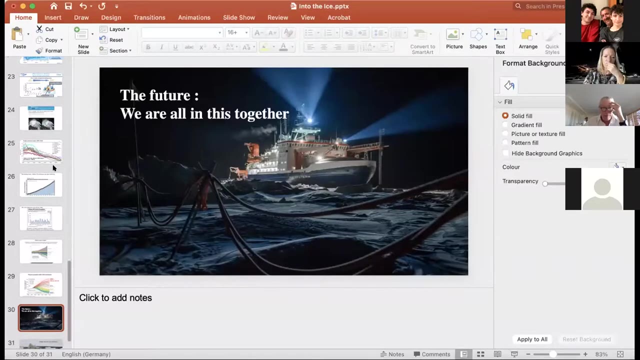 So there are a couple of questions. So there are a couple of questions, So let me focus on the latest ones. So the one question is an intriguing one. So the one question is an intriguing one, one from what you've learned. but, um, what do you have any insight about? what would be the impact? 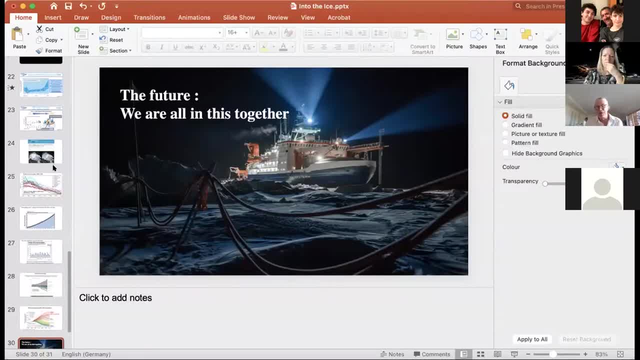 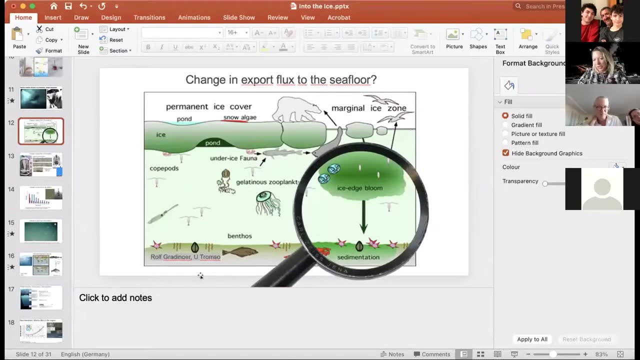 of um to the deep sea ecosystem in the arctic, presumably when there is, in fact, no sea ice available? yeah, that's a very good question. um, so the there are several publications out there that suggest that when sea ice shrinks, there will be even more sunlight, and that means more. 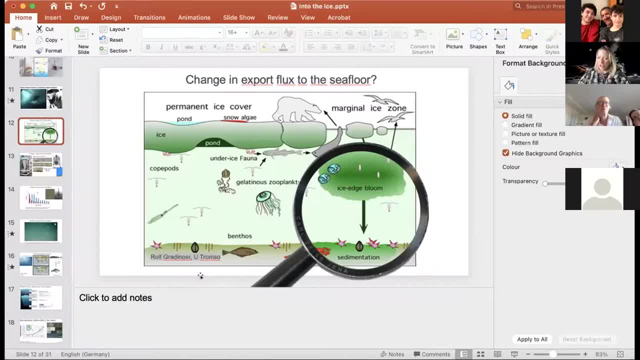 phytoplankton production. that means more energy, more nutrition to deep sea life. but there is a problem with this assumption and that is the stratification of the arctic ocean. so we know that in earth history the arctic ocean has become immensely stratified, almost a freshwater lake or 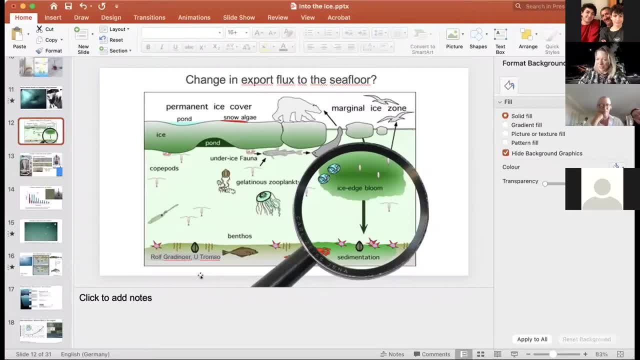 sometimes a full freshwater lake because it gets so much precipitation and and also river input and and that leads to a thin, less dense freshwater surface layer on top of the salty, warm Atlantic layer. And so once you have that stratification going on and we can. 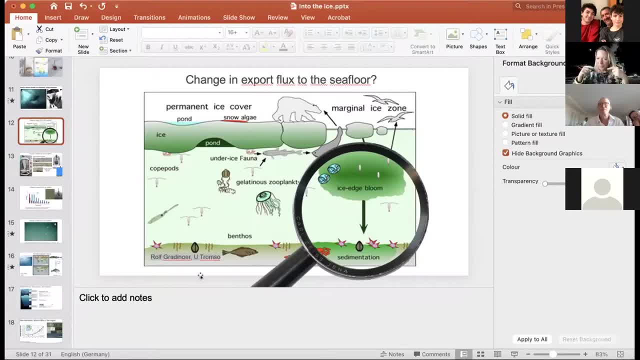 measure it already, there is almost no nutrient mixing. And so what we are waiting for- if eventually, the predicted increased waves and storms will kick in in the Arctic so that there would be nutrient mixing, because if you don't have mixing, if you have this very strict stratification, 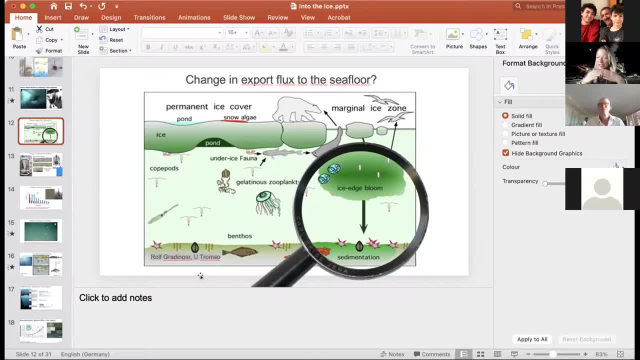 the idea that there will be more primal production is not realistic. So in some areas of the Arctic we see that effect already. we actually have so little nitrate as a nutrient in the Arctic that we can have only a tiny bit of phytoplankton production And the sea ice. when you think about 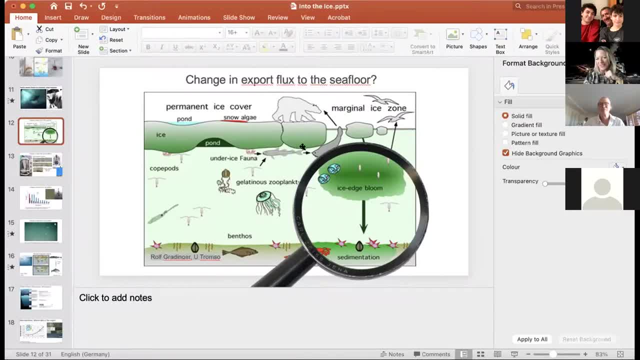 it for the phytoplankton mats that I've shown to you. the sea ice has sometimes a function like a transport means or like a bus. So the algae that get grow on the sea ice that get shuffled around by the wind, they will also get shuffled around by the wind. So the sea ice has a function like a always have access to more nutrients from that mixing of the sea ice, So they might be really critical in the nutrition of the life in the Arctic and deep sea, And that's exactly what we're researching. My prediction is that on the Arctic shelf areas there will be more food and more life. 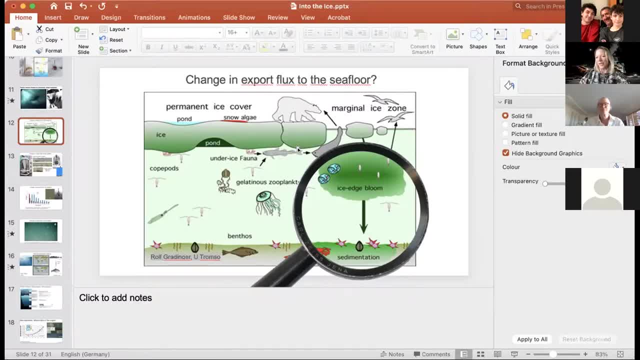 in the future, But that central basins will probably have a problem and having enough energy in the future- Fascinating. So there's another question which is a very contemporary one. Did you notice? did COVID, the lockdown, have an effect on the sea ice? the rate at which the 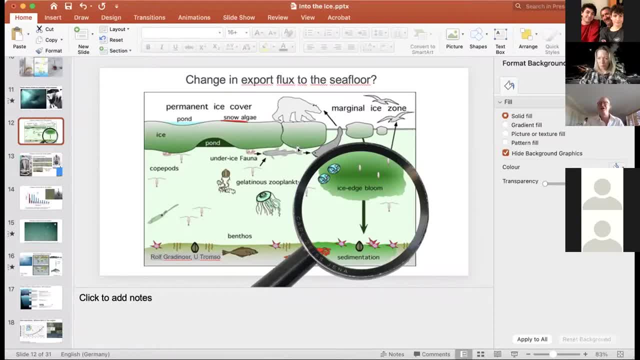 sea ice was melting. In other words, was there a direct effect between the reduction in emissions? No, the emission reductions were far too small to have an effect on the system as such. So the global carbon reduction: it's not fully calculated yet what the second and third waves that many countries saw what effect that had. But we are. we have probably saved us some seven or 8% of global emissions for a year now, And seven to 8% is just not enough to really change the climate system. as such, It is a contribution, So you could say. on the long run it matters also for sea ice extent. 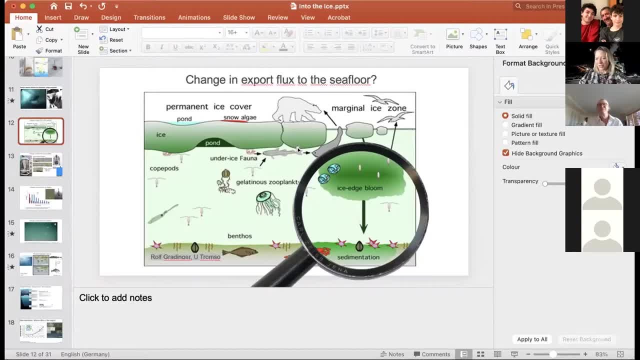 in the Arctic, But it is not an effect that we can have on the system as such, So I think that's what we can directly measure. In fact, we had the fastest sea ice melt ever last summer in the middle of the lockdown, because of the highly warmed atmosphere- the warm north, Don't know. if you read. 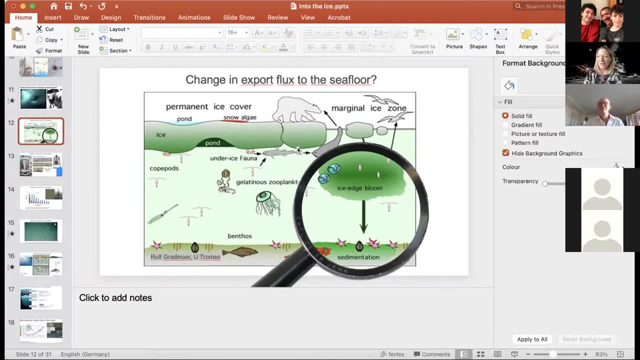 about this, but Siberia had heat waves where it became 30 degrees plus in Siberia. Okay. so one very last question. Okay, Because we're running out of time and I'm also cognizant of yours and Helene's time. 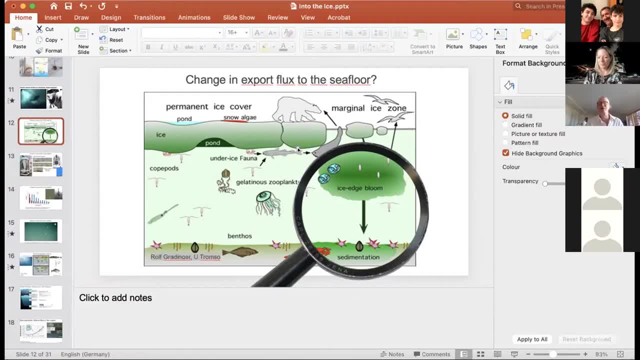 If we were to follow RCP- I mean SSP 1.1, how long would it take for the Arctic system to recover? That's an excellent question. So we have a big debate about this because when it is cold enough, so when we have a normal, when we have the ice, 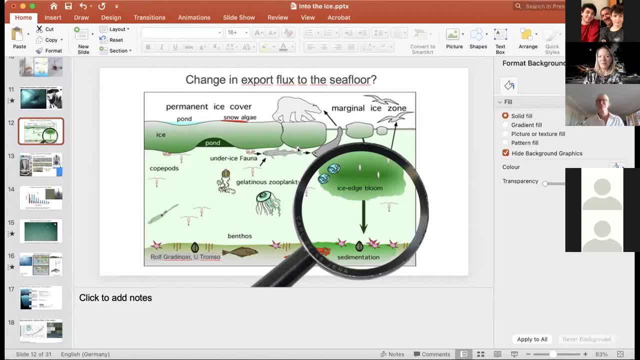 Okay, Okay, Okay Okay. winter, the polar night it can become very cold. So also during mosaic day observed minus 40, minus 42 degrees Celsius. And that's physics. So sea ice will build back when there is a cold. winter, when there's the next cold winter and the summers are not too warm. The prediction is that within 10 years we could have 10 to 20 years. we could have thick, multi-year ice back, But for that to have cold summers we need a completely different planet or a different progression. 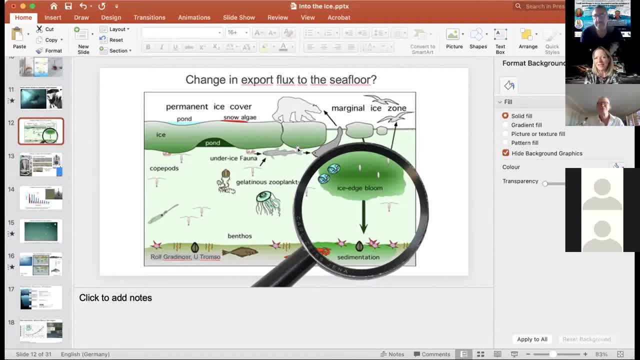 So the sea ice physicists that I asked the same question as biologists. they told me it probably needs some mitigation. There are crazy ideas like, for example, pumping ocean water onto the ice flows, that they are better protected in the future, or other things like that It could. 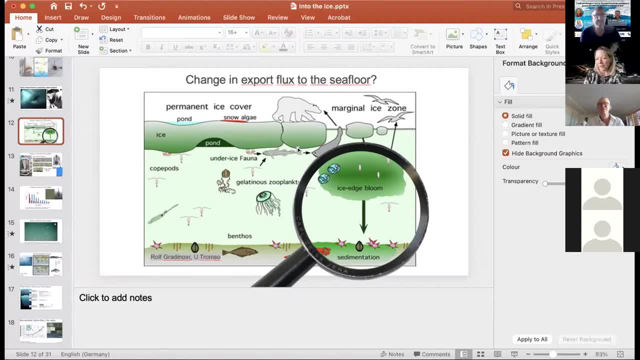 need a couple of decades if we would be really coming, managing a generalization of the sea ice as the plus 1.5 degree average warming. it still could take decades for the system to fall back into what we know, what we knew as PhD students, But that's all very unlikely to happen. So 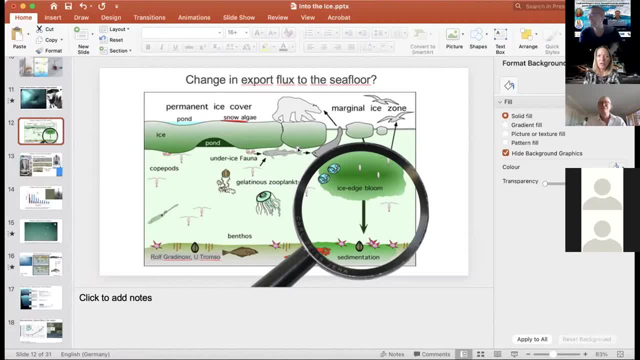 most sea ice. physicists say that our generation will see the first summerly ice-free Arctic. Well, on that, I'd like to thank you both very much for really both- both really inspiring presentations. They come at a good time for us, you know.